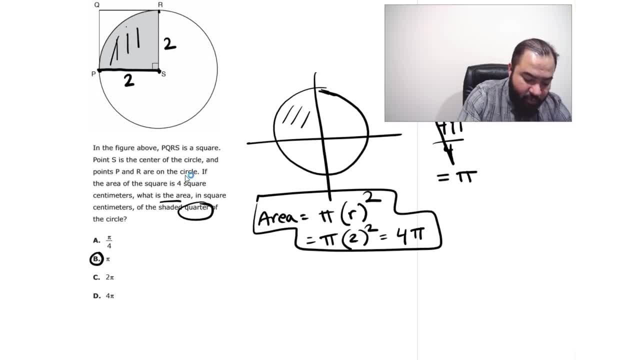 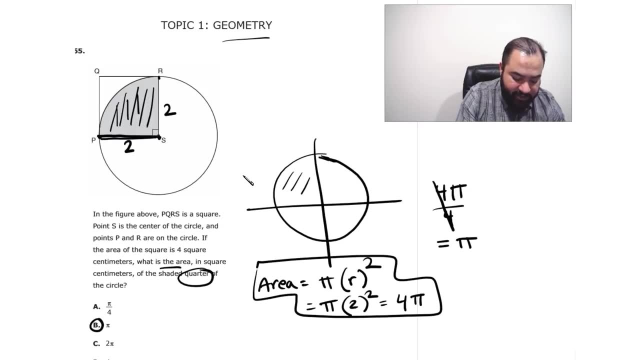 What we're learning here. So we have to just find one-fourth of the circle, not the full circle, Just one-fourth of it. So we did find the radius, which is 2, and we used the formula pi r squared and that gave you the answer. 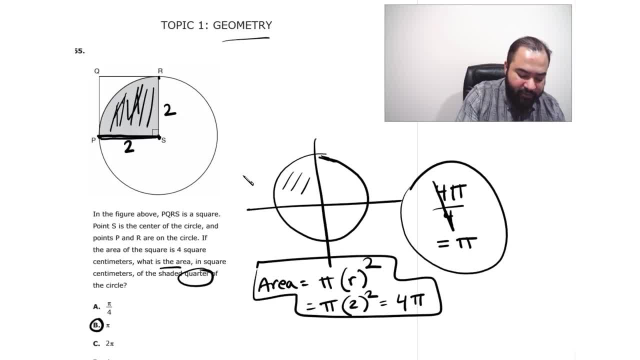 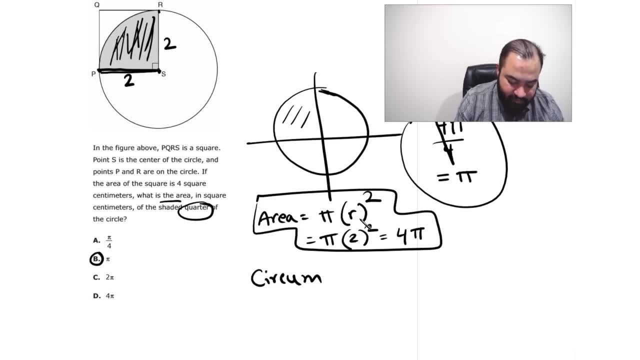 But we have to divide it by 4, because we want only the one-fourth of the circle. Now, remember, you have to also know the circumference formula for the circle for the test. Circumference is what guys Pi times the diameter. 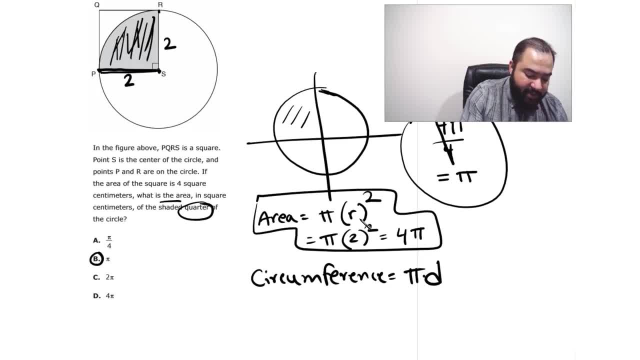 Pi times the diameter, Pi times the diameter. So if the radius is 2,, the diameter must have been 4.. If I were to find the circumference, which is the length of the skin- we can also call it r- I would do pi times the diameter, which is 4,, 4 pi. 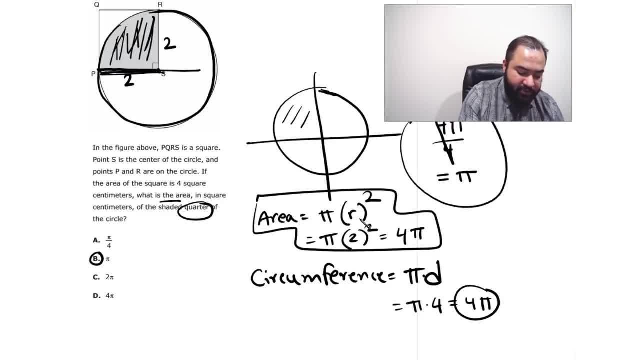 The diameter is 4 because radius is 2, diameter must have been double, so which is 4 pi. So these are the two formulas. These are the two formulas you must know for the test, for the circle area and circumference. 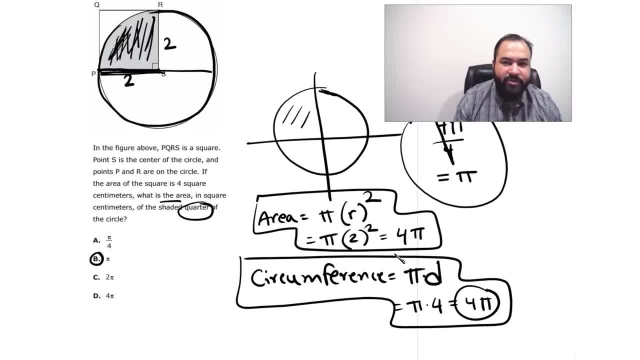 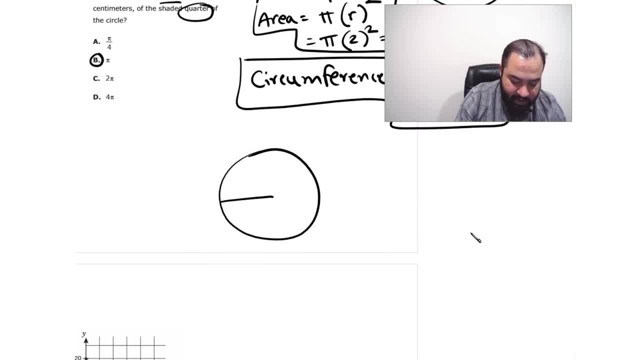 And also this is called sector means part of the circle you're finding. So let's talk about it a little bit more. Let's say I give you a circle and I tell you to find the area of this half of the circle where this is the center right. 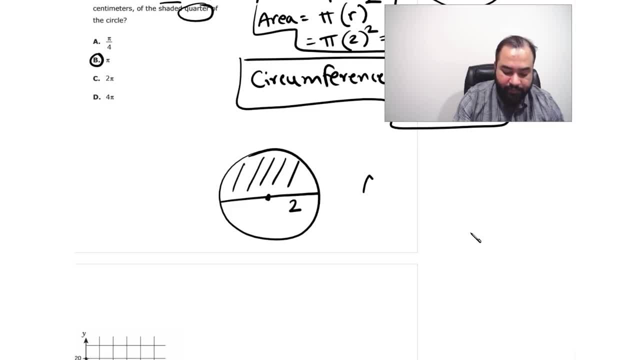 Half the circle and radius is 2.. What would you do? You know the area formula is pi times the radius, power 2. It's called square, So you'll do pi times 2, power 2. That's 4 pi right. 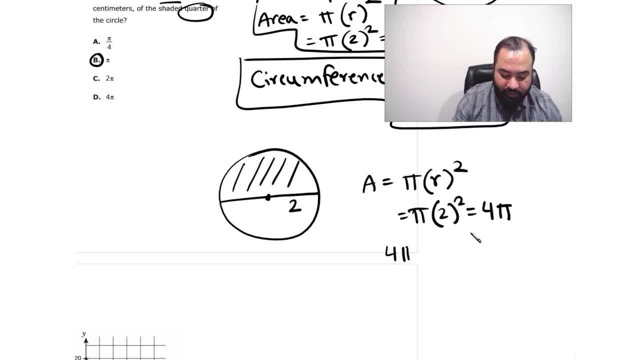 But we only want the half of the circle. So you do 4 pi divided by 2.. You're right. So you get 2 pi. So, similarly, the circumference works the same way. If I were to find the circumference, the half of the circle, I would use the formula pi times the diameter. 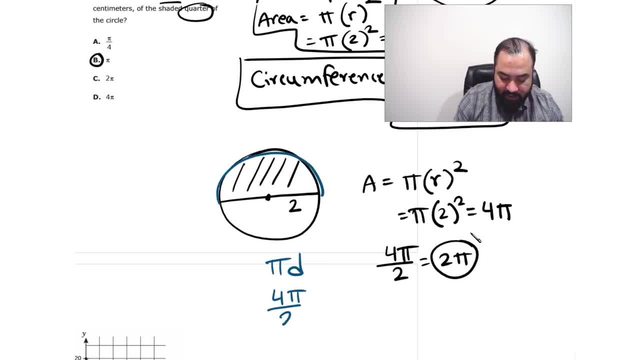 So diameter would be 4.. So it would be 4 pi divided by 2.. Because I want to know, I want to find only half the circumference, That's 2 pi. So you should understand that part All right. the next question, 78.. 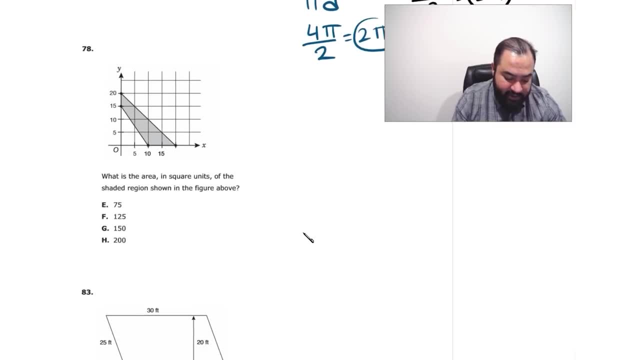 It's the shaded region again. So in this case they said: what is the area of the shaded region? Now, if you can see, the shaded region is kind of like a weird shape. It's not like a regular shape, It's not a parallelogram or something. 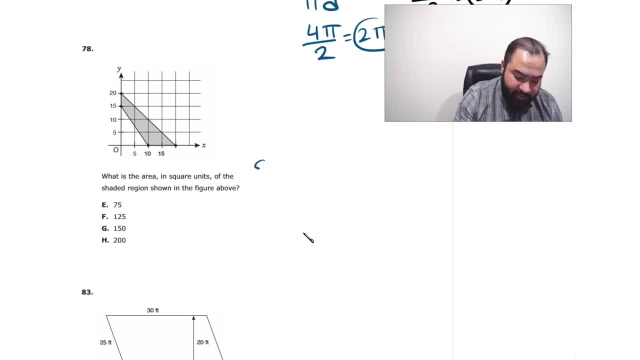 So we don't know what it is. So what we can do is we can use the formula that if I were to find the shaded, I would find the total minus unshaded. Now, if you were to see what I mean by total, 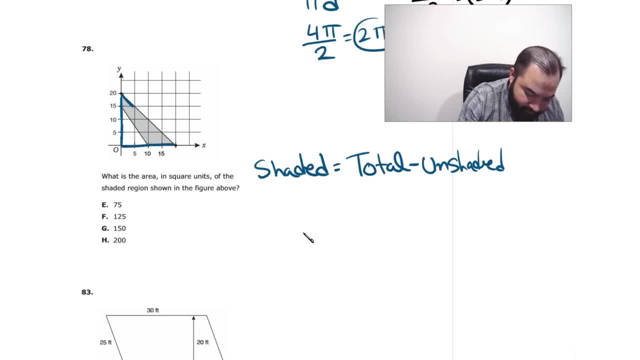 So I can target this triangle here, a big triangle, You see, the blue triangle. So from the blue triangle, if I were to just subtract out this baby right, triangle, right. If I just subtract this out, that leaves me with the shaded region, right. 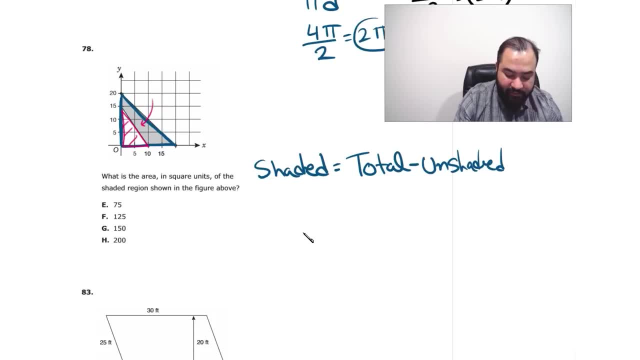 So what we can do is find the area of the big triangle. How do we find the area of a triangle? So remember that area of a triangle is half times base, times height, right. So here base is 5,, 10,, 15,, 20.. 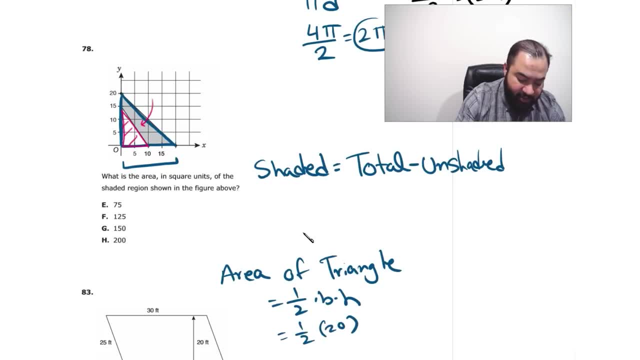 So half times 20 times the height is 20 as well 20.. I'm finding the area of the big blue triangle, That's 200, right. Now let's find the area of this small pink triangle, which is 10 by 15, right. 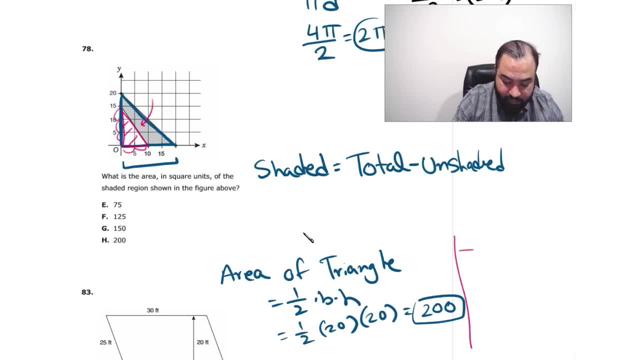 So we use the same formula. So half 10 times 15.. So that's 150 divided by 2 is 75.. Now how do we find the shaded region, guys? I know the area of the big blue triangle is 200.. 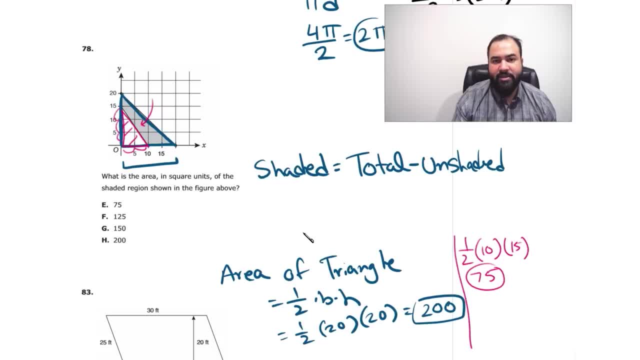 The area of the pink one is 75. So how do we find the shaded region? You're right, We just subtract So 200 minus the 75. That gives me 125, and that's the answer. Let's do the next question. 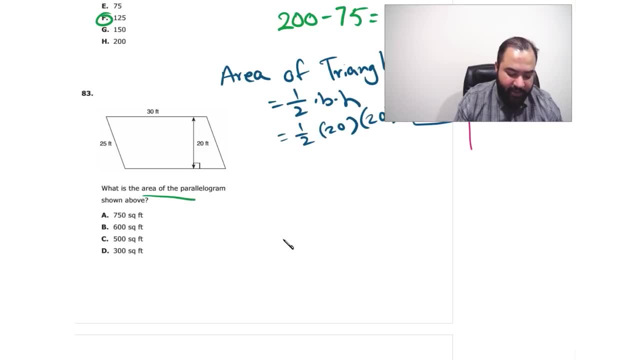 It says there is a parallelogram. They said: what is the area of the parallelogram? So we know the formula is: area of the parallelogram is equal to base times the height. That's it, just base times height. Now you have to recognize this base. here is similar: 30.. 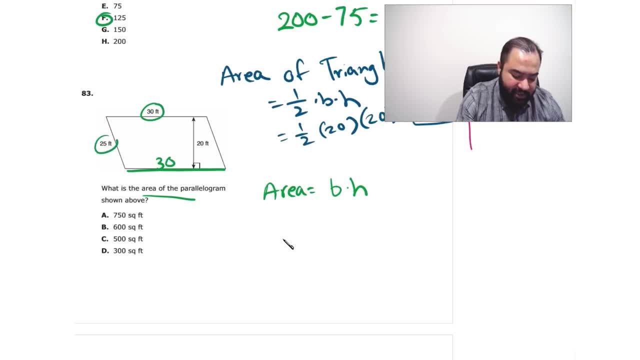 And the height is: which one is the height, guys? 25 or 20?? Now, the answer is 20.. Do you know why? Let me explain it. The reason is, you see, the 20 is making 90 degree with the base. 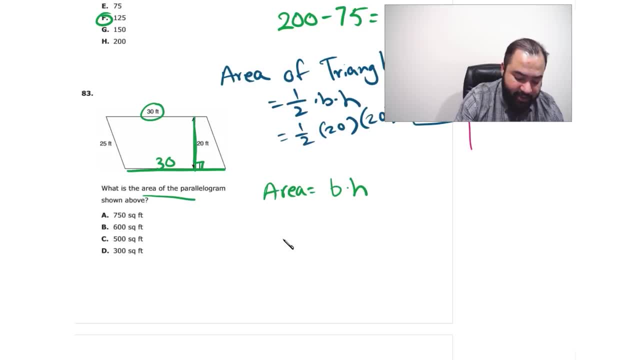 So the definition of height is: height has to make 90 degree with the base. But this 25 is not 90. It's more than 90. So that's not the height. The height has to make 90 degree with the base. 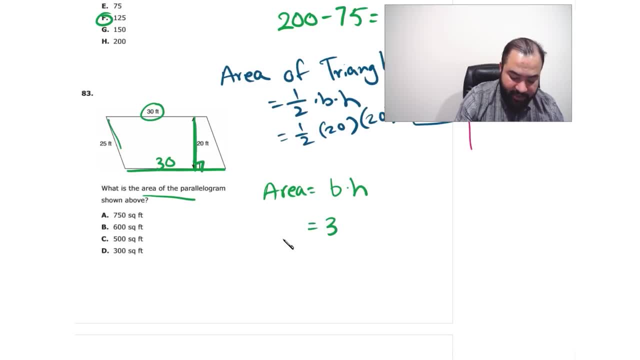 That's the definition of height. So we're going to take the base as 30, and the height is what guys? 20, because it is making 90 degree with the base, Remember this. So that's 600.. Okay, that's for parallelogram. 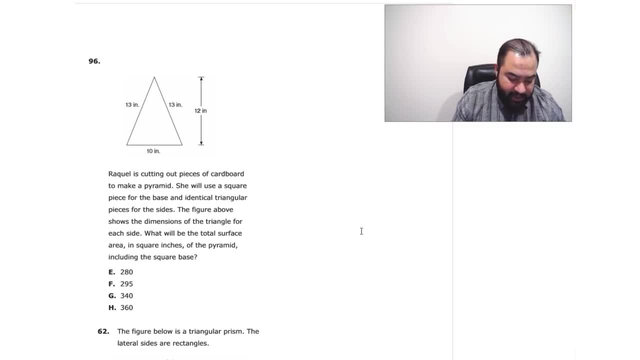 Now, here there is a triangle, as you can see. So now it says: Dracuil is cutting out pieces of cardboard to make a pyramid. She will use a square piece for the base. So she will use a square piece for the base and identical triangular pieces for the sides. 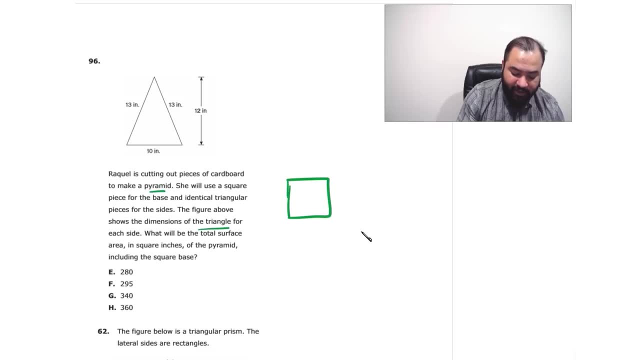 The figure above shows the dimensions of the triangle for each side. So these are the triangles. So she will use the pyramid. takes four triangles, So four identical triangles to make the pyramid. So one square and four triangles. Now what will be the total surface area? 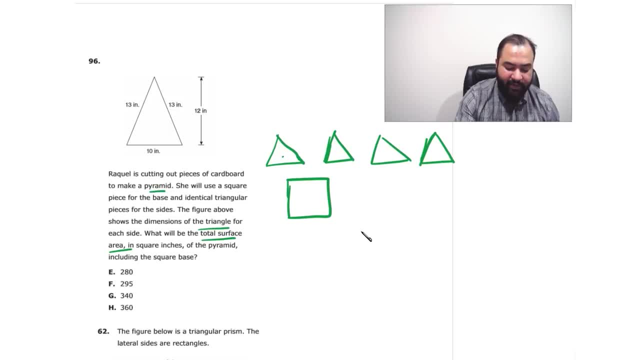 If you want to find the surface area, you can just find the area of each shape, all five of these and add them And that will give you the surface area. So first of all, the triangle, the shape is, the base is 10.. 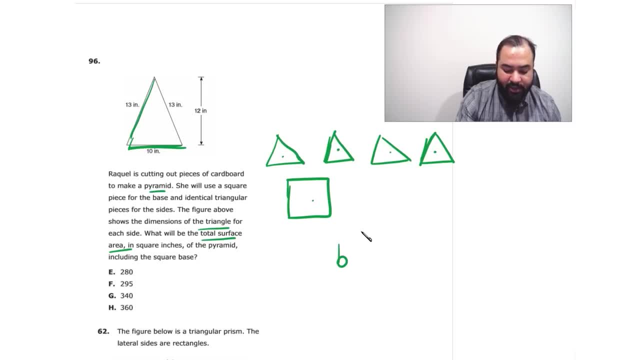 You remember the formula How to find the area of a triangle. Yes, base times height divided by 2, right Or half base times height, same thing. So base is 10.. What is the height, guys? Is 13 the height or 12?? 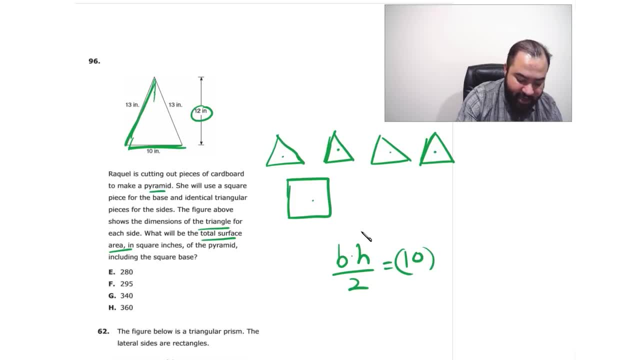 You remember the definition of the height: Height has to make 90 degree with the base. So the 13 doesn't make 90, but the 12 does. This 12 is here. if I put it, It's the same thing. 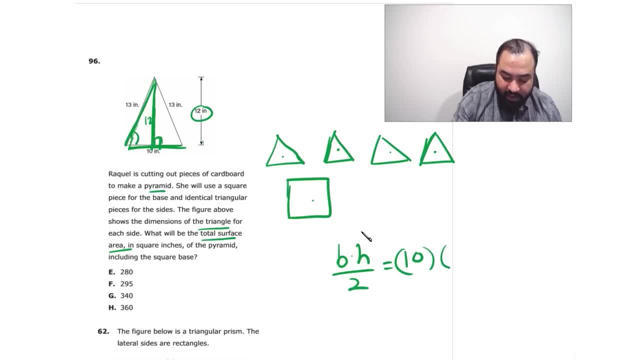 So 12 does make 90 degree with the base. So I'm going to take 12 as the height and divide it by 2, of course. So that's 120 divided by 2. It's 60. So 60 is the area of one of the triangles, and there are four of them, four identical. 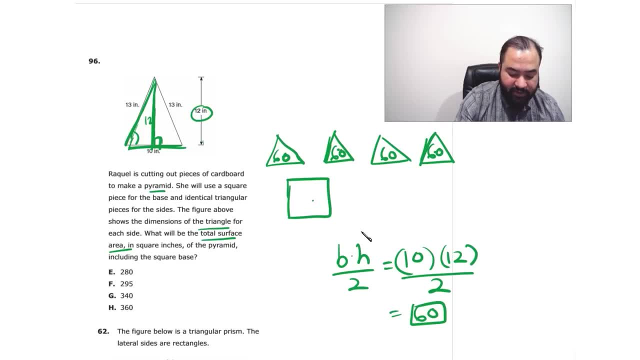 You know, a pyramid takes four triangles. So 4 times 60 is 240.. That's the area of the four triangles. Is 240? the answer No, because you have to add the area of the square. Now, what is the dimension of the square? 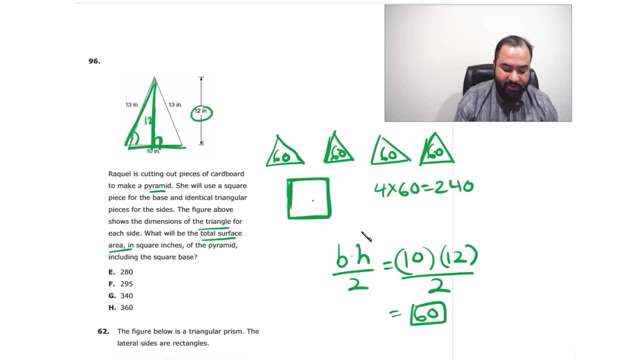 You know how to find the area of the square: the length times width, or the side squared. So the dimension of the square will be: each side is 10.. You'll be like why? Now let me show you. If I were to make the pyramid, I would make it something like this: 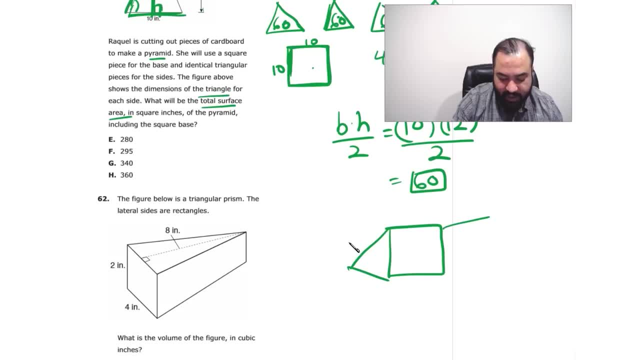 The square, Then I would have to put a triangle on this side. Sorry, Another triangle on this side, Another on this side, Another on this side, And then all these four vertices. I'm going to just put it together And then it will turn into a pyramid. 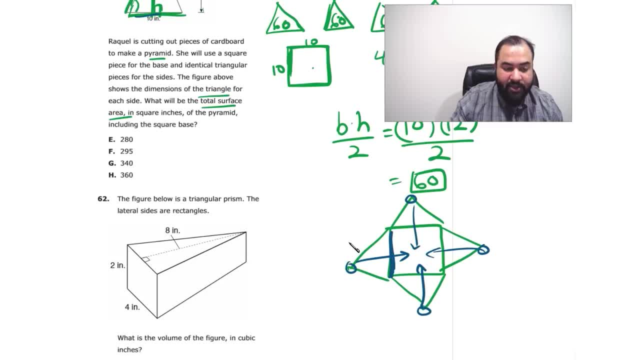 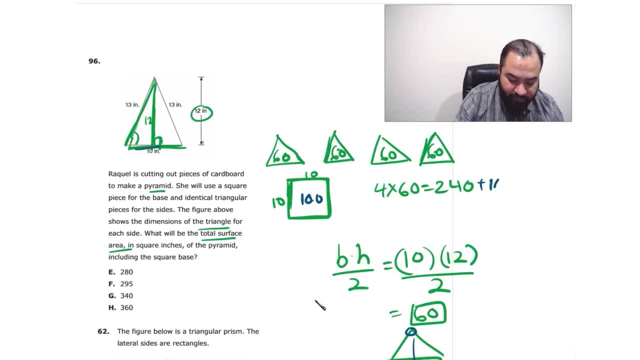 So, as you can see, the base of the triangle is actually the side length of the square, So the area of the square will be 100.. And now you add it with 240. So that's 340.. Okay, So if you want to find the surface area, find the area of each shape, just add them. 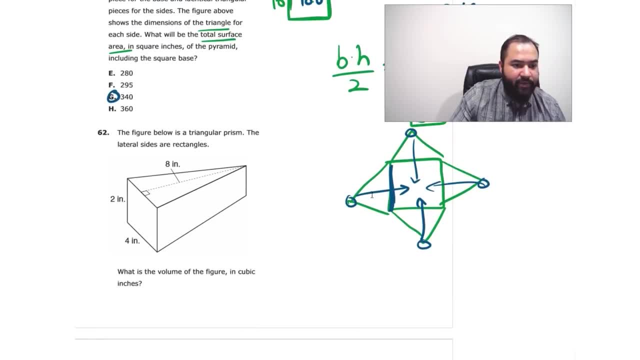 These questions are very important. They come on your test, So I'm giving you a brief explanation so you guys can study it before the test and get some help. All right, Number 62. The figure below is a triangular prism, guys. 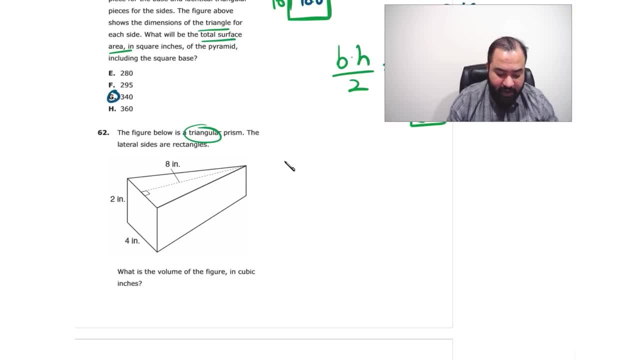 Remember this Triangular prism. Now You want to find volume, because that's what they're asking for. What is the volume of this shape? This looks like a piece of cake. So if you were to find the volume of, let's say, a rectangular prism right which has a length, width and a height, 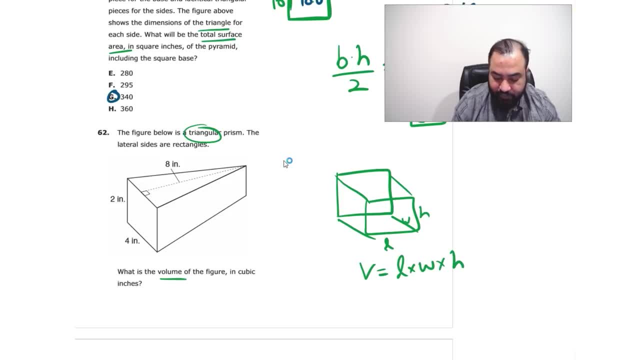 If you were to find the volume, you would do length times, width times, height, Right. So if it were to be a cylinder, how would you find the volume of a cylinder? If it were a cylinder, it has a radius and a height. 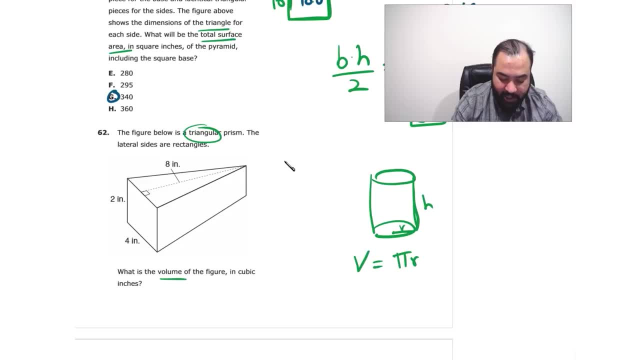 So if you were to find the volume of a cylinder, it would be pi? r squared times width by height. So that's how you find it. Notice what am I doing in each cases. So we find the area of the base, which is a circle. 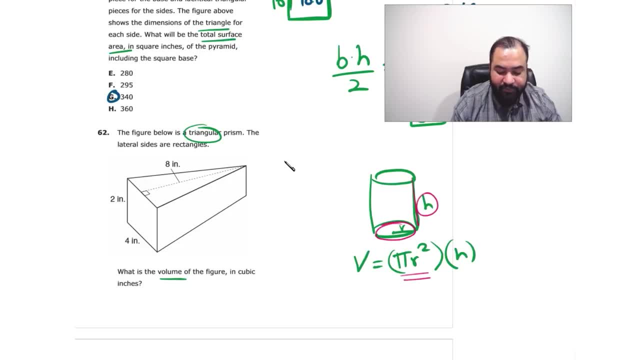 That's pi? r squared And we times it by height. That's how we find the volume of the shapes. We find area of the base, times it by height. So now I'm going to do this shape. This is a shape, It's a triangular prism. 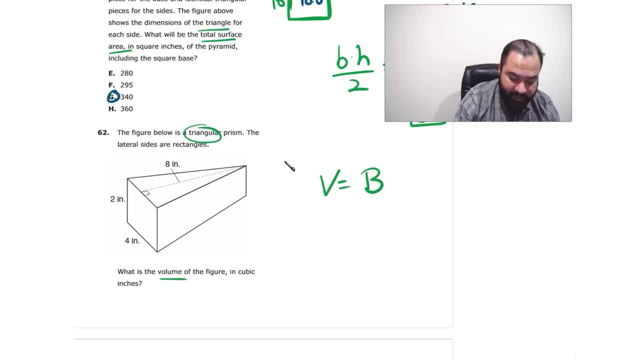 So first, if I were to find the volume, I have to find the area of the base. So the capital B stands for area of the base. If you see, before I used lowercase b for just the base, But the capital B is not just the base. 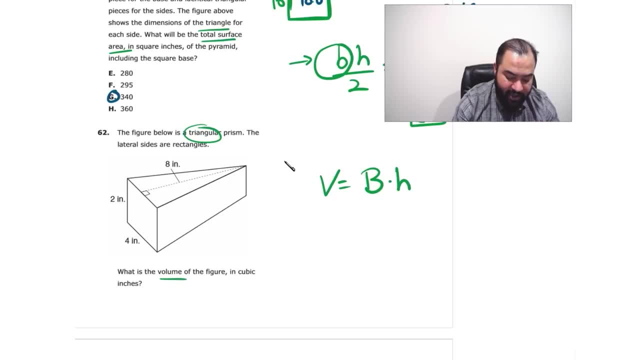 It's the area of the base. times it by height. Now let's take a look at it. What is the base of this shape? You can see there are five shapes in this, like three rectangles right and two triangles. Three rectangles and two triangles. 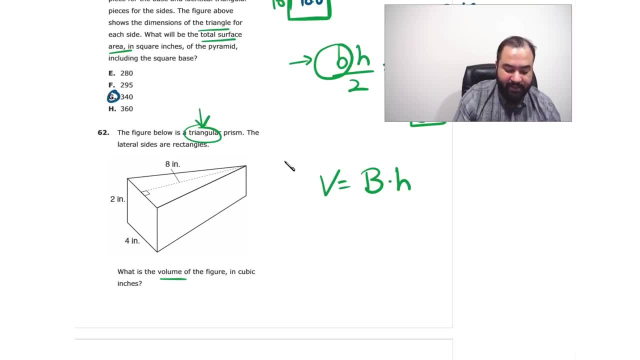 So since they named it triangular prism, so the base has to be triangles. So how do I recognize the base? It's going to be named right there. So area of this triangle is: we know that the base times the height is eight. 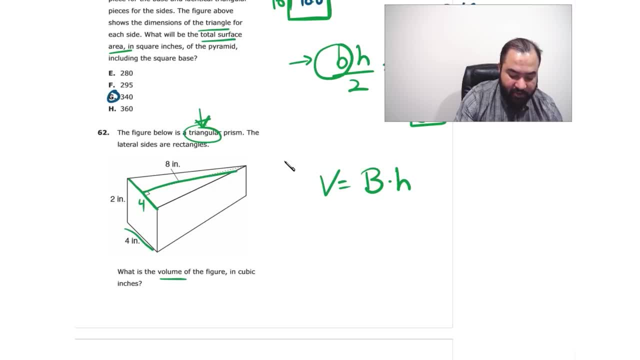 And the base is four. As you can see, this is four. So if you want to find the area of the base, so the B, let's use a different color. So capital B is equal to eight times Four divided by two. 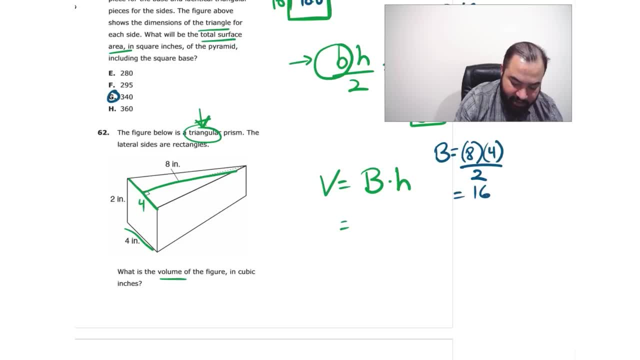 So that's sixteen. So we got it. that area of the base is sixteen. Now, what is the height? Now, that's the question. What is the height here, guys? Is the height? height is eight, Two Like. what height is this? 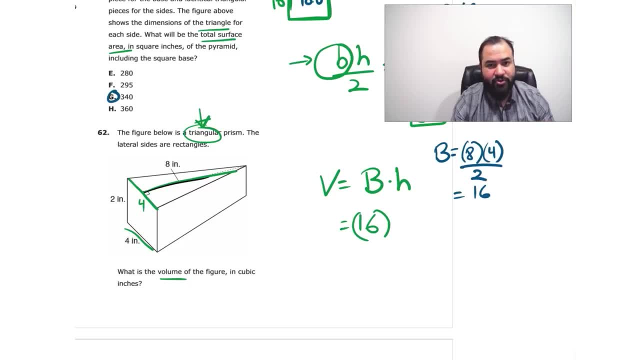 This is the height of the full shape. Now, as I said, the height has to make ninety degree with the base. If you can see this, sorry, This line two, that's making ninety degree with the base triangle. You see the line here that makes ninety degree with the triangle. 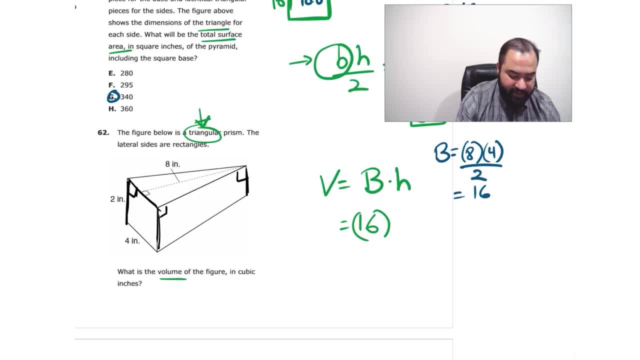 It's like perpendicular, If you can think of this as a roof, like a ceiling, And these are the pillars. So these are the actual height of the full shape, The height eight, that was just the height of the triangle, the base. 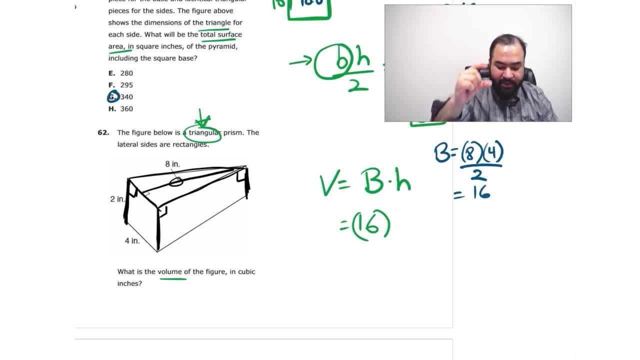 The two is the height of the full shape, like how thick it is. That's the height. So we're going to use two as the height, So sixteen times two And that is the volume. So area of the base times it by the height. 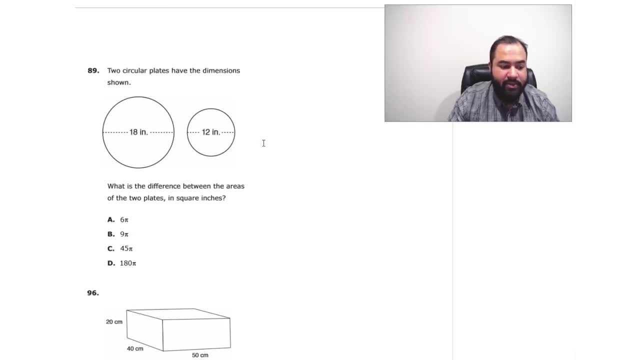 Be careful with the height, Like how you recognize the height is important. Alright, then we have circle, They said. what is the difference between the areas of the two circles? You already know how to find area of a circle: Pi times R square. 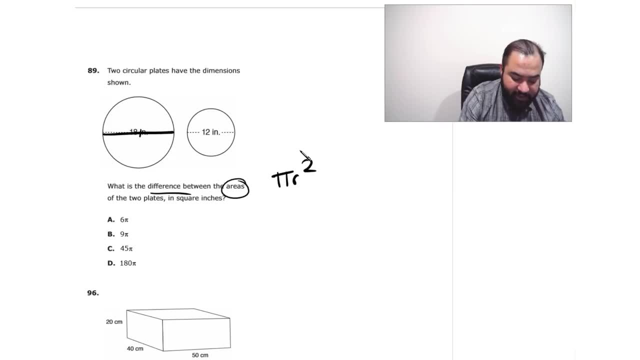 So if diameter is eighteen guys, what is the radius? Nine? So what must have been the area? Pi times nine power two, That's what Eighty one pi. How do you find the area of this baby circle? The radius is six. 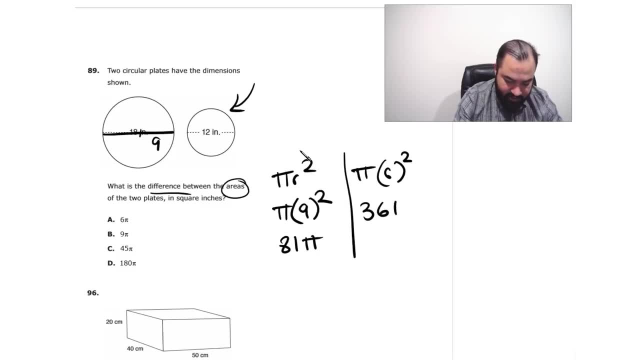 So pi times six square, So that's thirty six pi. And they said: what is the difference? Difference means subtraction, So you do eighty one pi minus thirty six pi. I believe that's forty five pi, And that's it Simple. 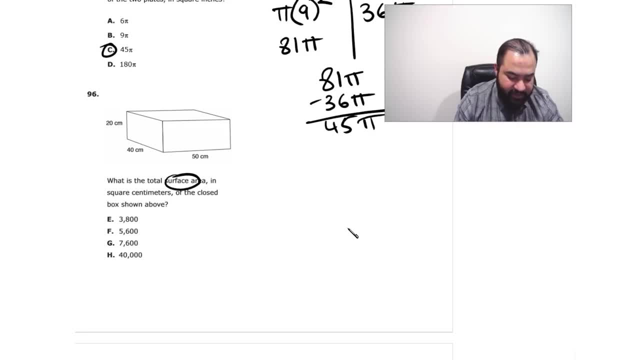 Now here, rectangular prism. They said: what is the total surface area? If you want to find the surface area of the rectangular prism, it's very easy. You could also find the area of each shape and add it, As I said for the surface area. 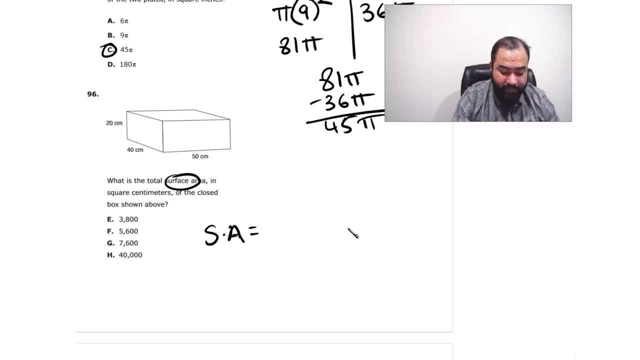 But rectangular prism. there is actually a way to find it Simple. You can just do two times. started parenthesis Right, Two times because there are two of each shape. So you see the three numbers: twenty forty and fifty. So I'll just write: twenty times fifty. let's say: 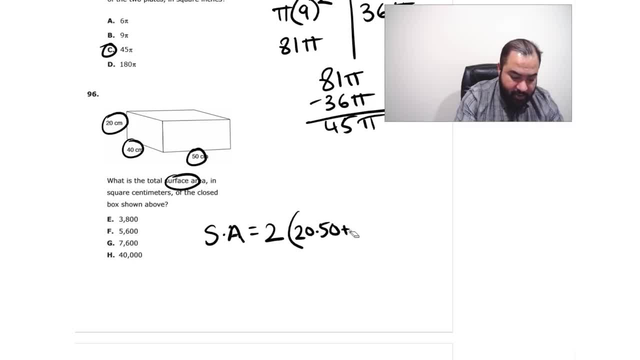 Plus Plus. you write Twenty times forty Plus. So I did twenty this times this And I did this times this. What remains This times this? So forty times fifty, And that will give you the answer. So you can see, I just switch around the three numbers. 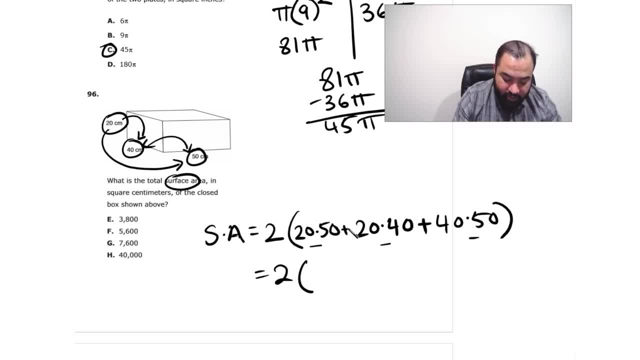 I multiply two times, So I get two times that's a thousand Plus eight hundred Plus that's two thousand Three thousand eight hundred times hit by Two. Seven hundred Seventy six hundred. That's your answer. Alright, That's the surface area. 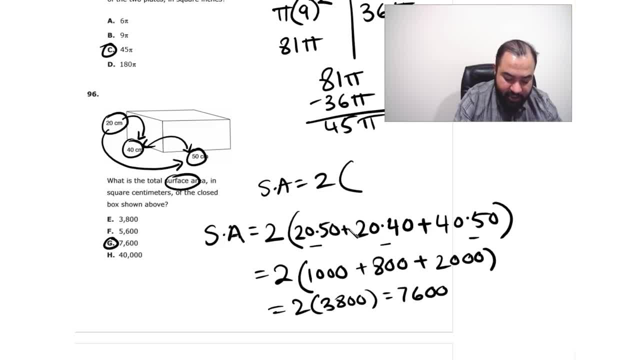 So technically, what I'm doing is, for surface area, Two times the length, times the width Plus width, times the height Plus height, times the length. Like you switch them around And you multiply. That's very simple. So now we have two triangles. 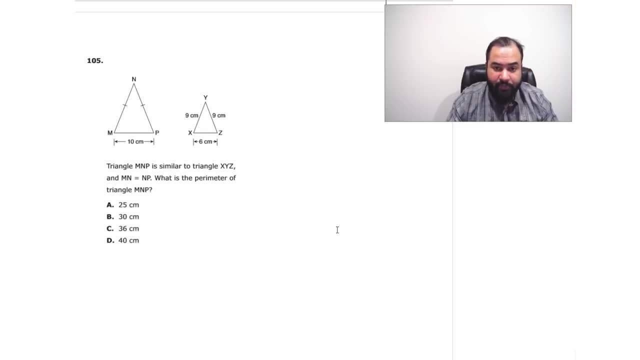 The triangle M and P And X, Y, Z, Right. They're similar. The word similar means proportional, Proportional Right, So we can set up a proportion between two triangles, You're like. what do you mean by that? 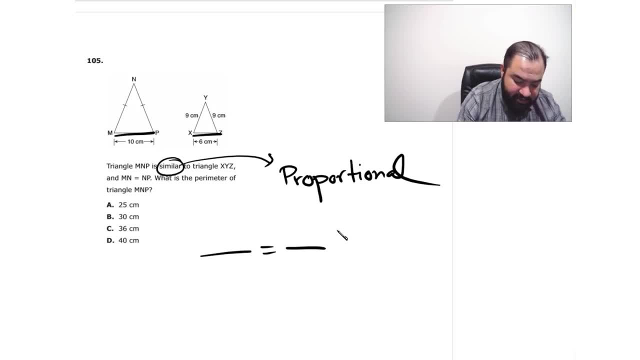 So I know, this side is ten, This is six. So let's put ten over six. And I don't know what this side is. Let's say X And this is nine. I can put X over nine, Right, Set up a simple proportion. 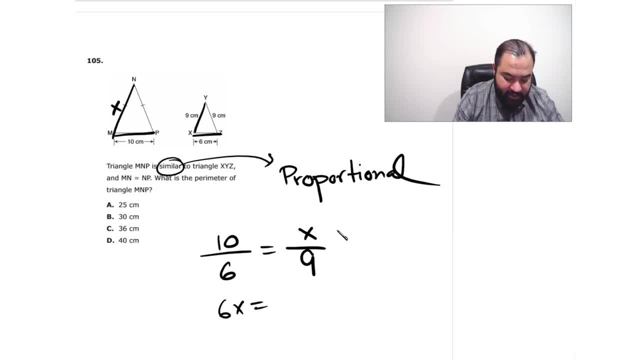 So now cross, multiply, So I get six X equal to ninety, And divide both sides by six, Six X equal to one By fifteen. So that's this side Fifteen. So as you can see, these two sides are equal. 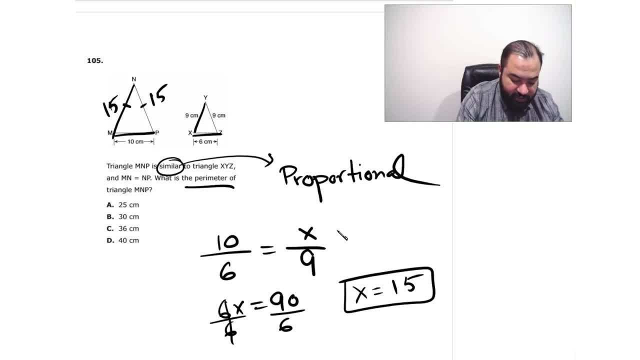 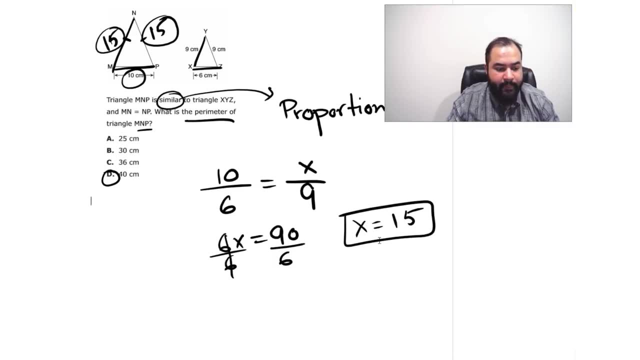 They marked it like this: So this is also fifteen. Now they say: what is the perimeter of the triangle M and P? So that's fifteen plus fifteen, Thirty Plus a ten, That's forty. Alright, That was it for the geometry. 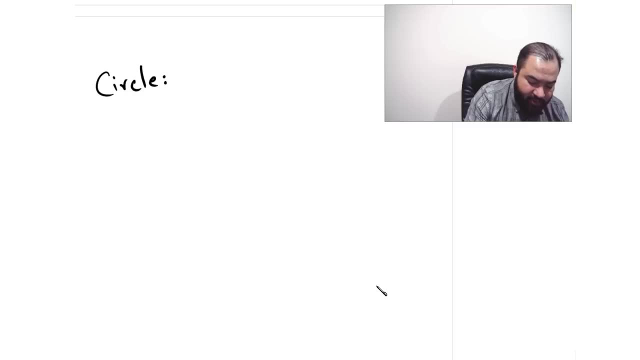 So, as you can see the things you have learned. So the circle You know, The diameter for the area Circumference is pi times the diameter. Parallelogram Area is equal to the base times height. Right, And one more thing you should know is the trapezoid. 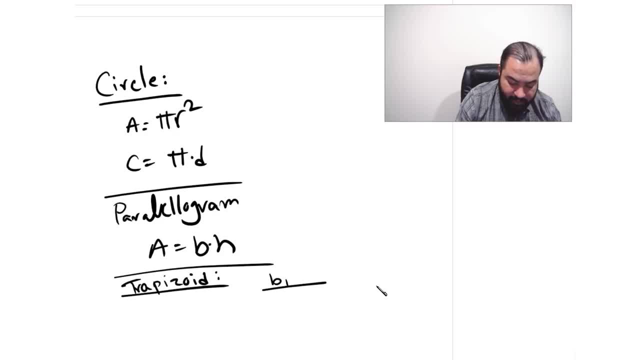 So the area of the trapezoid is base one plus base two. And you see about height Divide by two, Right, And how a trapezoid looks like. You can see Something like this: So that's the base one, base two. 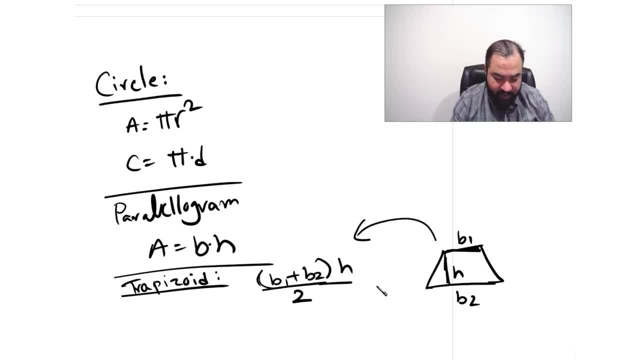 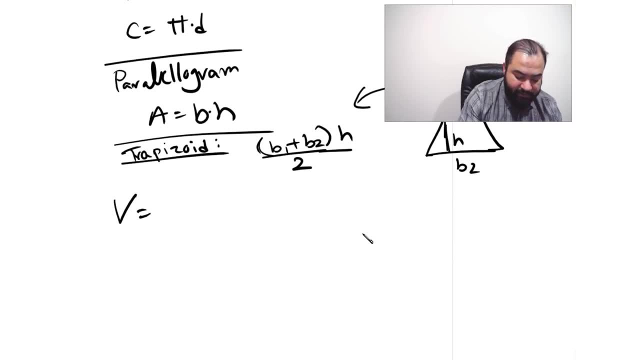 And this is the height. Now you can just plug it into the formula to find it Right. And then I showed how do you find the area of volume of the triangular prism. So that's capital B times the height. The area of the base times the height. 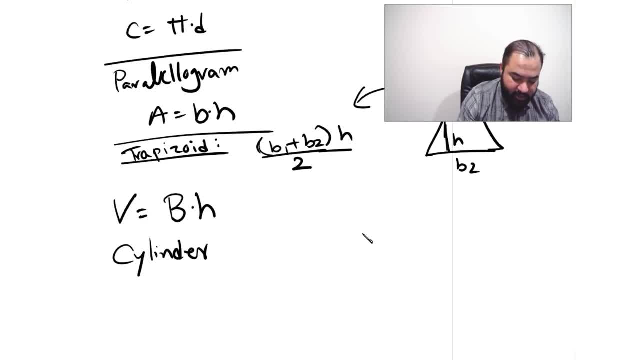 Right, And I said how to find cylinder. you do pi times radius power, 2 times it by height, right? And let's do one question. let's say radius is 3 and the height is 4, so how do you find? 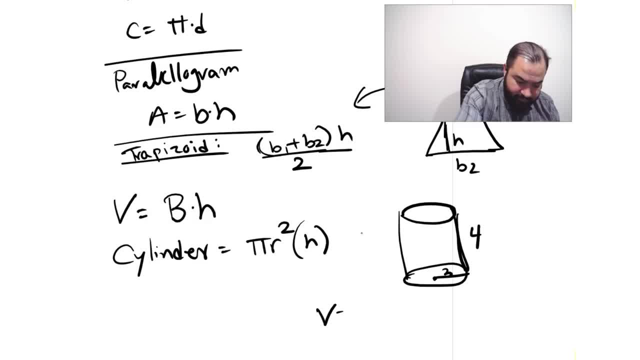 the volume You do. I can put it here: how do you find the volume? so you do, pi times radius is 3 power 2 and then times it by 4, so that's 9 times 4, 36 pi. 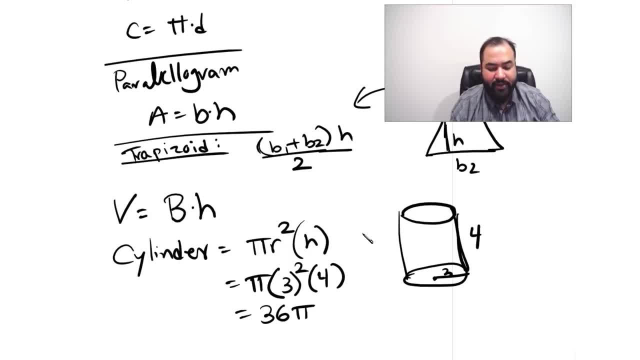 I'm giving you a brief explanation here. I'm assuming you have a certain level of background and basics, so you understand what I'm doing And that's pretty much it. these are the basics. these are more common things that you can expect. 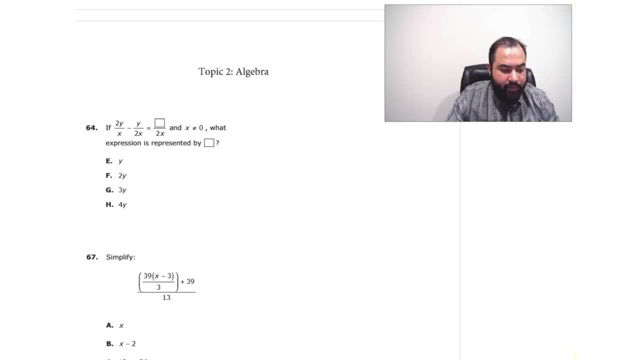 Now let's do some algebra questions, right? So, algebra, the first question is asking: these are the types of questions you're going to be facing. So, as you can see, this is a fraction subtraction. so what do we do in the fraction subtraction? 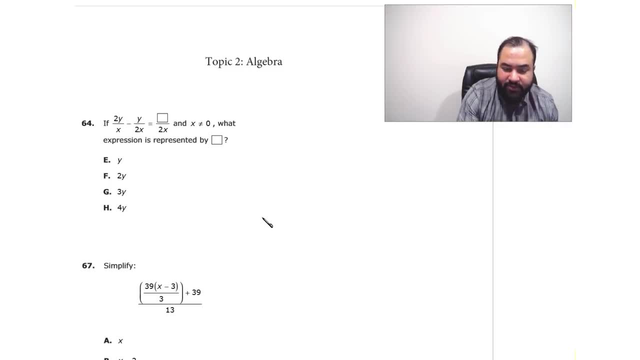 We want the common denominator right. So denominators, we want it to be same. so I have a 2x, I want this to be 2x. so what do I multiply this by? I multiply it by 2, top and bottom right. 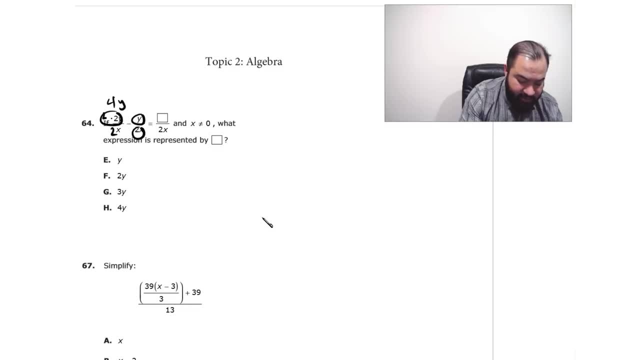 So this becomes 4y, and minus the y it will become 3y. that's where the answer is 3y. You know common denominators and that's it. Let's do a simplification involving algebra. So this one can be done a couple of different ways. I'm going to show you the most general. 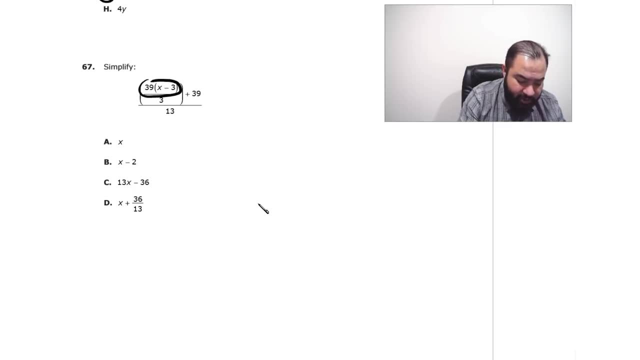 basic way. So at first let's work with this part where we can distribute right. So I get 39x minus 3 times 39 is 170, okay, divided by 3, and then there's a plus 39 and then over 13 overall. 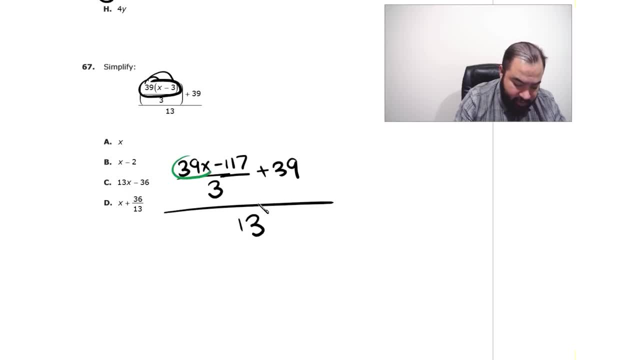 So now, when you divide by 3 here, guys, remember, you have to divide by 3.. You have to divide by 3.. You have to divide by 3.. You have to divide both 39x and 117 by this 3, okay. 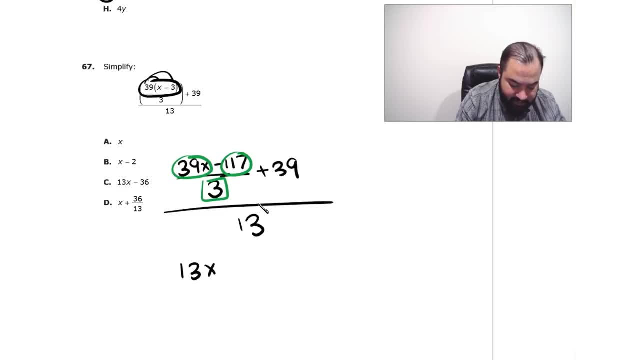 So let's see: 39 divided by 3 is 13x and 117 divided by 3 is 39. because you know, when you multiply by 39 by 3, we got 117, and then we have a plus 39 here and over at the bottom. 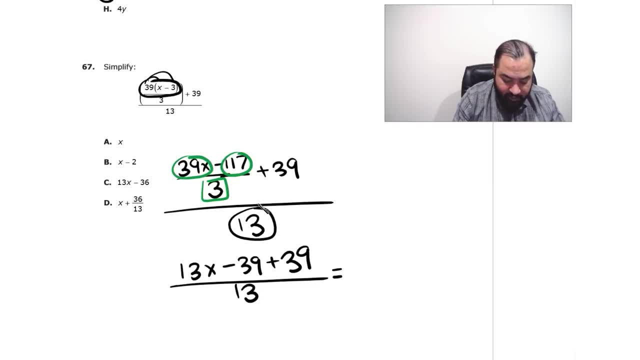 we have another 13,. don't forget that right. So now this 39 is a negative, it's a positive, so it becomes 0.. So we have just a 13x on top, 13 on bottom. we can take out the 13s. all we have is x. 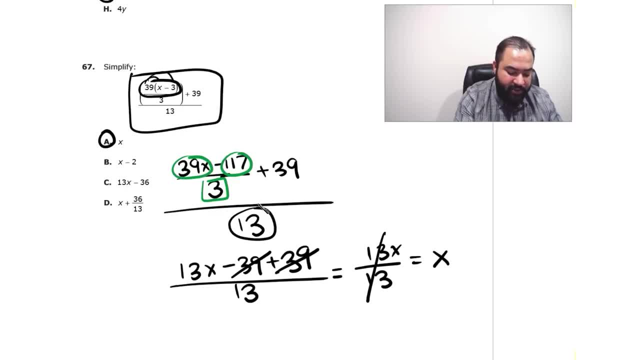 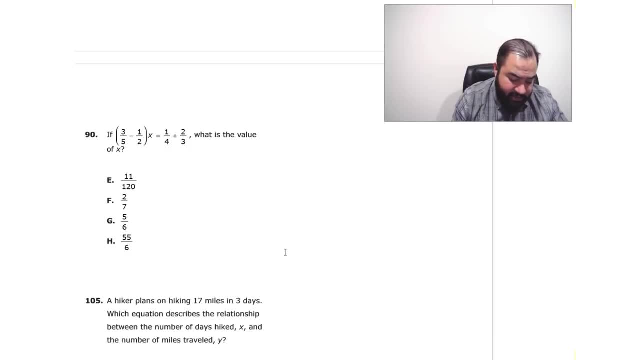 I will suggest that you practice it on your own, like: copy this question on a notebook, pause the video, try it before you move on. Alright, now question another one. this is again fraction subtraction. right, When you do fraction subtractions, we want the denominators to be same. so 5 and 2, so. 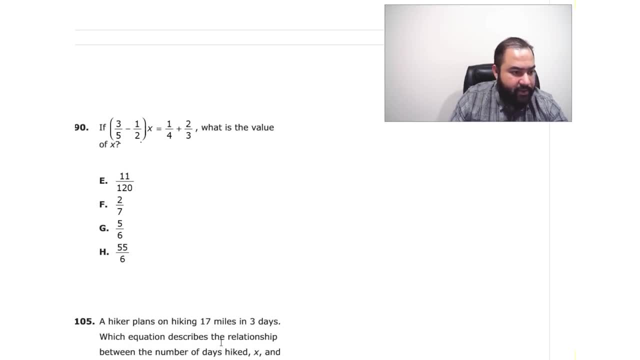 we want. let's zoom in a bit so you guys can see it better, Okay, Okay, Okay, Okay. So 5 and 2 denominators. so I will multiply the 5 by what: 2, this one by 2, this one by 5, this one by 5.. 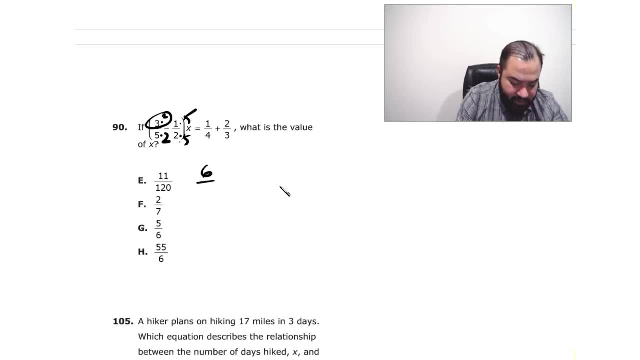 So I have a 6 over 10 and minus 5 over 10, and remember, out of the parenthesis, there is an x On the other side. I could also do. you see, here I am adding the fractions, so the denominators. I want them to be same: 4 and 3.. 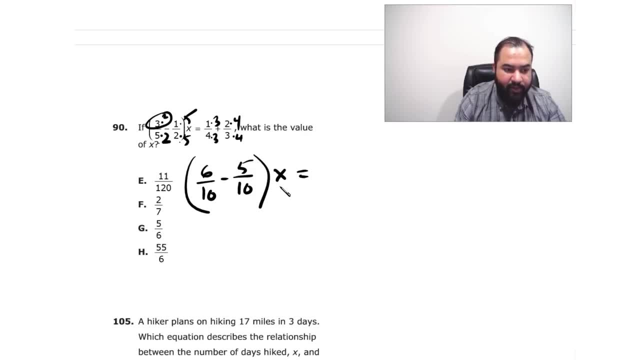 So times this by 3., 3., 3. And this by 4. 4. Right. So what do we get? 3 over 12 plus 8 over 12. Right. So if we subtract this, 1 tenth x equal to 8 plus 3 is what? 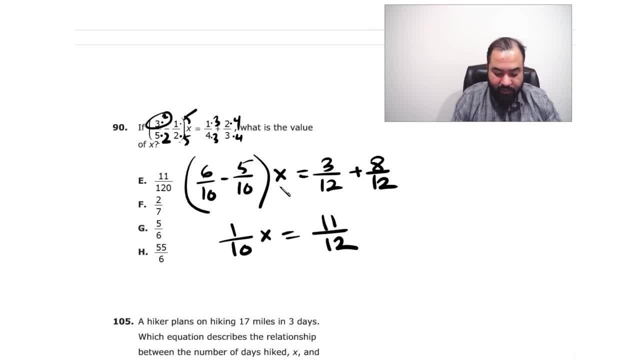 11 over 12.. Now, how do you solve for x? Now you can, you know, when we isolate the variable. let's say you have 4x equal. let's say you have 4x equal to sorry, 4x equal to 8.. 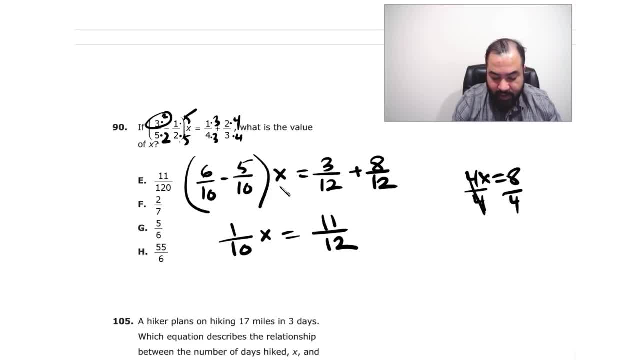 How would you solve for x? Divide both sides by 4.. Right, So whatever is next to the x, the coefficient of x, the number next to it, we divide by that. So you could divide both sides by 1 tenth, like this: 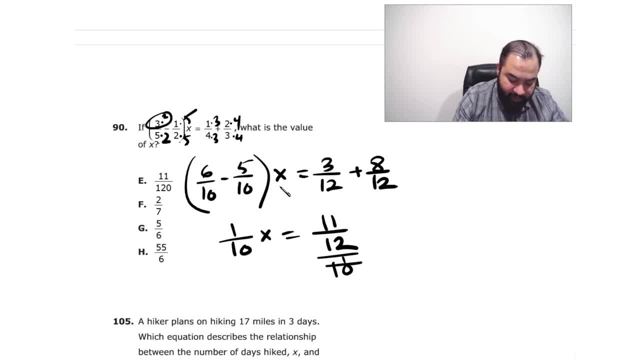 Right? Or what I prefer is: you see, the denominator is 10.. Oh sorry. So what I can do is just multiply both fractions, both sides, by just 10.. You'll be like, why? So if I just times it by 10 over 1 from both sides, the 10 in the numerator will cancel. 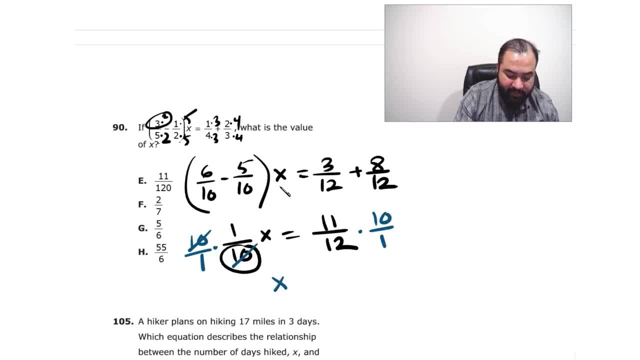 out 10 in the denominator. So the only thing that remains is x. So 11 times 10 is 110 divided by 12.. If I simplify it, it means divide both by, let's say, 2, I get 55 over 6.. 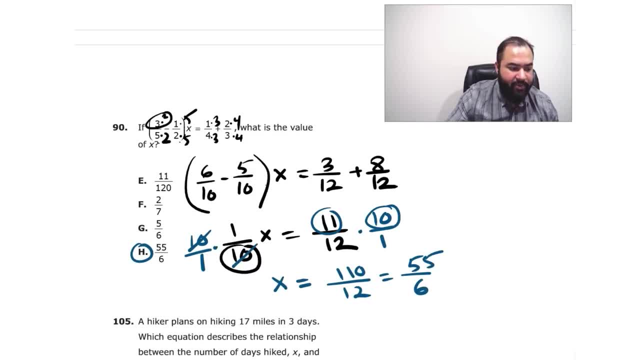 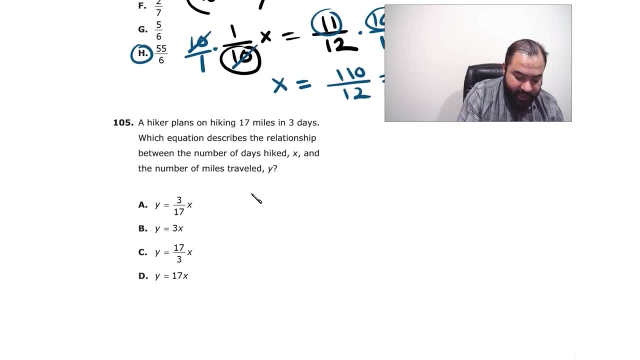 I'm assuming you guys know how to simplify the denominator with the numerator. I will explain it later in the video. So let's say here another algebraic equation. So a hiker plans on hiking 17 miles in 3 days. So when you're dealing with work problems like read one line, take some notes, like 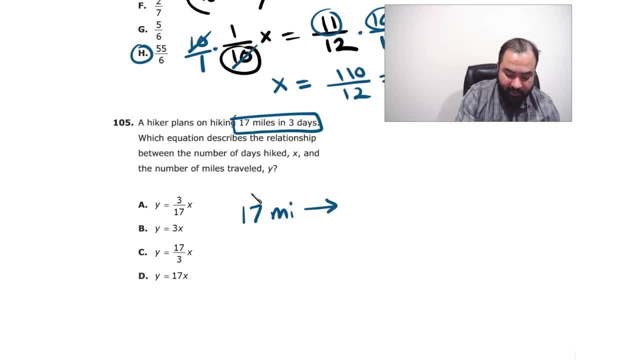 take out the outline like this: So 17 miles on 3 days. Write that down very quickly. And then so the unit rate. the unit rate means per day, So we divide 17 by 3.. Whatever I get this, this is like in 1 day. 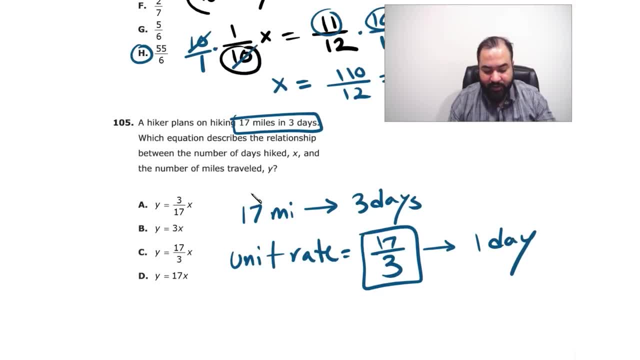 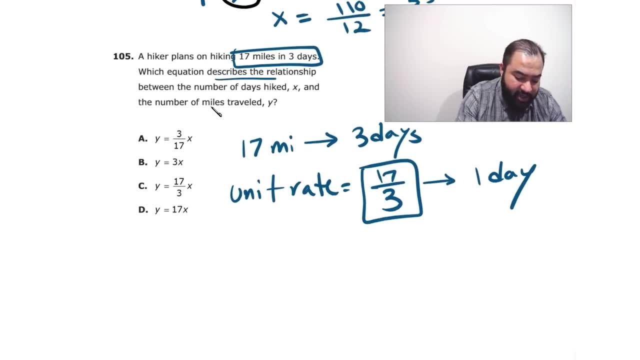 Right, Because 17 miles in 3 days for 1 day. you divide it by 3. That's called unit rate, That's 1.. Now which equation describes? okay, which equation describes the relationship between the number of days height? 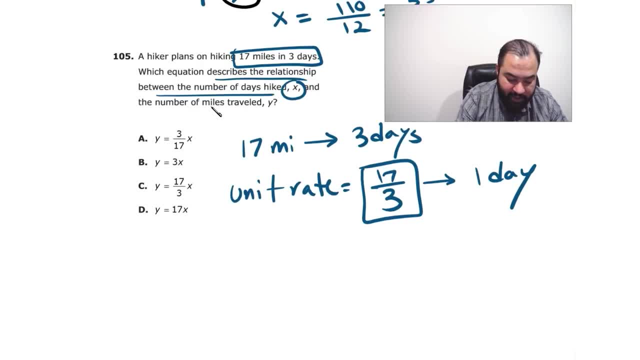 So the number of days is x And the number of miles traveled y. Right, So one day it's 17 over 3.. Right, One day you go 17 over 3 miles. Now they said x days. You see number of days x. 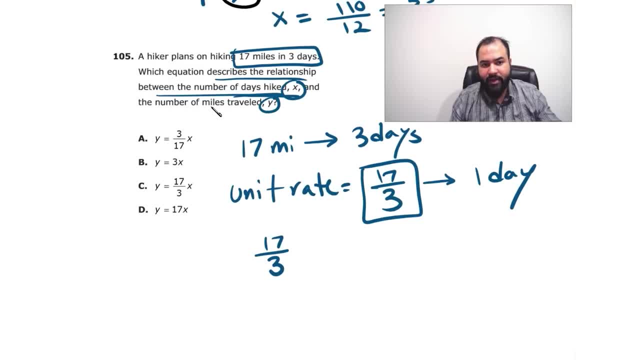 So let me ask you this: Like: if one day is 17 over 3. 5 days will be 17 over 3 times it by 5.. For 10 days: 17 over 3 times it by 10.. For x days: 17 over 3 times it by x. 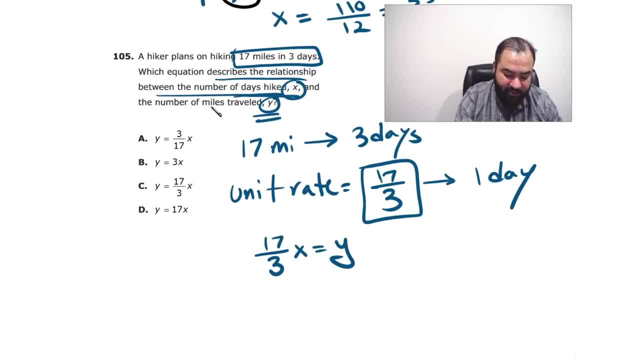 And that's the total. y Be like. that's the total travel, Because y represents the number of miles traveled all together. So y is equal to 17 over 3 x times it by 17 over 3 times it by x. 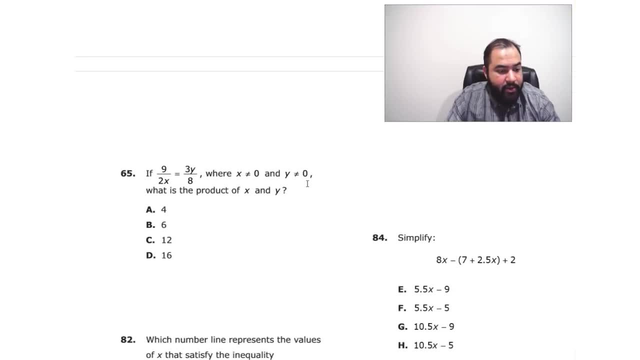 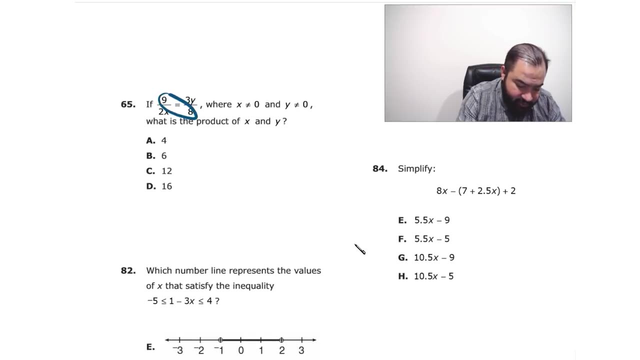 That's a Alright. now here are a bunch of algebra questions. Let's do this one first one. So it's again: it's an equal sign in the middle, So you can just cross multiply. So 2x times 3x is 6xy. 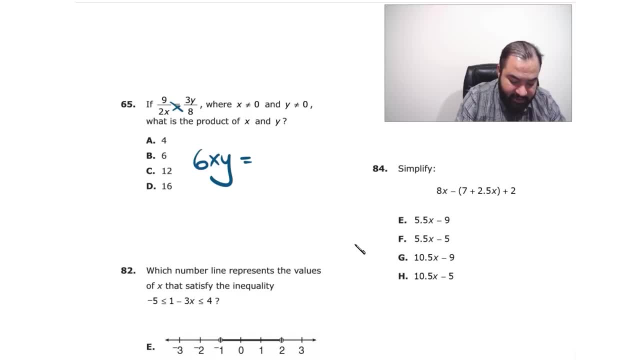 2x times 3y And 9 times 8 is 72.. Now look what is the question I'm asking: What is the product of x and y? So they said x cannot be 0, y cannot be 0.. 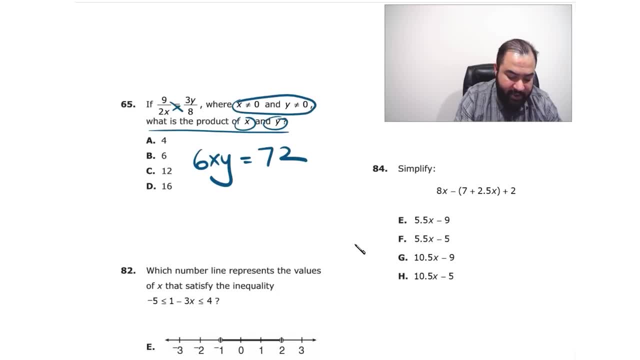 This is just an extra piece of info, Don't worry about it. They just want to know. product of x and y means x times y, So here I have x times y. Let's just divide by this 6, both sides, So I get xy equal to 12.. 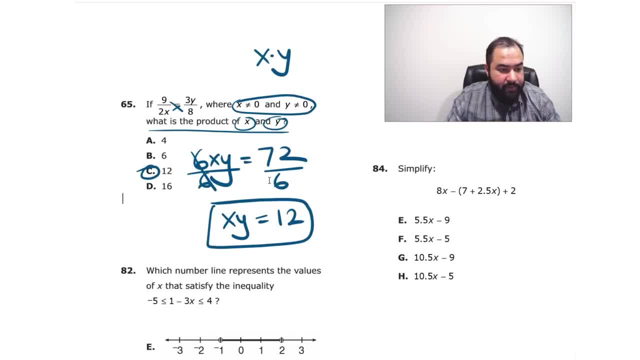 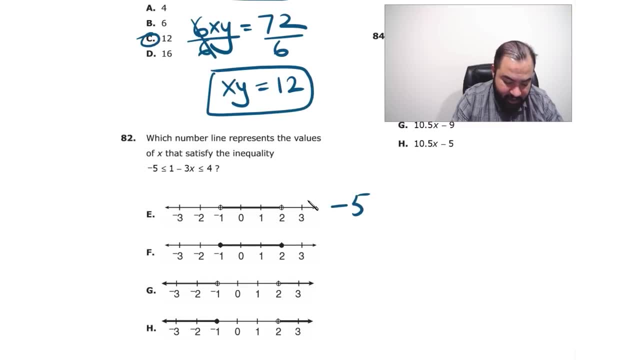 Yeah, That's the answer Simple. You can pause the videos and always practice. So I have an inequality here. It says negative 5 less than equal to 1, minus 3x less than equal to 4.. So first of all, if I were to ask, 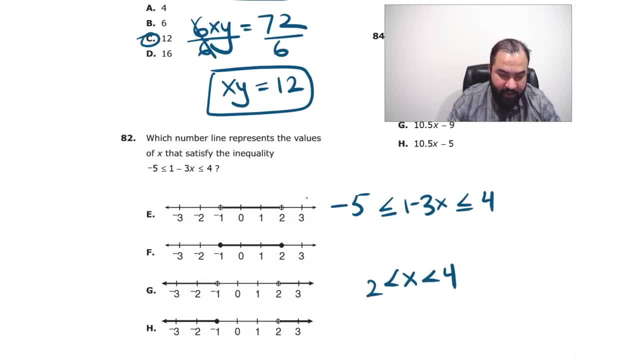 If I say, okay, graph this. X is greater than 2, but less than 4.. Right, You'll be easily able to graph it. You'll be like: okay, you know, let's say this is 0.. Let's say this is 2.. 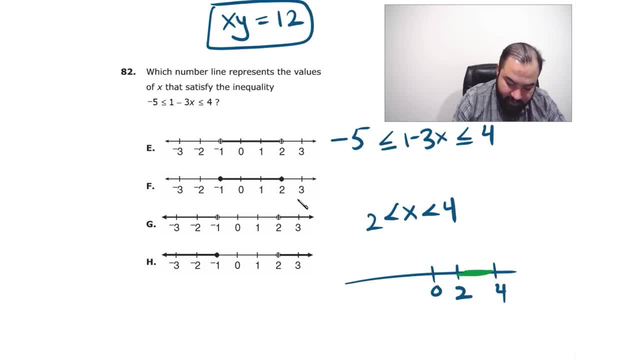 This is 4.. X would be somewhere here. Right, You would just like do it that way, But look at the difference. Here in the middle I have just x by itself, But here I have not x. I have a 1 and minus and 3 times the x. 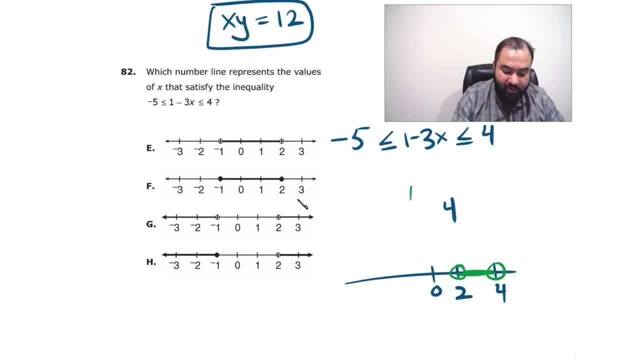 You get it. So I have to solve for x. We're going to solve it like, similarly as Equations. So first of all, what we can do is: You see, there's a plus 1.. We can do minus 1 from each and every side. 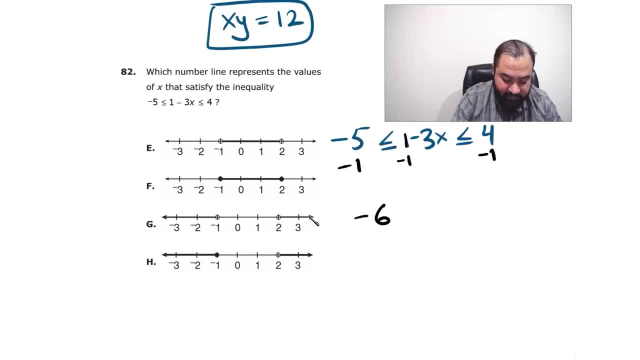 So 5 minus 1 is negative 6. Negative 5, negative 1 is negative 6. And here, 1 minus 1- cancel out- is negative 3x less than equal to 3.. Now it says I have to solve for x. 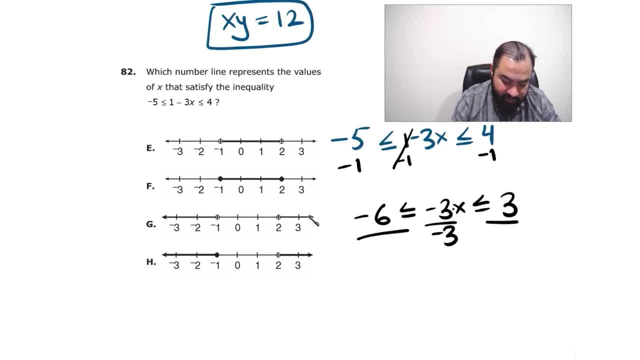 So I divide by what number, guys? Next to x is a negative 3.. So we divide by negative 3, each and every side Right. So we get x. is what, When you divide by a negative number in inequality, what happens, guys? 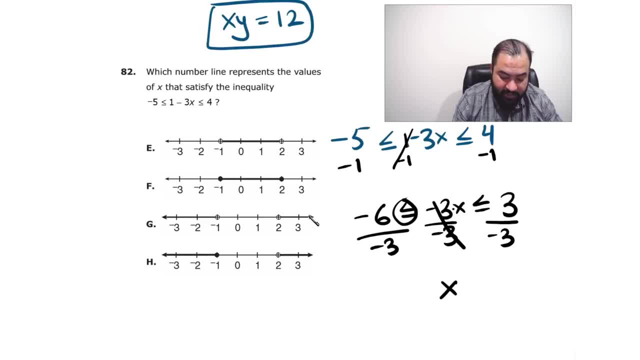 The inequality flips. You see, this is less than I mean greater than Now. it will change it to less than This will also change The whole inequality will flip. So negative 6 divided by negative 3 is just 2.. And 3 divided by negative 3 is 1.. 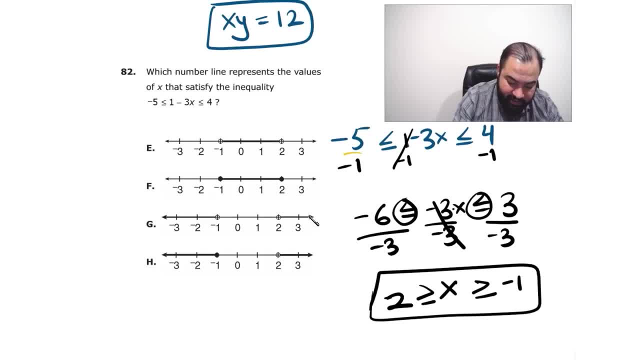 Negative 1.. Now take a look at it. When I subtracted negative 1 from each and every part of the inequality, I didn't flip the sign. That happened when I divided by a negative number. You see, divided by a negative number. that's when the inequality flipped. 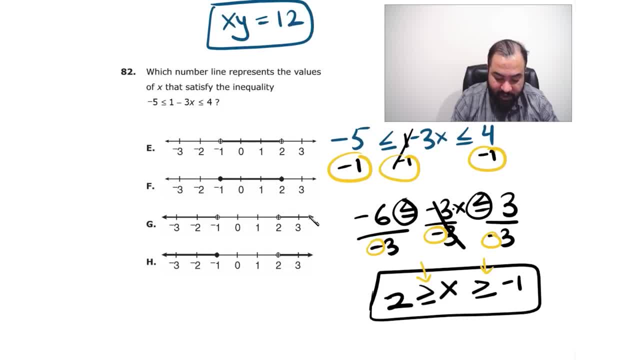 Now you can graph it: x is greater than equal to negative 1 and less than equal to 2.. So that's f, You see, greater than negative 1 to 2 is in the middle. That's it. Let's do 84.. 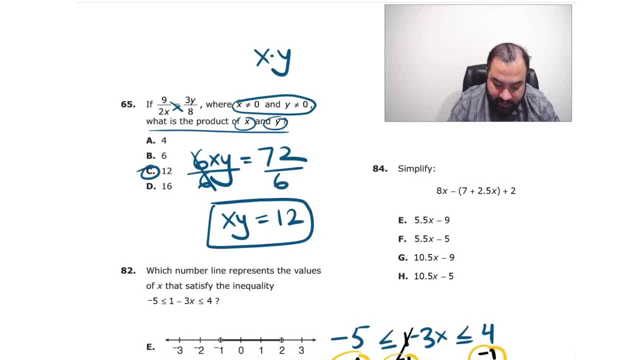 The reason I picked this question here is because you see, the negative here is very important. The negative changes the sign inside the parentheses, So you guys probably know how to distribute already. as I'm assuming that you know the basics for this video, I can make other videos later, probably for basics. 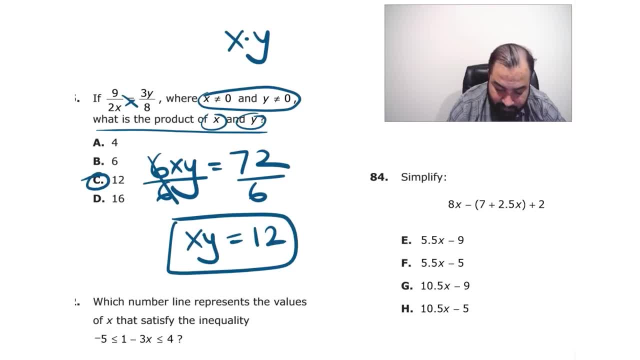 or you can join my classes to learn, of course. So here there's a minus here, right? Remember one thing, guys: If you have 8, let's say here, and parentheses x plus 5, you see, the number 8 is right next to the parentheses. 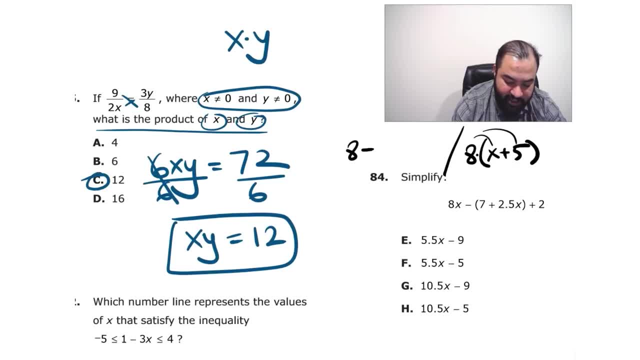 So you can distribute. But if you have something like this: 8 minus x plus 5, you see that 8 is not next to the parentheses. So what is next to the parentheses is an invisible 1 here, And that negative 1 will be distributed. 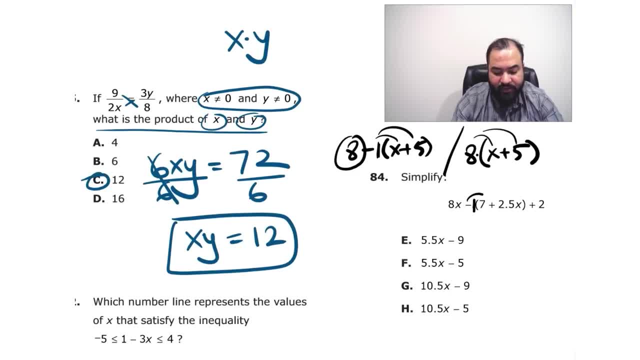 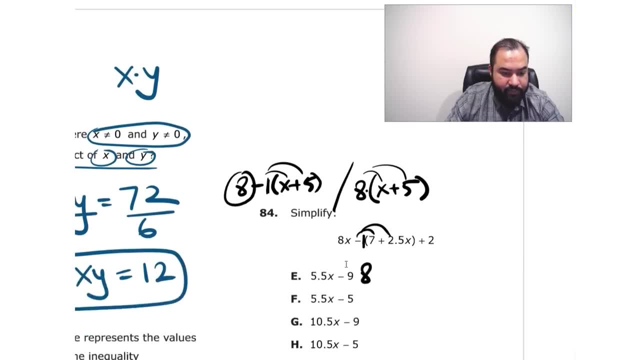 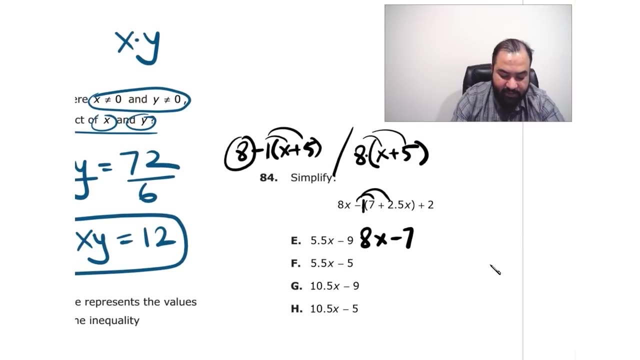 So I can put an invisible 1 here. You see, invisible 1.. Now distribute the invisible 1.. So you get 8x. Let me move it to the middle. So 8x minus x, Minus 7, because negative 1 times 7 is a negative 7.. 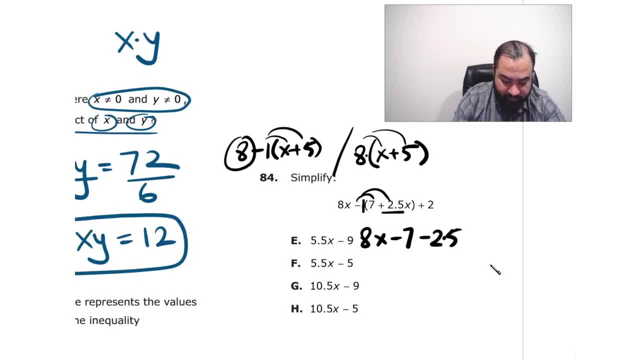 And negative 1 times positive. 2.5 is negative 2.5x, And then there's a plus 2.. So now I can just combine the like terms: So 8x minus the 2.5, that's 5.5x, I believe. 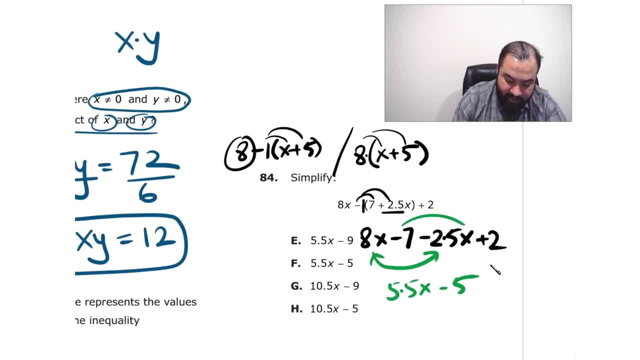 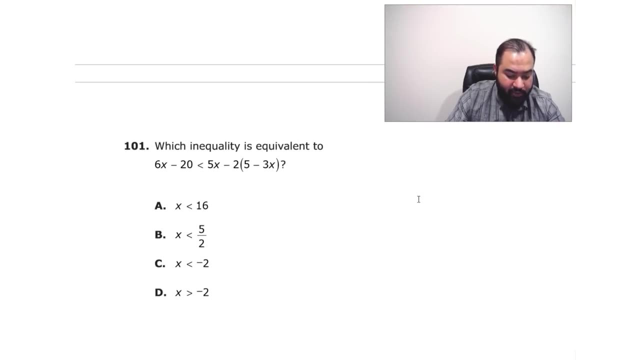 And negative 7, positive 2, that's negative 5.. So 5.5x minus 5, that's f. Remember guys, this negative 1 here has to be distributed. Now let's continue. One more here: inequality. 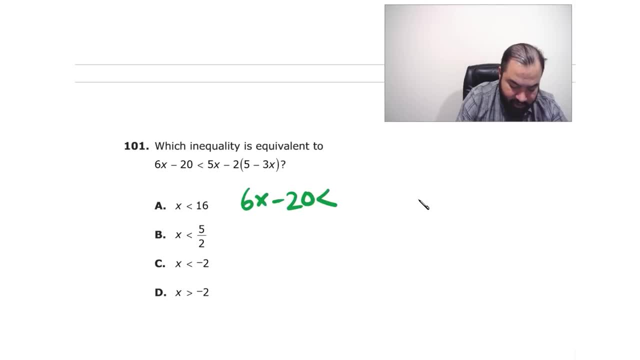 Let's solve this inequality. We have 6x minus 20, then 5x We can distribute here, So you get a negative 10 and a positive 3,, sorry, positive 6x, Because remember this negative will be distributed. 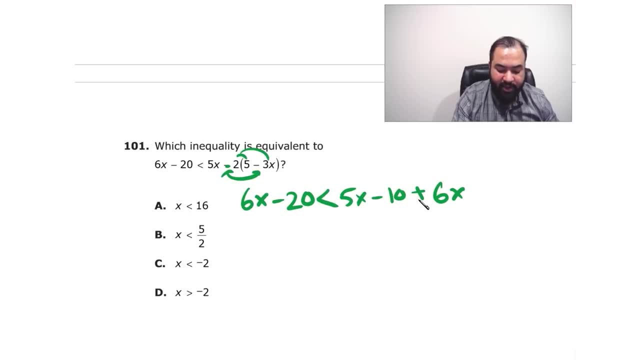 Don't forget This negative and that negative will make it positive. So now I have a 6x minus 20.. And 5x and 6x combines to what 11x minus 10 here. So you know what we can do is plus 10 both sides, right. 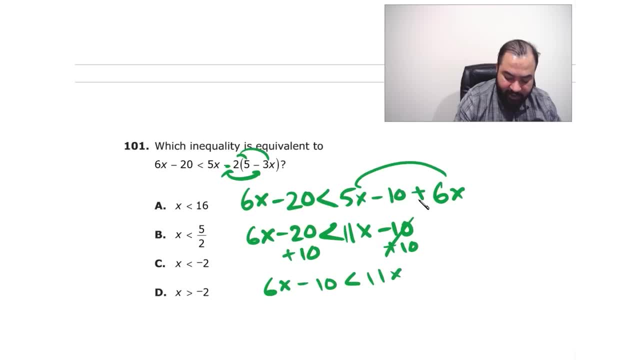 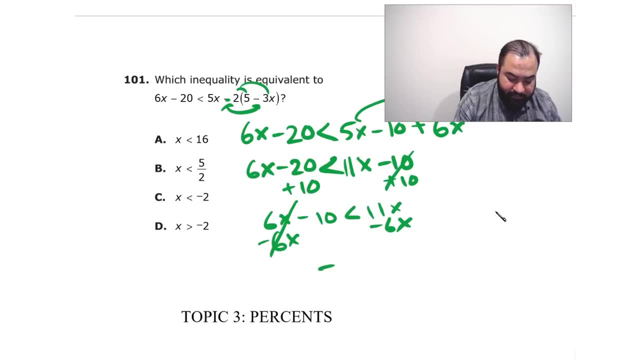 So we have 6x minus 10 less than 11x. Now we can do minus 6x both sides, right. So we get negative 10 less than just 5x, Right? So how do we solve for x? 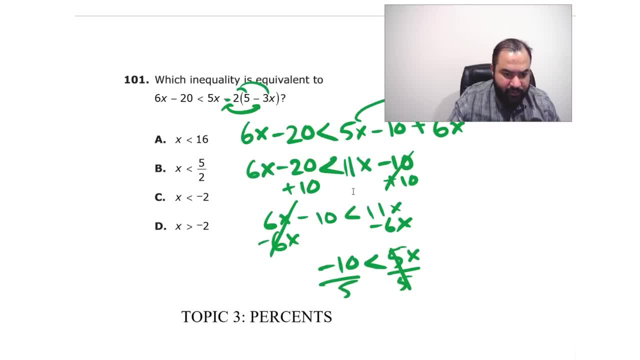 Divide both sides by 5.. So when we divide by 5, do I flip this inequality in the middle, guys? No, because I'm not dividing by a negative number. If I were to divide by a negative number, I would have to flip it. 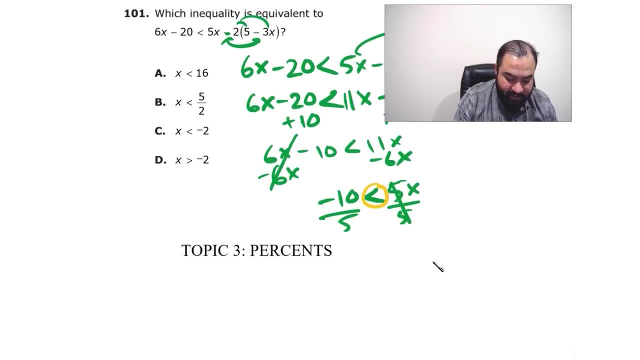 It doesn't matter if there's a negative on the other side, It doesn't. So when you're dividing, the number you're dividing on the bottom has to be negative. So I get negative 2 here. So x is here, then negative 2.. 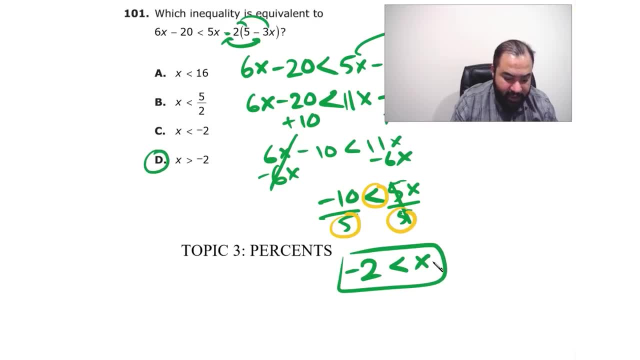 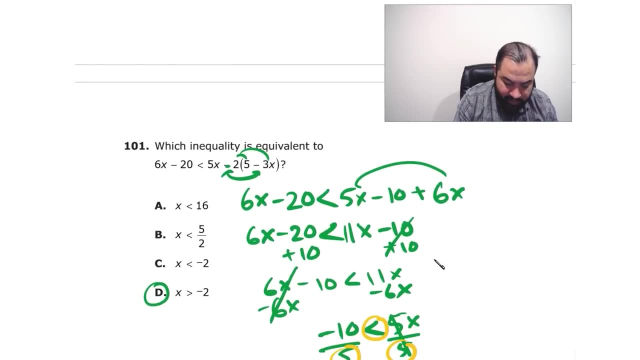 It must be d So let's see if I did it right. So I'm just going to double check my work. So 6x minus 20, less than 5x, that's negative 10,, positive 6x: yes. 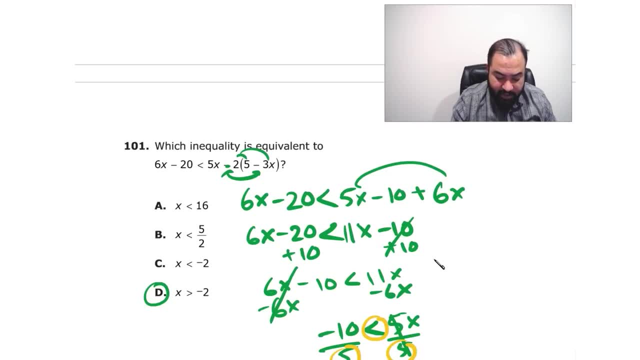 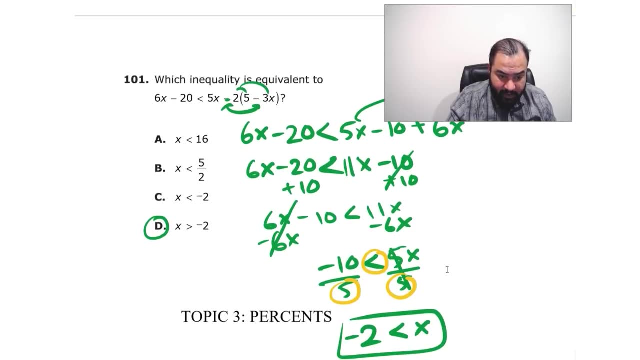 So that's 6x plus 10 both sides. we did huh, So that's negative 10, then minus 6x. So 11x minus 6x. yes, So that's negative 10 divided by 5, which is negative 2 should be fine, yeah. 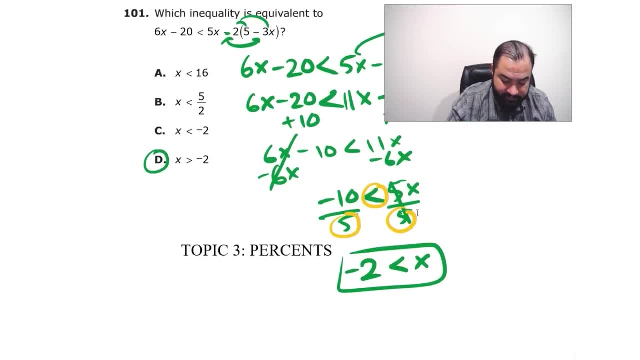 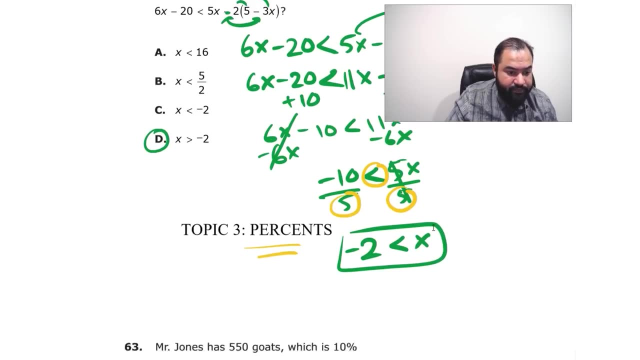 So x is greater than negative 2.. That's this one d. All right, that's it for that. Now we're going to learn some percentage For percentage guys, before I go to the question, I'll give you a lesson on percent. 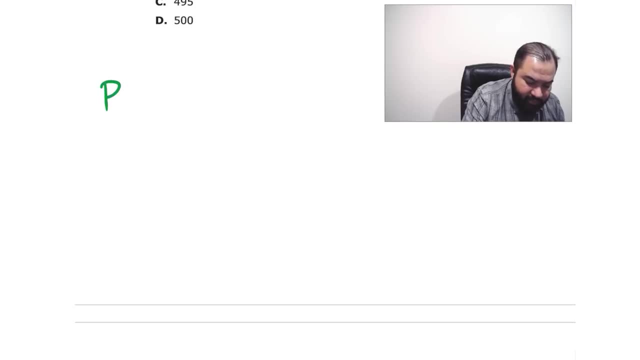 So how does this percentage work? So percent, there are three types of percentage. First type: you guys know that. let's say what is 20% of 50. You know how to find it. 20% means what like one-fifth. 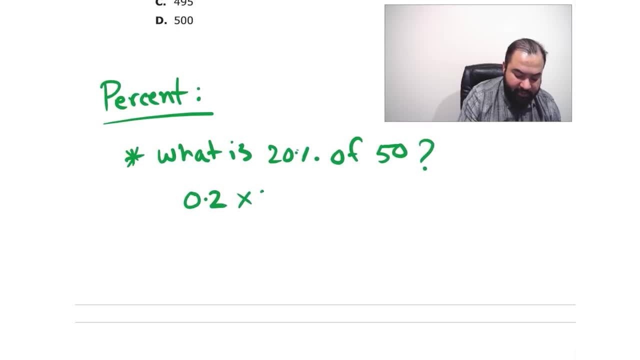 Or 20% is also 0.2, right Times it by 50, that gives you the answer. That's the simplest form of how to find percent right. 20% means 0.2.. Like you know, move the decimal two times. 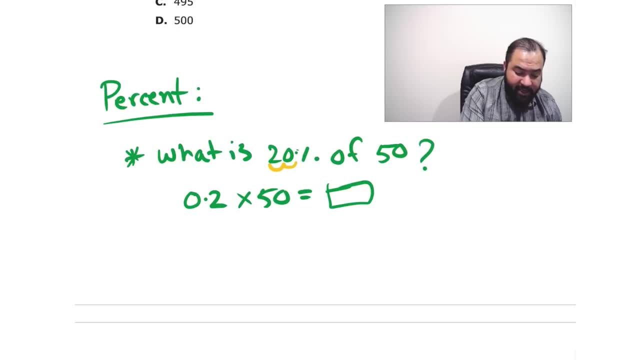 That's 0.2, right. The second type you're going to face is, let's say, 5 is what, This is ease, What percent? or I can say, 5 is 20% of what. Now take a look at the question. 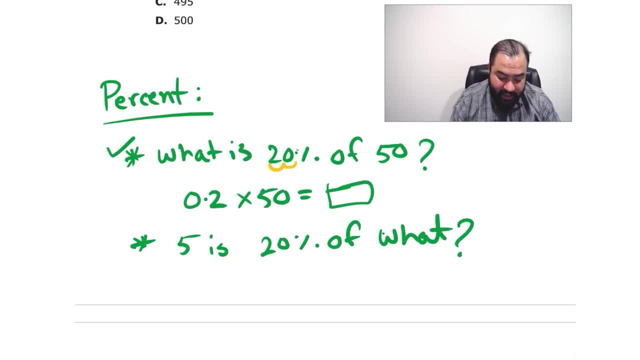 It's different than what the first question says. Here it says 5 is 20% of what? So I cannot just find 0.2 times it by 5. That would be wrong, because they said no 20% of whatever, that number, 0.2 times this number here. that's missing. 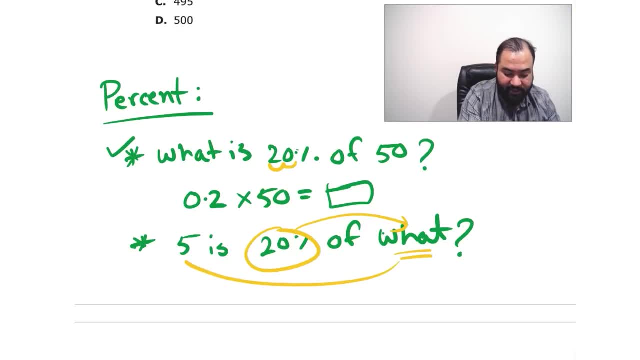 that will give you this 5.. That's what the question says. So in this case I cannot just multiply 0.2 with 5.. So what we can do, we need to set up a proportion. All right, We're going to set up the proportion like this: 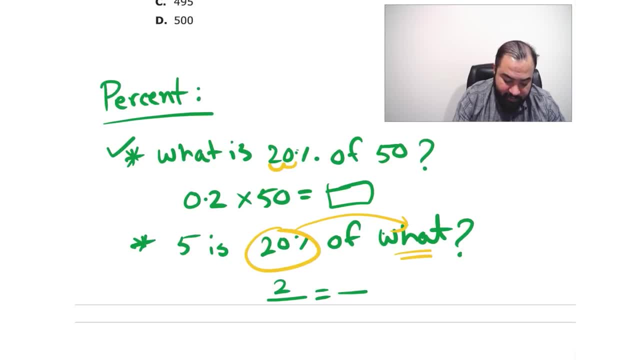 Is it draw two lines equals and in the middle. Now, 20% means 20 over the 100, right, And 5 is the 20%. So you put 5, that's the 20%. You see, 5 is the 20%. 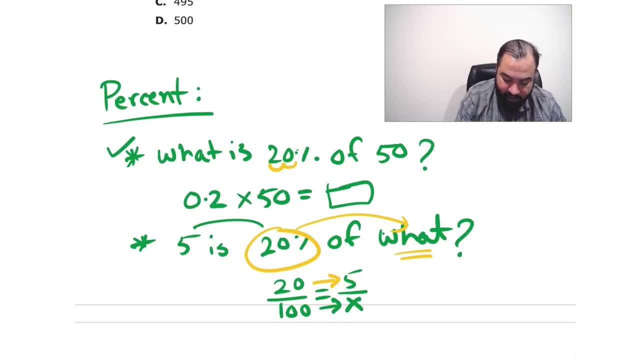 And we want to find the 100%, which is x, right, So x is the 100%. Now, solving this, you just cross, multiply and solve for x. Take a look at it again: This 20% is the 5, guys. 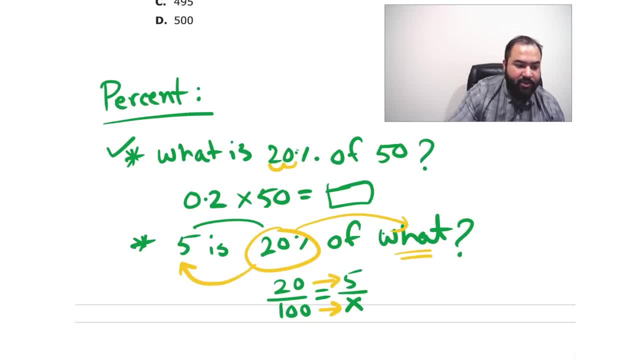 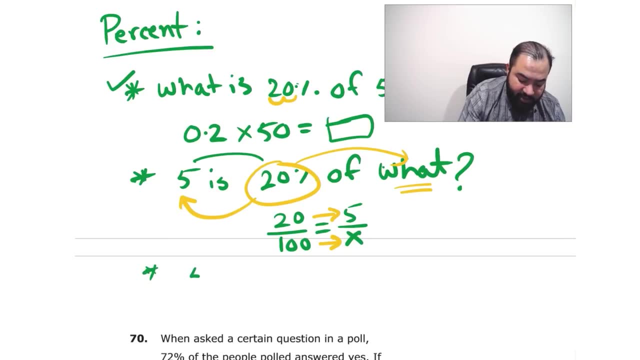 And then the 100% is what is missing. So that's x. So that's how we set up the proportion. Let's talk about a third type. It says: let's say what percent is what percent of 30?? Now take a look. 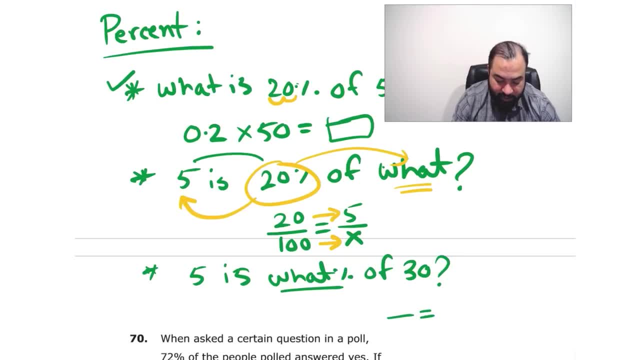 I cannot just multiply Here. percent is missing, So we have to set up a proportion for that proportion. So what percent? We don't know. It's like 5 is a part of the 30. So 5 out of the 30 is the whole thing. 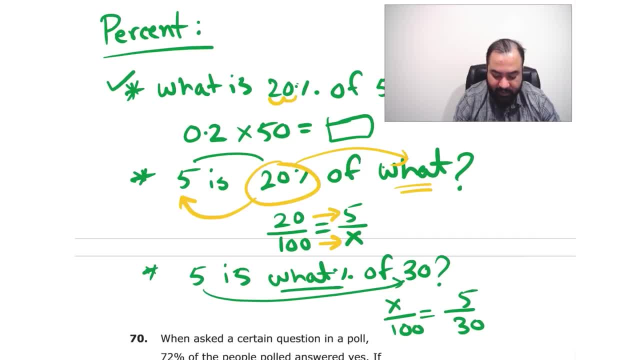 But I don't know 5 is what percent, But I know the 30 is the 100%, the total, The percentage of 5 is missing. You see, as you can see that 5, we don't know what percent. 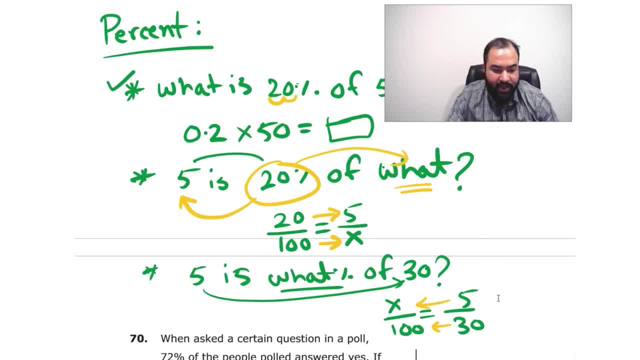 But 30 is the total, That's 100%. Now you can just cross multiply and find it. I'm assuming you know how to do cross multiplication already. All right, So these are the three different types. So you have to recognize what types it falls into. 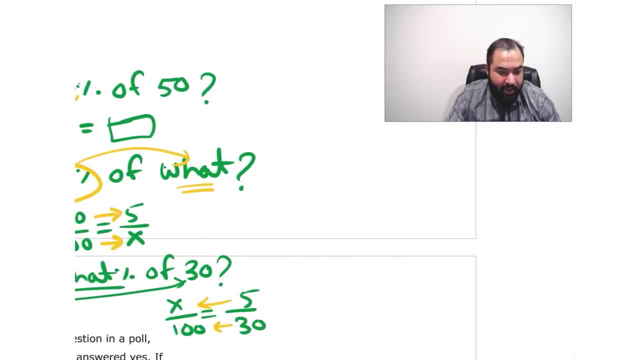 And one more thing I want to show you guys is how the increase and decrease works. So let's say you have $200.. You're buying something with $200, let's say: Then you get a discount. This $200 is the 100% right. 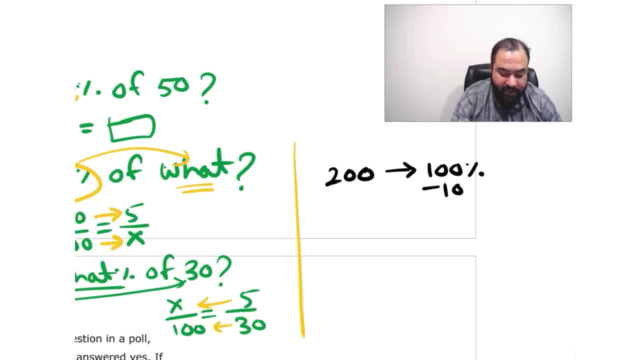 And then you get a discount of 10%. So you do minus 10%, So you are paying 90%. So after the discount, if you want to find how much you paid, you can just find 90% of 200.. How do you do that? 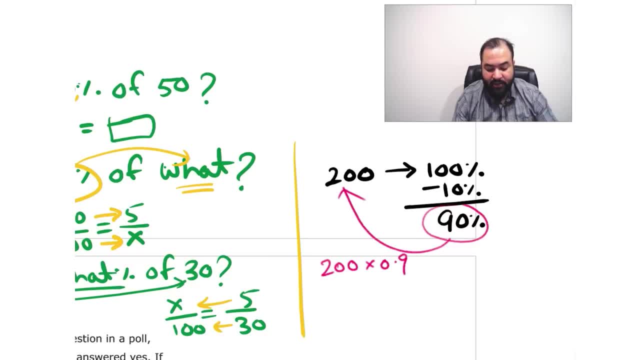 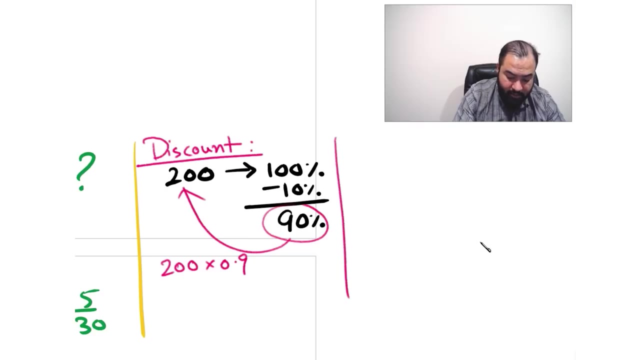 200 times 0.9.. Or there are other ways, of course. That's like discount: If you're getting discount, you can just subtract the percentage right. And the second thing you need to know is the increase, Like, for example, sales tax. 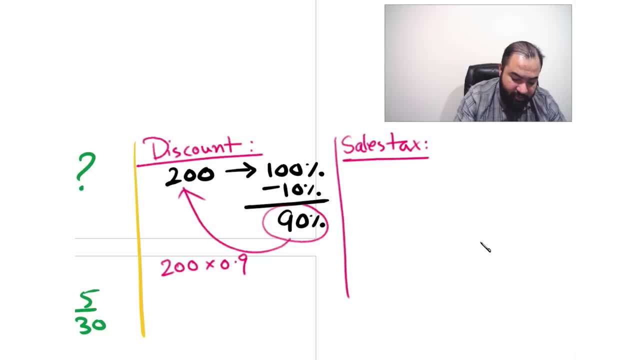 You have to pay the tax, right. So let's say you bought something with $200.. You bought something with $200. And that's the 100% And you're paying, let's say, a 5% tax. So you have to add the 5% with it. 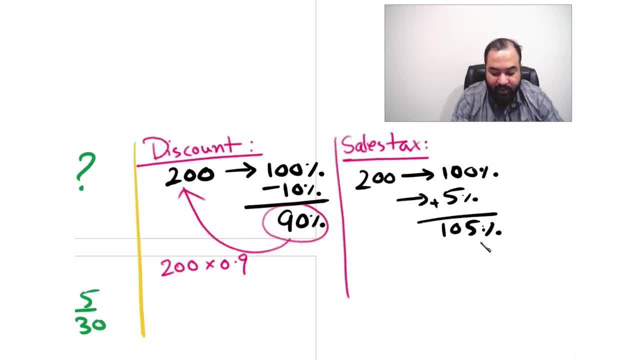 So that's 105%. So if you want to find out how much money you were paying after the tax, so you just find 105% of 200.. So that's like you know when you're adding percent and this is when you're subtracting percent, right? 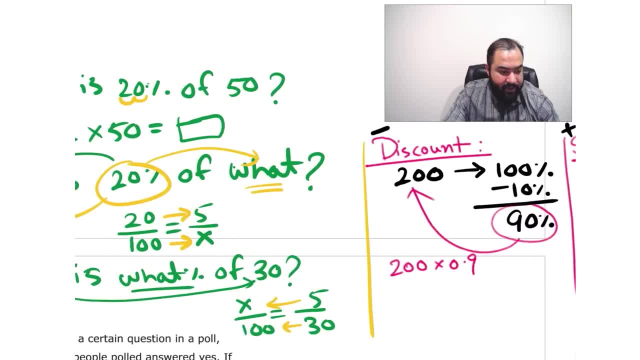 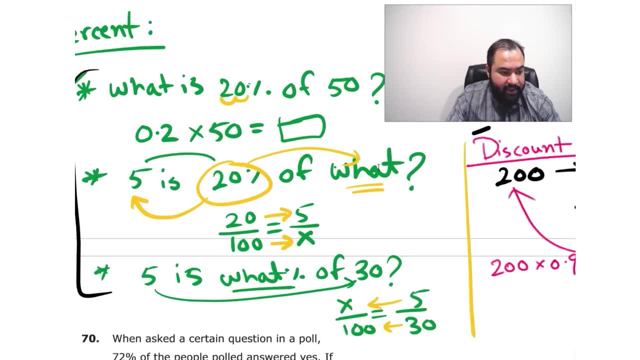 So you can always deal with it this way. So I gave you like the percentage how to think about. So these are the three main different ways. And then you have the discount and sales tax. Now let's just apply this here. 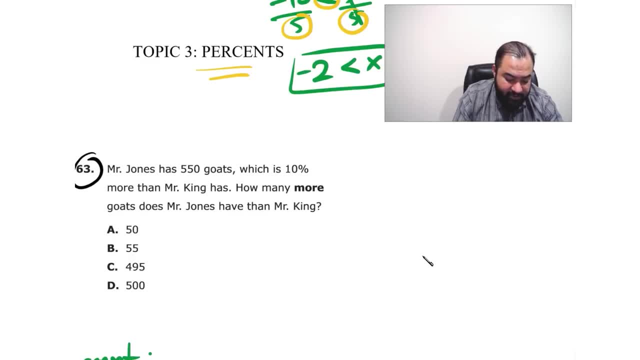 Take a look at this question here It says Mr Jones has 550 goals, which is 10% more. 10% more means what You have to add 10%. It means it's 110%, 10% more than Mr King. 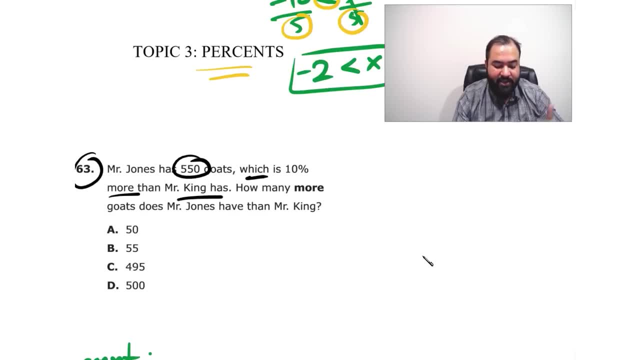 So whatever Mr King has, he has 10% more, So I can set it up. So let's say, 10% more is the 110%, And that's what is 550.. And Mr King has the 100%, which we don't know how much. 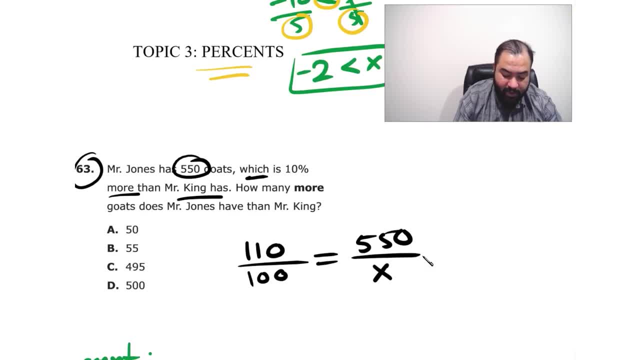 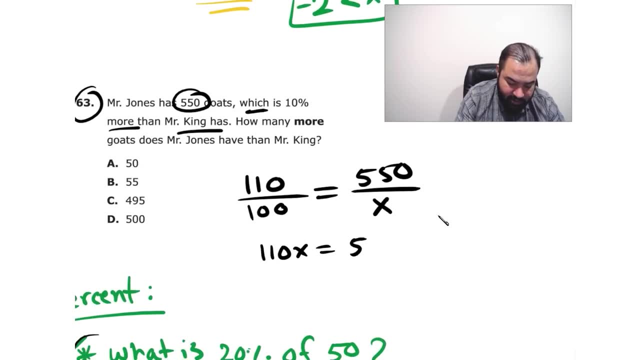 So we have to find it. Now we can cross-multiply. So if you do cross-multiply, what do you get? Multiply 110 with X 550, two more zeros. You know, you can definitely simplify which I'm coming to it. 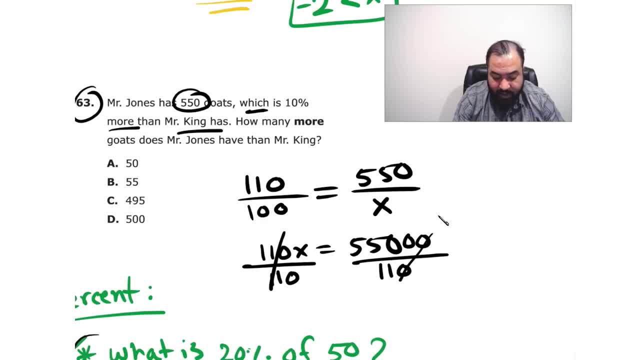 Do I have both sides by 110?? Here zeros cancel out And so X equal to 11 goes into 55, five times and two zeros. So Mr King has $500.. So Mr 500 goals, Mr Jones has 550 and King has 500. 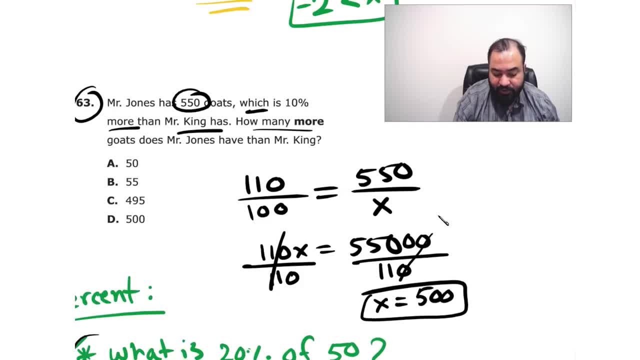 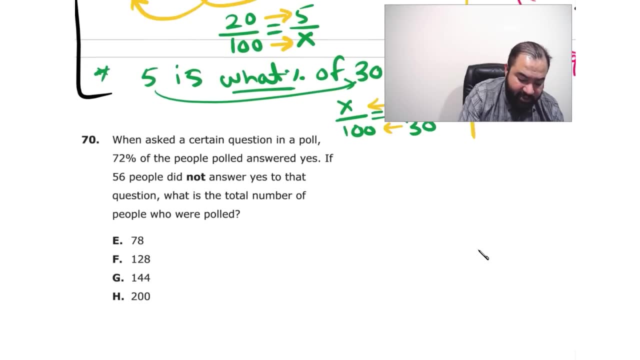 So they said: how many more does Mr Jones have? So you can just do 550 minus 500. That's 50.. Let's do some more questions and then we'll get more clear. Let's do number 70. It says okay, when asked a certain question in a poll, 72% people answered yes. 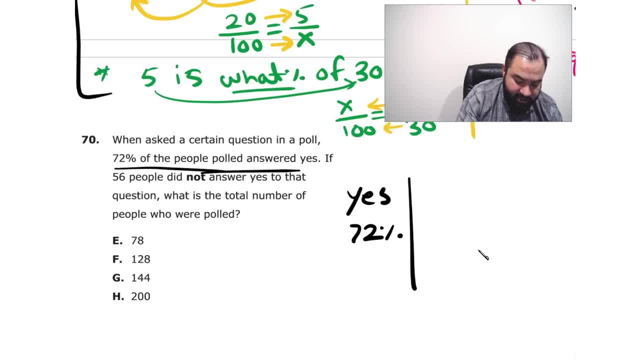 So 72% people said yes. So no is said by what? Total is 100% always. So 100% minus 72 is 28%. people said no. Now they said: if 56 people did not say yes, so if 56 people said no, then what is the total number of people there? 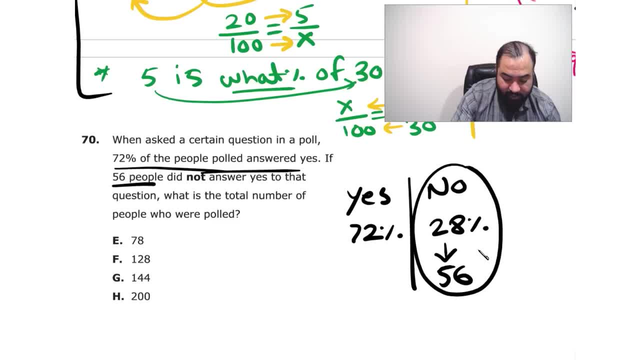 So 56 people said no. So we can set up the proportion that. all right, the 28% is the what 56.. So I want to know: 100% is what do I put here? X, That's it. 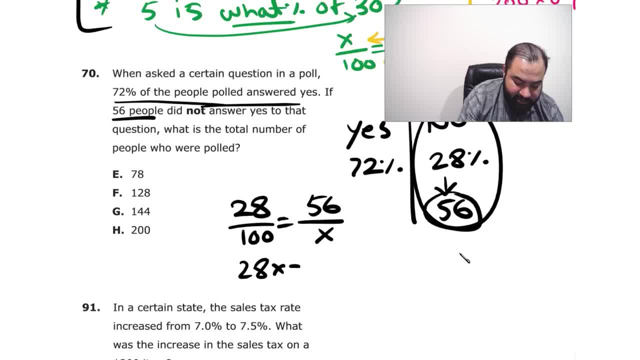 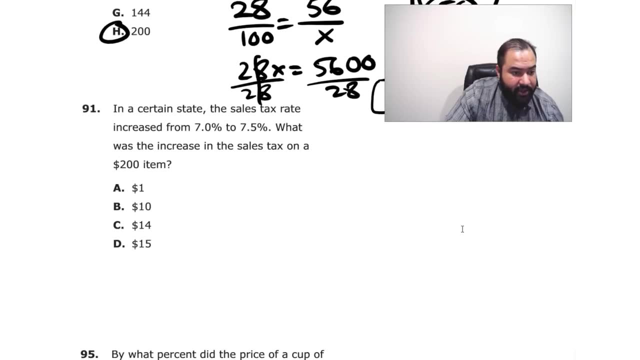 Now you just cross multiply, solve it. So it's 28X equal to 5600.. You have both sides by 28.. So X equal to 200.. So that's the total. Let's do another here. So now here, in this case they said that's a different one. 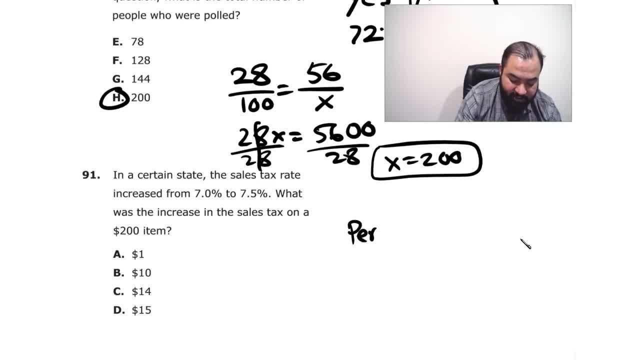 Another thing you have to know about percent is like there's a formula that's called percent change, Right, You've probably heard about it. So percent change So a number from, let's say, $5 to $8.. So it changed from $5 to $8.. 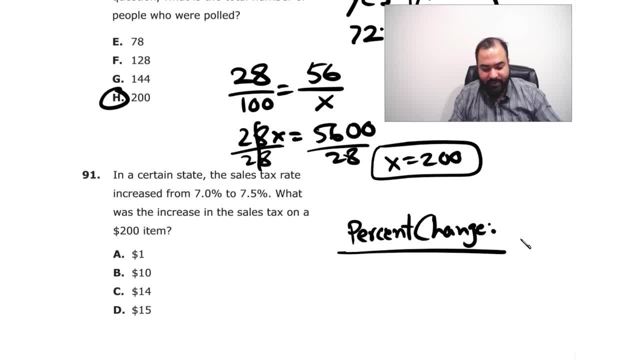 So there's a $3 difference, but they want to know what percent difference. So if you want to know the percent change, you use the formula. That's the new value minus the old one Divided by the old one: Absolute value times 100.. 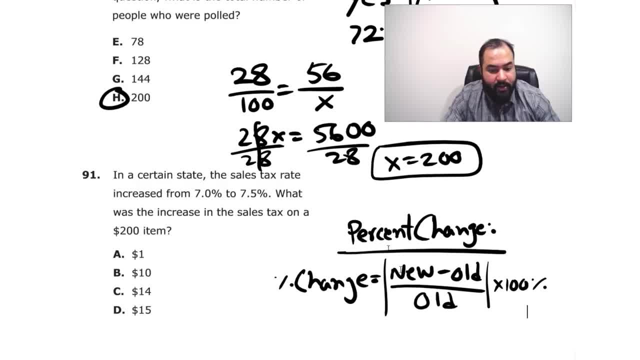 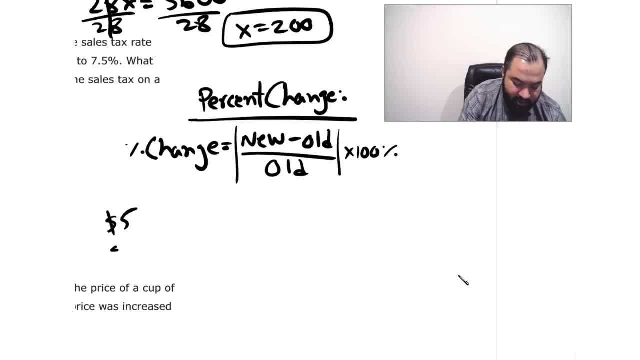 Well, it sounds hard but it's actually pretty easy. I'm going to give you an example before I move on with our questions. So let's say a product. it was $5. Now it became $10. So I want to know percent increase. 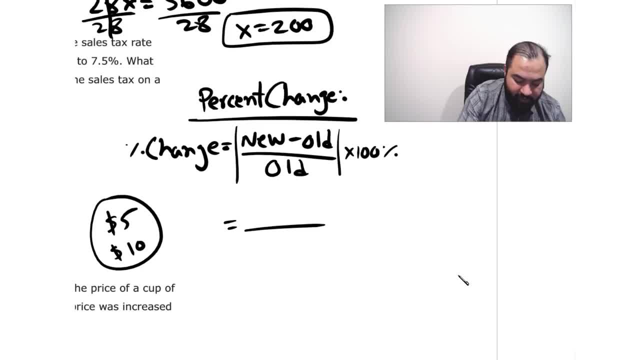 Well, it's kind of common sense, but here you can use the formula: So the new value is $10 minus the old value is 5. And then you divide it by 5.. Right, Because that's the old value, Absolutely. 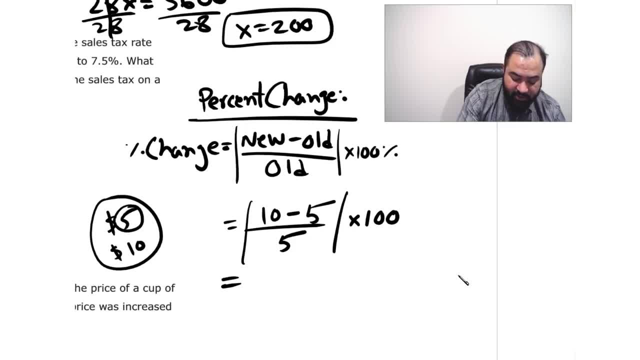 Absolute value, because you don't want it to be negative. times it by 100.. So 10 minus 5 is 5 over 5. That's 1 times 100. That's a 100% increase. Okay, So that's how we find it. 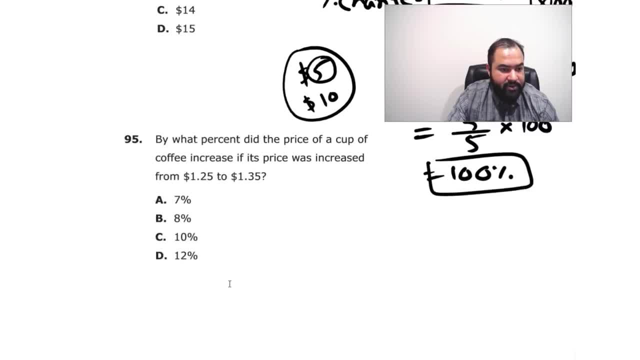 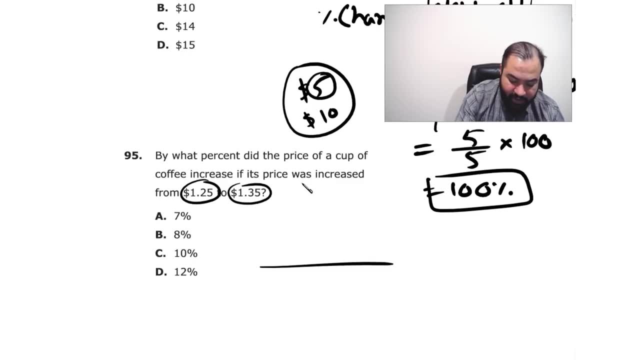 Now let's do this question here. first, the 195.. I'm going to go back to the one before it later. So let's see. So 125 became 135.. So what is the percent increase? So what is the new value, guys? the increased one. 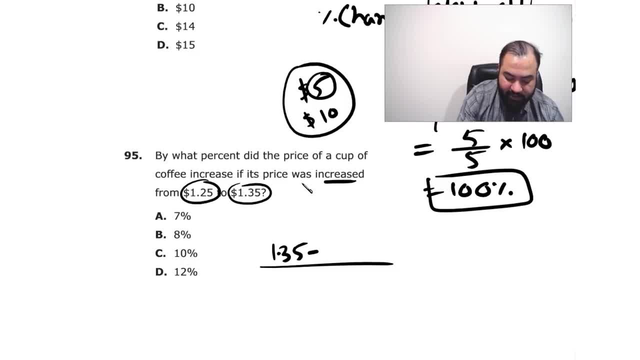 135.. So 1.35 minus 1.25 divided by 1.25.. Absolute value times it by 100.. Right Now, let's just solve it. So if you just subtract it, I think this is 0.10.. 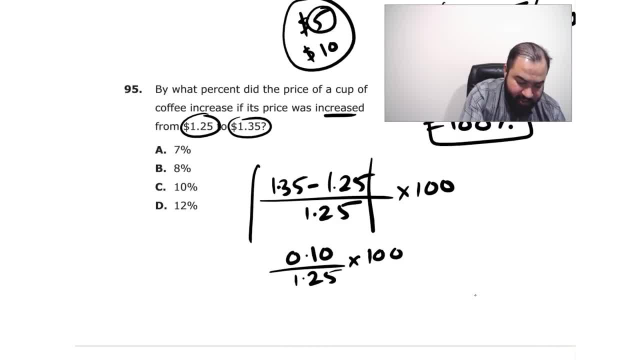 1.25 times it by 100. I can move the decimal two times to the right here also, So I get a 10 over 125 times it by 100.. Right, So that's 1,000 over 125.. 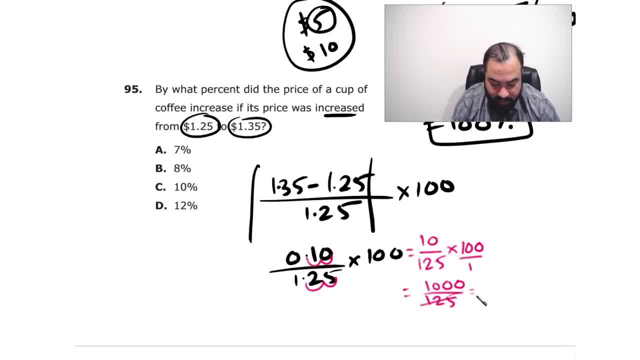 I can simplify it by 25.. 25 goes into 125. five times 25 goes into 1,000, like 40 times Right? So? and this 40 divided by 5 is just 8.. So it's 8%. 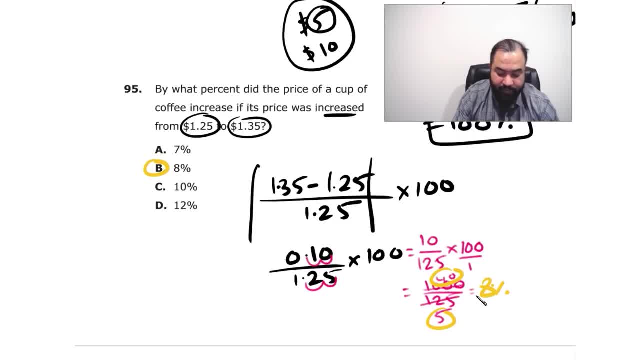 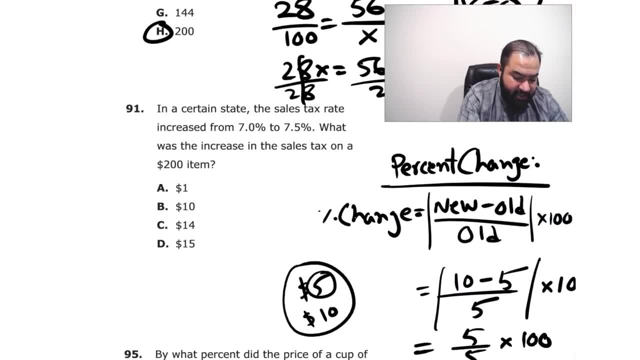 Clear. So now let's take a look at this question here. 91. It says: what is the percentage increase? 1, it says they're trying to trick you on this question. So the sales tax rate increased from 7% to 7.5%. 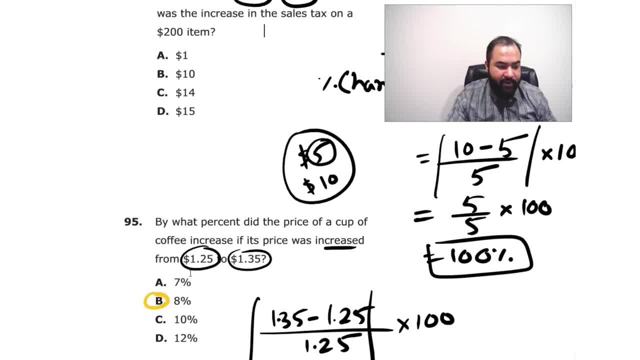 This is already in percentage. The other question we did: they were just numbers like $1.25, $1.35.. That's not percentages. So if you want to find the percent change between two numbers, then you use the formula. 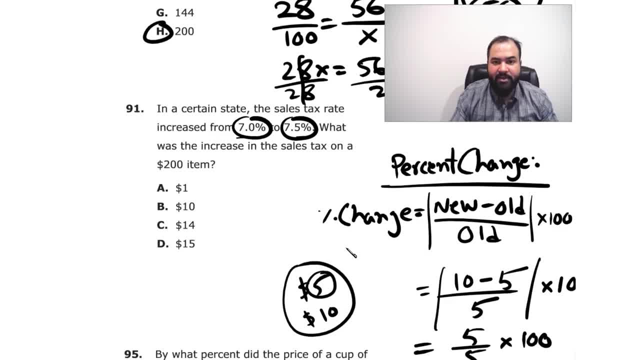 But they're already just the percentage 7 to 7.5.. I can just simply subtract 7.5 minus 7, which is a 0.5% increase, Right, So on $200.. So 0.5% means I'm just going to erase these things here. 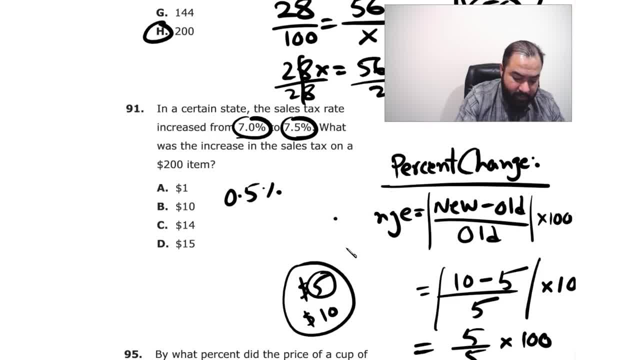 Oh, sorry, Okay, So 0.5%- be extremely careful about it- is 0.005.. Right, Because if you move that decimal two times, then 2-0 is going to be there And times it by. 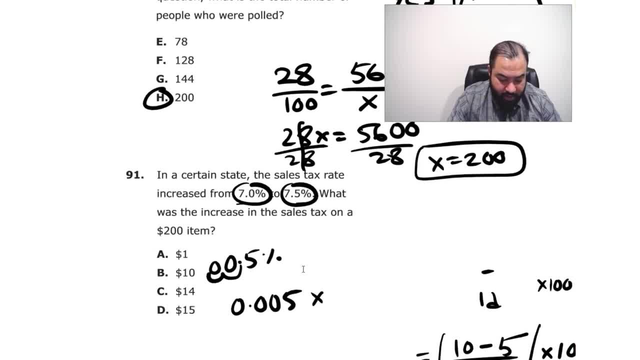 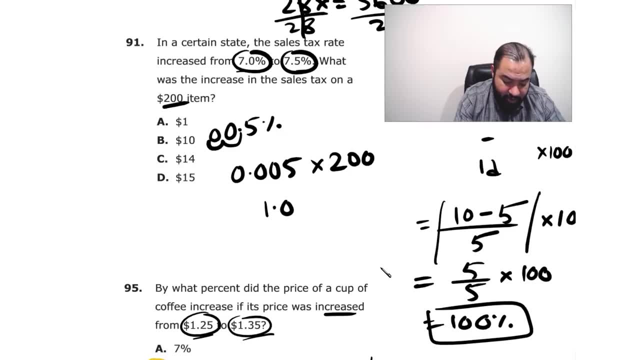 200.. Times it by 200, yeah, Because that's 200, yeah, And then it's 1.0.. If you multiply, you see there are three numbers. Be careful, extremely careful with the multiplication. I believe it's $1.. 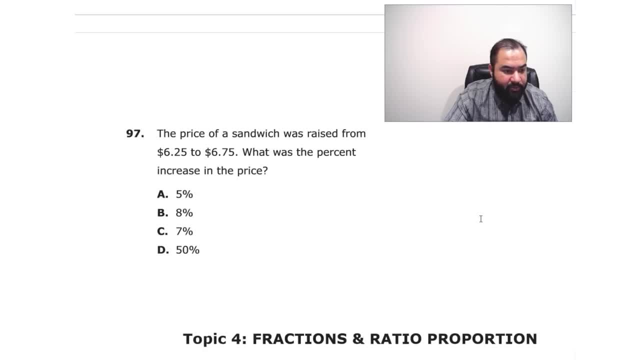 All right, So that's it about percent. There's one more percent change. Well, this is just number to number, so we have to literally use the formula. So percent increase, The new one is the bigger one. Remember there can be percent decrease as well. 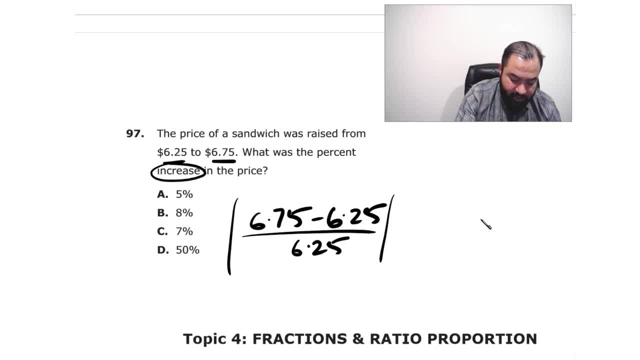 And divide it by 6.25.. Absolute value: times it by 100.. Well, when you just subtract, what do you guys get? 7 minus 2 is 0.5.. 6.25.. Times it by 100.. 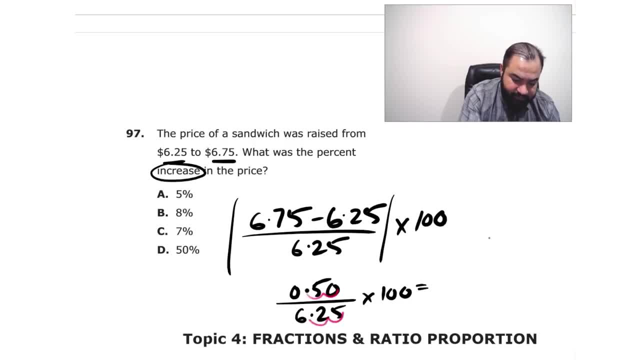 So I can move. as I said. I can move the two decimals to the right. It'll be 50 over 6.25 times 100.. Well, if I times 50 with the 100, that becomes just 5,000.. 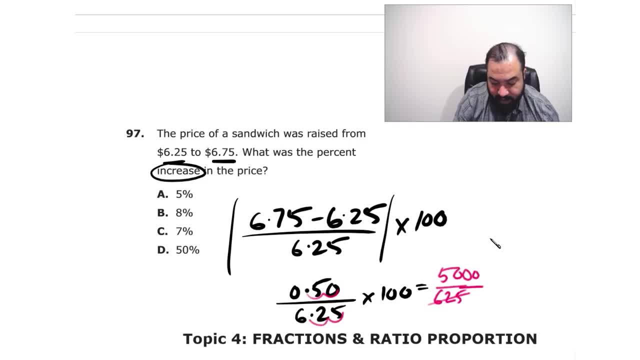 I can simplify it by: 25 goes into 6.25, right 225 times, And 25 goes into 5,000, like 200 times. So I can divide by 25 again, I get 8.. So the answer is 8%. 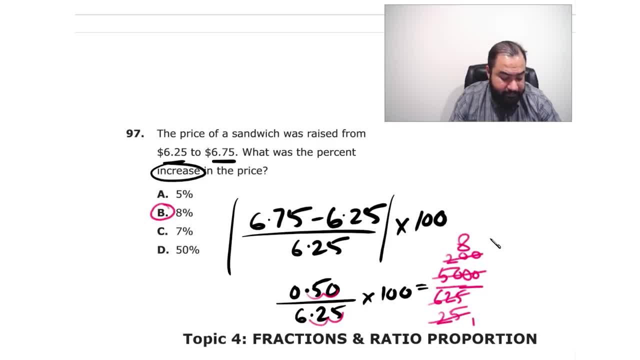 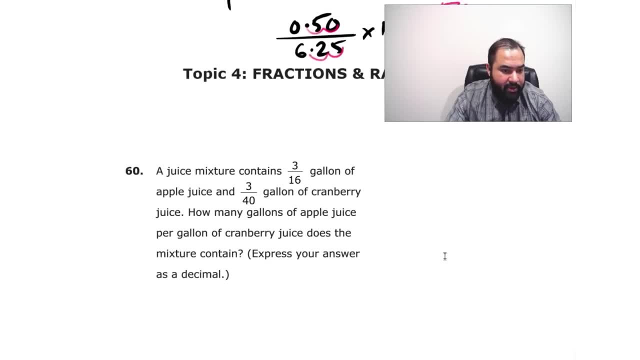 I believe it's 8.. Okay, Yeah, So that's it. You can look at them. I went, I gave you a brief, So this is just to help you during the exam that's coming. So, all right, let's talk about fraction and ratio. proportion: 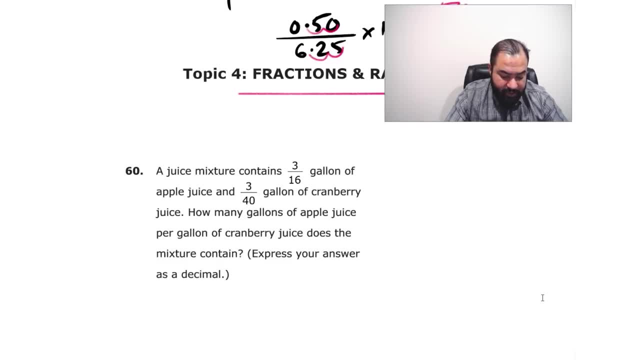 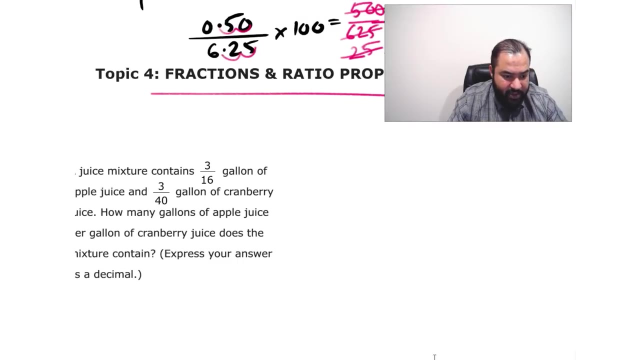 So it says a juice mixture contains 3 over 16 gallons of apple juice, So the apple juice is 316.. And but before I go for this question, I want to show you how fraction simplification works. That will make the life easier. 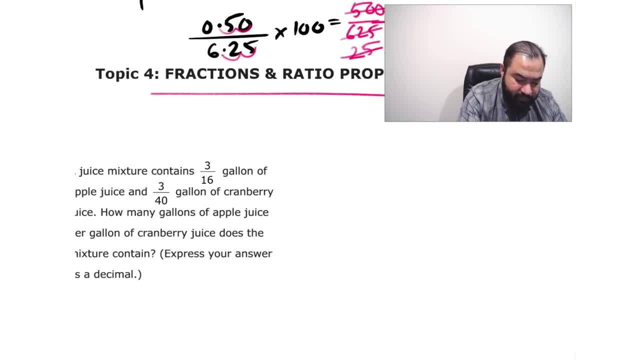 Okay. So how fraction simplification works. Okay. So now you can see. let's say, I give you a question, Let's say 4 out of 20 times it by 40, out of 16 times it by 32 out of 10 times it by 25. 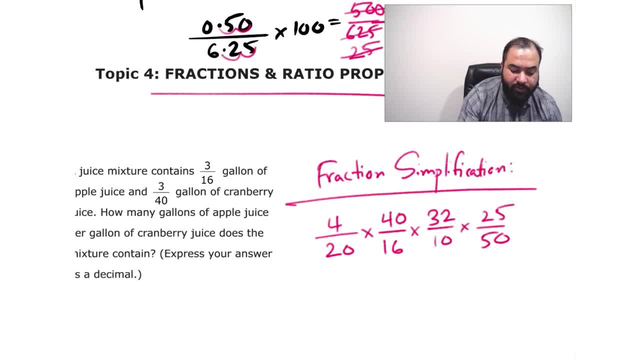 out of 50. So if you were to do it the traditional way, you'll probably multiply all these numbers and then divide by the product of all these numbers. That's a lot of work. So we can do simplification. What we can do is, you see this: the rule for simplification is you can simplify as 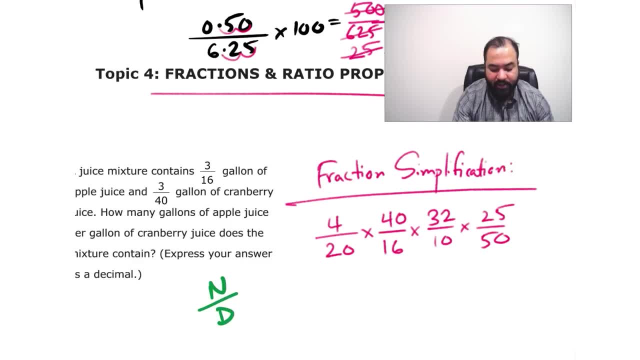 long as one number is the numerator, another denominator, You can simplify with the numerator, with the denominator. What I mean by that is: I can simplify the 4 and 16, right. I can also simplify the 16 with 32, right. 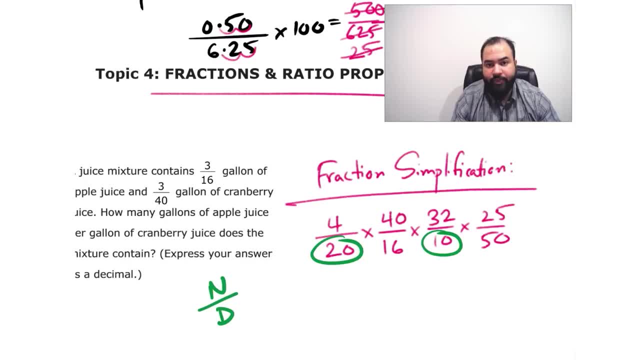 But can I simplify with this 10 and 20? No, because they both are denominators, All right. So can I simplify this: 4 with the 40? No, because they both are numerators. So you see the situation. 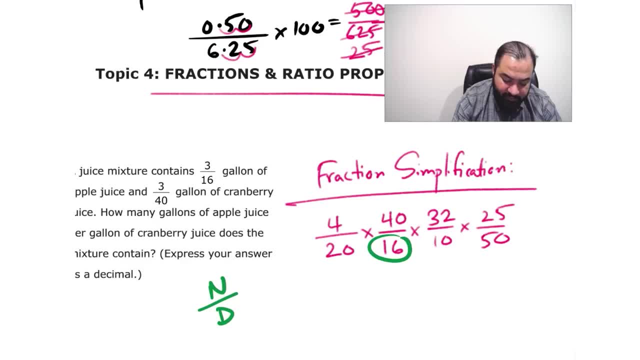 So one has to be denominator, another has to be numerator. So let's simplify the 16 and 32.. Can I divide both of them by 16?? Well, 16 divided by 16 will give me 1.. Just cross it out. write a 1.. 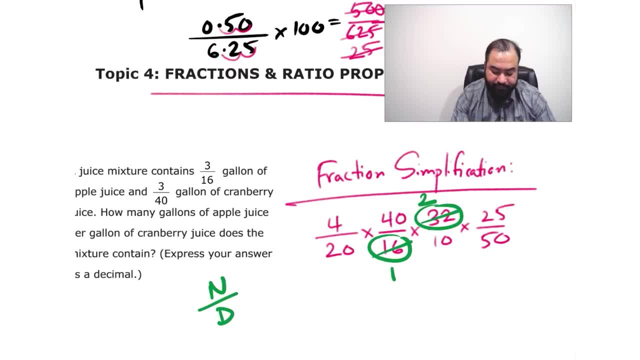 And 32 divided by 16 will give you 2.. Well, can I simplify this? 20 with the 40?? Yes, So I can divide both of them by 20.. So I get a 1 here, a 2 there. 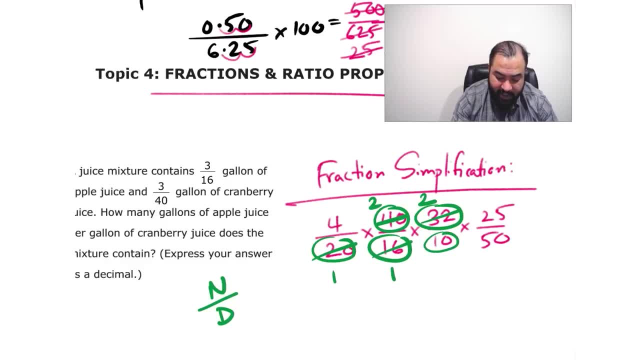 Now can I simplify this: 10 and 50?? No, they both are denominators. Remember, one has to be numerator, another denominator. Can I do 25 and 50?? Yes, we can do it. 25 is a numerator and 50 is a denominator. 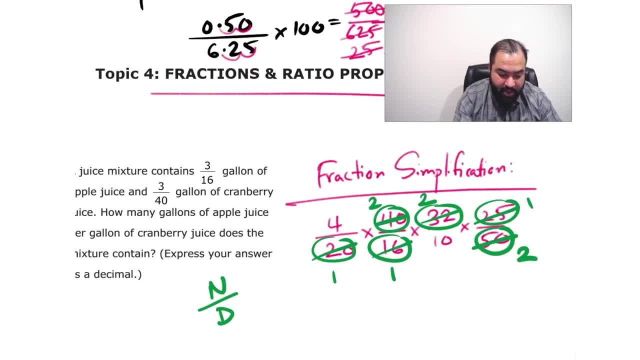 So we can divide both by 25.. We get a 1 and 2.. Now take a look at it. Can I simplify this 2 with that 2?? Yes, numerator and denominator, I can divide both of them by 2.. 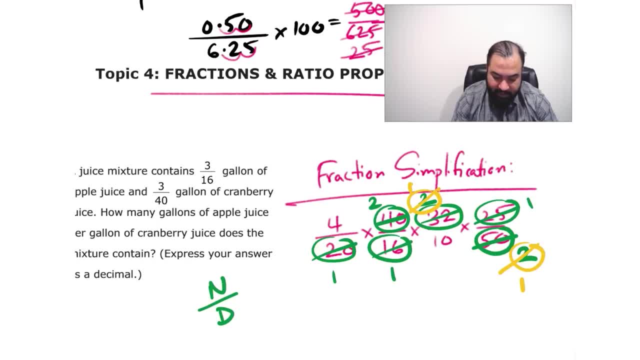 I get a 1, 1.. Can I simplify this 2 with this 10?? Yes, So I get a 1 and this a 5.. Can I simplify anything else? So all I have remaining at the end is this 4 and the 5 in the bottom. 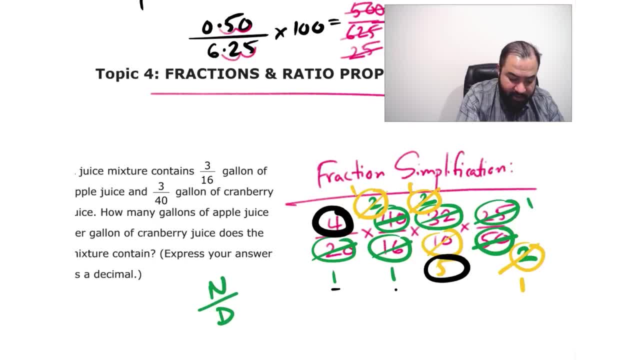 So everything else is just 1, 1.. So the final answer is just 4 over 5.. That's it. So that's how fraction simplification works. Let's do one more fraction simplification. I'm going to give you a simpler one. 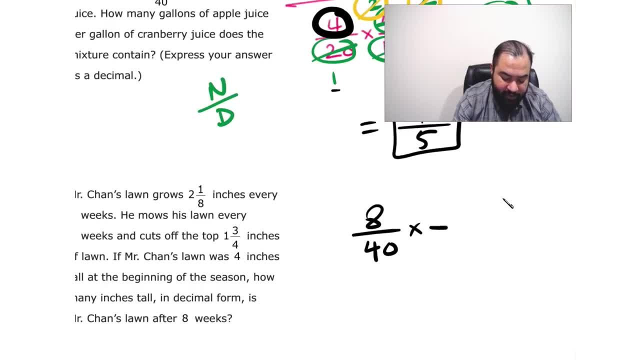 Let's say 8 over 40 times 8 by 80 over 16.. I could easily simplify 8 with the 16. I get a 1 and a 2.. I could easily simplify 40 with the 80. I get 1 and 2.. 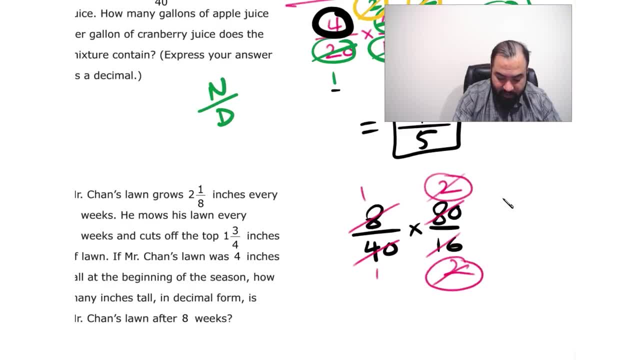 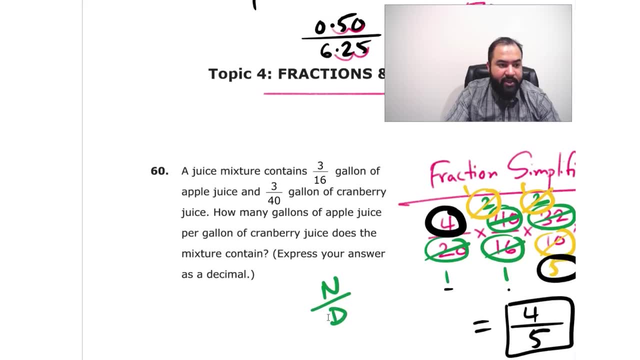 And then I can simplify at the end the 2 with the 2. 1, 1.. So at the end my answer is just 1.. Right, So that's how the simplification works. We're going to use this technique for every question now. 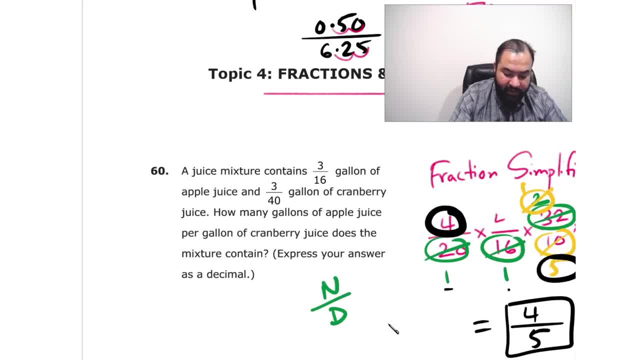 So, and fraction most likely. So simplifying fraction is easy. Well, this only works with fraction multiplication. all right, Okay now. So here let's do the question. They said a juice mixture contains 3 over 16.. 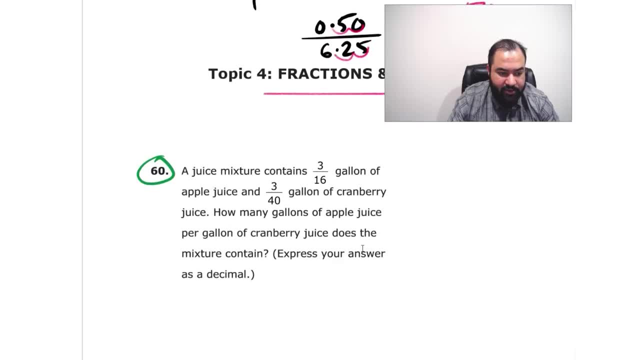 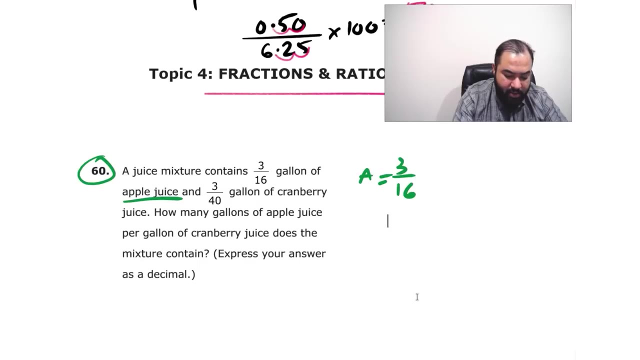 So we're dealing with the fraction and ratio, proportion And ratio proportion together, right, So a juice contains 3, 16th gallon of apple juice. So apple, we have 3 over 16.. All right, That's the apple. 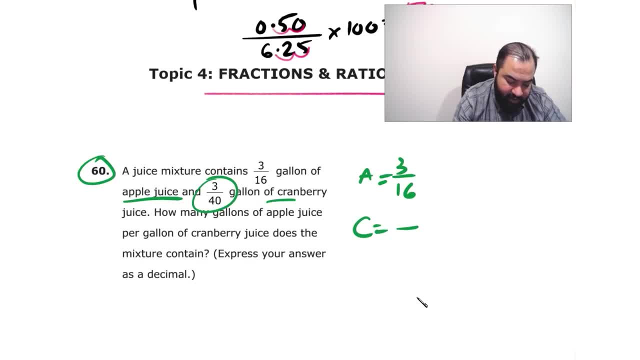 And cranberry we have 3: 40.. Where cranberry is 3, 40 gallons, Now it says how many gallons of apple juice. So apple, I don't know how many gallons of apple juice, But actually you're right. 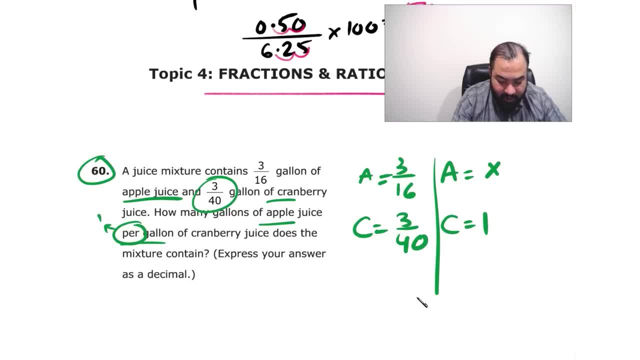 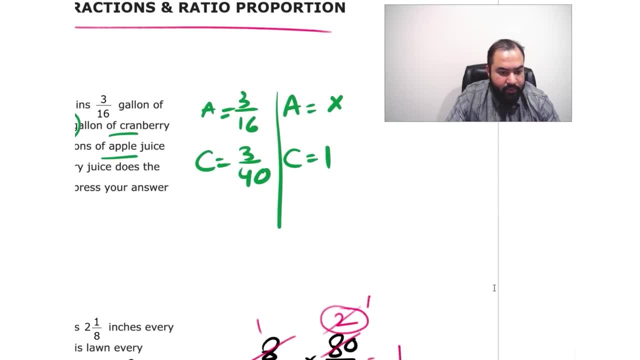 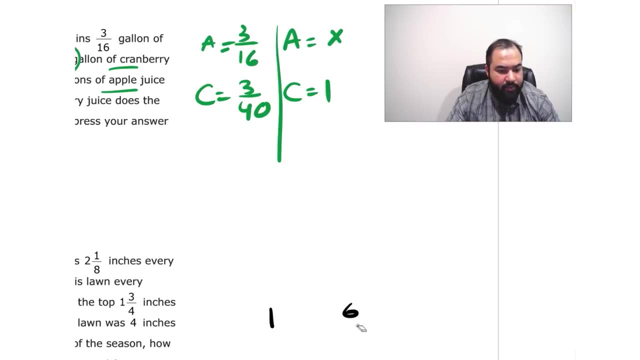 3, 40 gallons. so 1 gallon of cranberry. How many gallons? No, How many gallons? Ah, O, O. One gallon, One gallon of거야, One gallon, right, That's not true. 3 over 40 and here x over 1. so x over 1 is just X, you know. so I just have to. 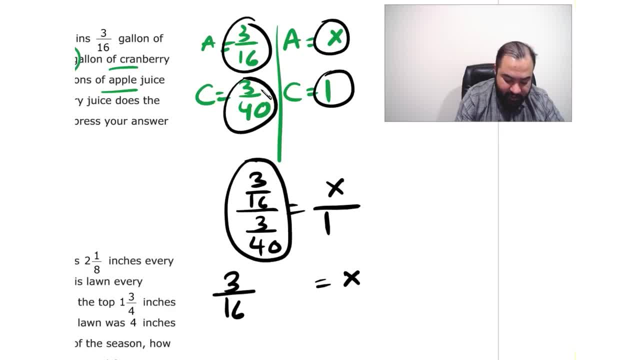 divide these two. you know keep change flip. so 3 over 16 times 40 over 3. now, remember I showed you how to simplify. now can I simplify this 3 with this 3, like, divide both of them by 3. yes, I get a 1 and a 1. can I simplify 16 with 40? I? 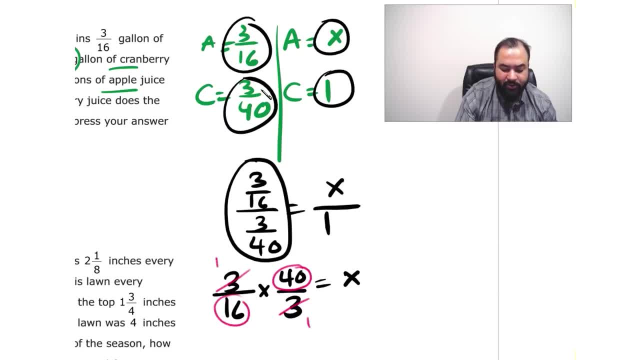 could simplify by 2 or I could do by 8. so 16 divided by 8 is 2,, 40 divided by 8 is 5. so it's just 5 over 2. so 5 over 2 and that's X right. so 5 over 2 is just 2.5. 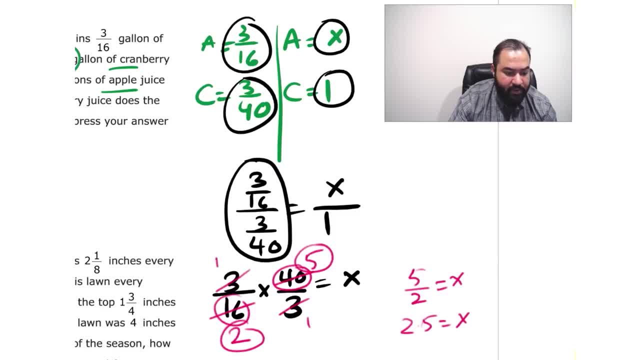 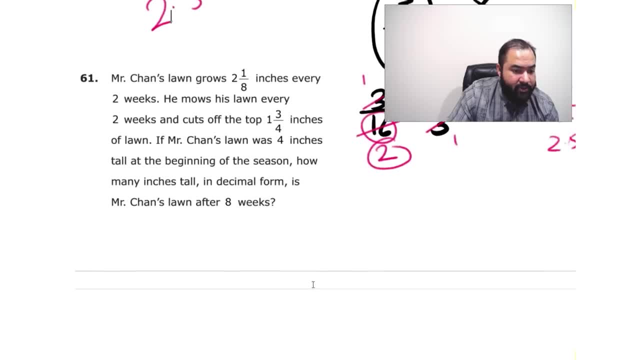 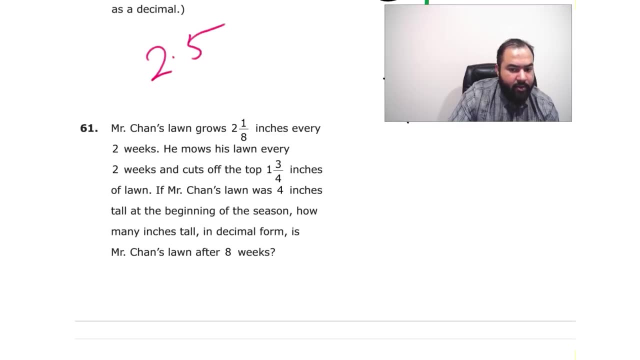 that's a simple proportion. let's do another question. this one is a very interesting one. Alright, so Mr Chan's lawn grows one and two and one-eighth inches every day, okay, Every two weeks, sorry. So two and one-eighth in every two weeks it grows. 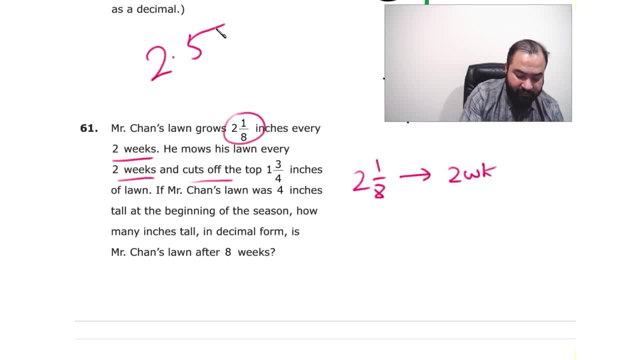 He mows his lawn every two weeks and cuts off one and three-fourth. So he cuts off means he minus one and three-fourth, so every two weeks. So at the end of two weeks let's see how much it grows. 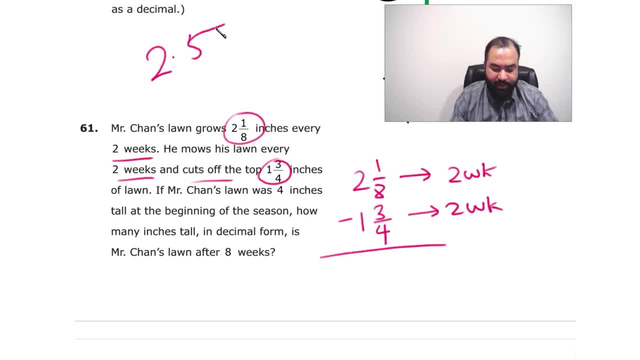 So it grows by two and one-eighth, but after the cutting let's see how much it remains. We subtract, So two and one-eighth means like eight times two, sixteen, that's seventeen over eight minus, that's four times one. four plus three, what 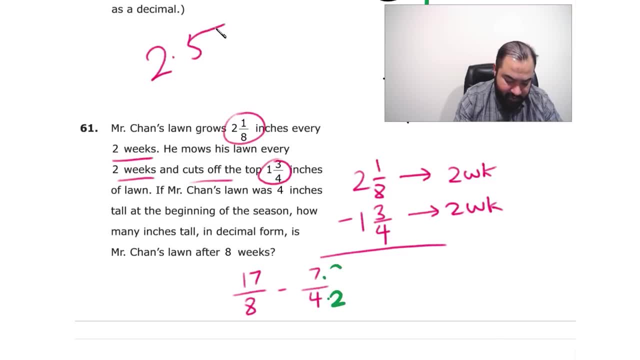 Seven over four. We're going to make the denominator the same, so times it by two two. So what do we get? That's a seventeen minus that's a fourteen. So that's seventeen minus fourteen is a three over eight. 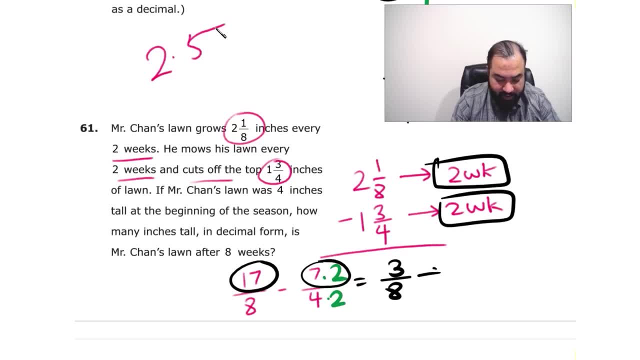 So that happens every after two weeks, right, Two weeks, two weeks later. So, after growing and cutting, this is what remains. three-eighth every two weeks Now it says. if Mr Chan's lawn was four inches tall at the beginning of the season at the 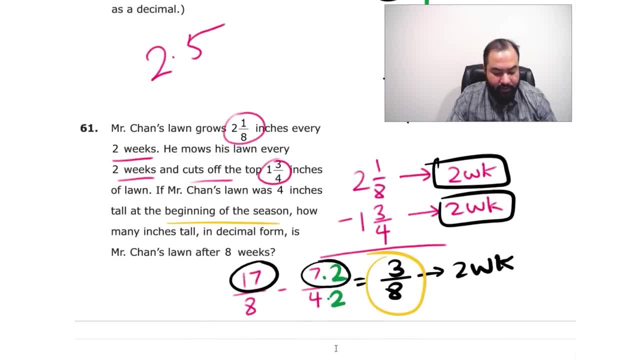 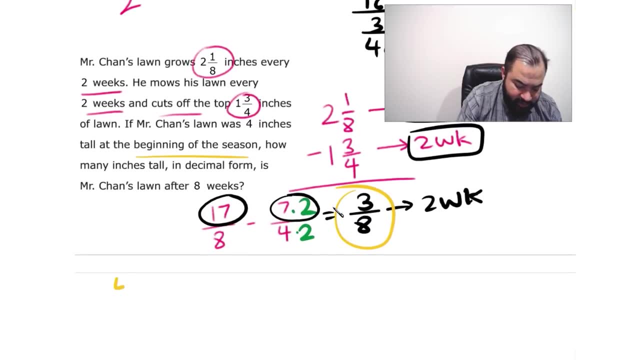 beginning of the season it was already what? Four inches tall, right? Okay, So we can move it a little bit. all right, let's move it this way. all right, it was already four inches tall, right? So they said how many inches tall it will become after eight weeks. 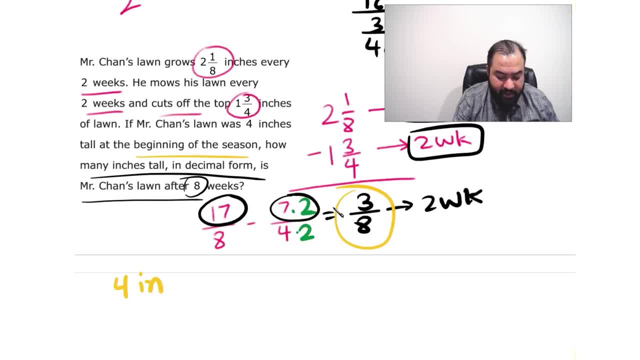 Well, we know that every two weeks later is three-eighth. then four weeks later is another three-eighth, and then another three-eighth, six weeks later, eight weeks later, another three-eighth. So four times four of these, right. 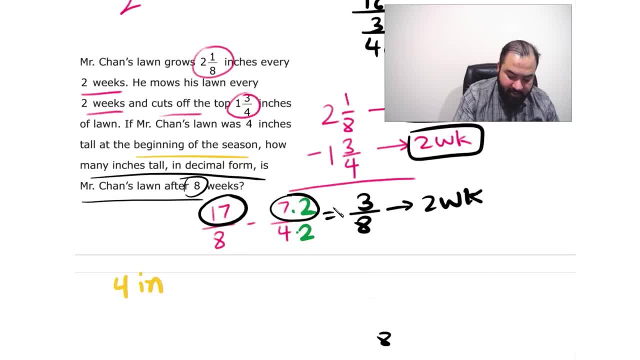 So I can just multiply three-eighth by four, Right? So three-eighth times eight by four over one, so that's twelve over eight. that simplifies to what guys Divided by four both of them, so we get a three over two. that's one point five. 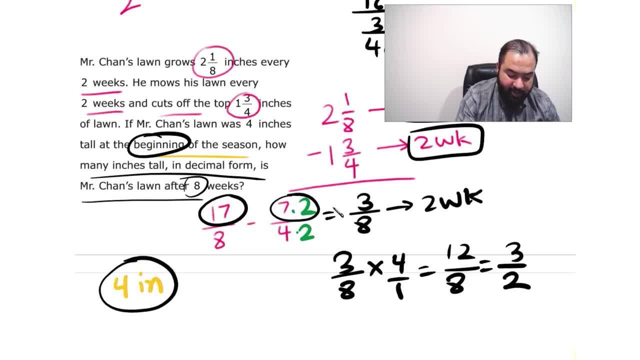 So it was already four inches from the beginning, remember, and then three over two, it increased after eight weeks and that's one point five. so that's five point five. Now the question is why I multiplied by four, Even though it was eight weeks, because, remember, we're dealing with every two weeks. 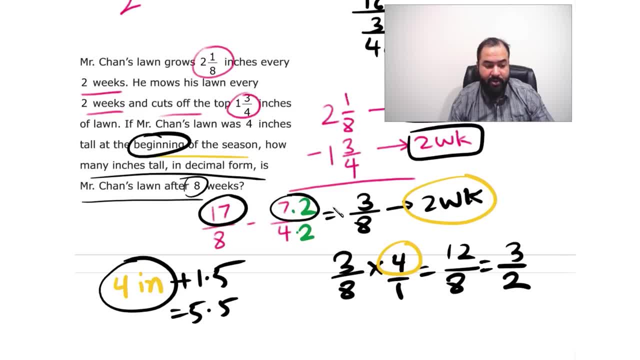 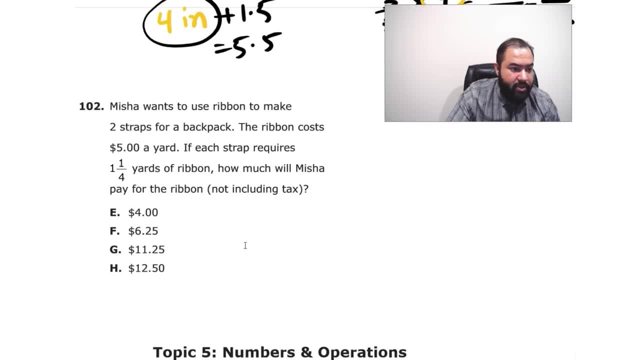 So there are like four periods of two weeks on eight weeks, remember that. So total five point five. Another one: Misha wants to use a ribbon to make two straps of a backpack. all right, So the ribbon costs five dollars a year. 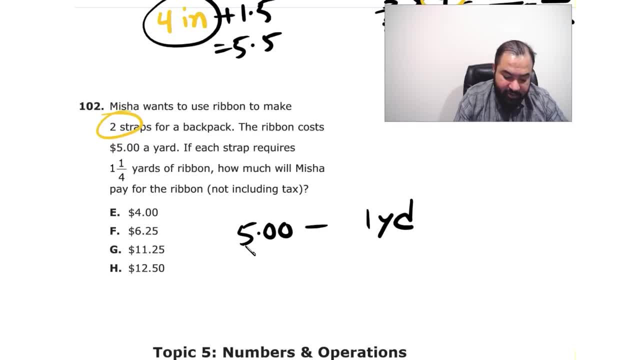 Five dollars a year, Five dollars for one year. So if each strap requires one and one-fourth year, well, five dollars for one year. so for one and one-fourth year it will be one and one-fourth times five. So that's four times one. it's like five over four times five, right. 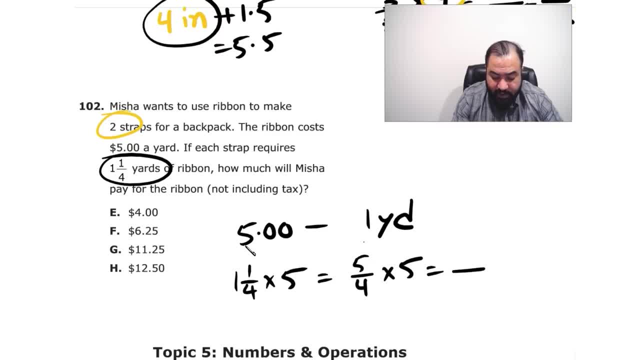 Isn't it? Yeah, five over four times five, so that's five over one. so twenty-five over four, That's what. Six point two. five, That's for one strap. so remember that each strap takes one and one-fourth year, but she's. 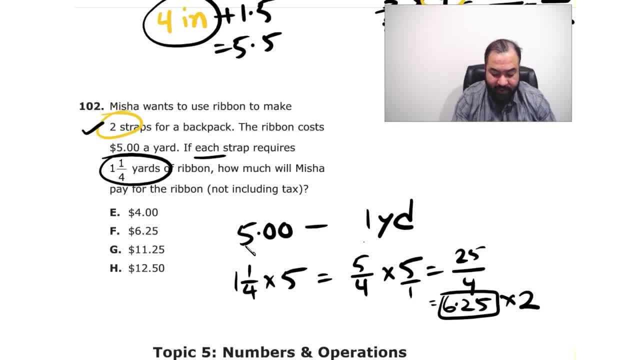 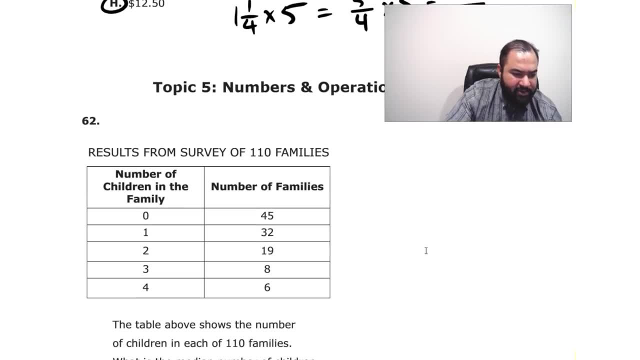 making two straps. so I'm going to times it by two to see, because this is the cost of one. you times it by two, so it's twelve-fifty for like the two straps. Simple word problems, guys, read and that's going to be fine. 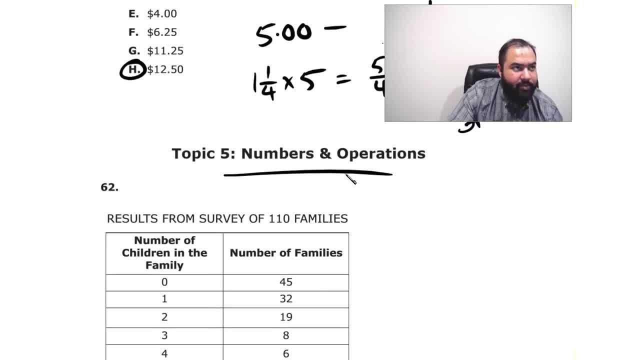 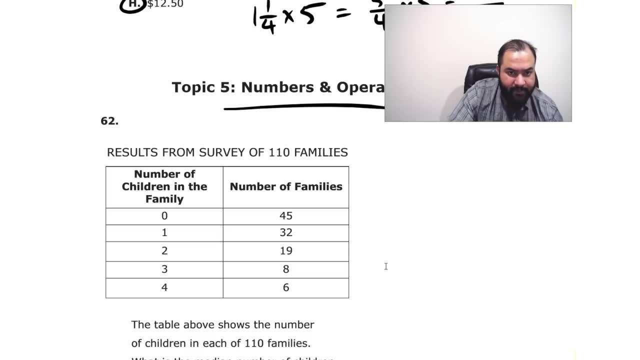 Now there are, like these, numbers and operation questions. you have to be careful about these. okay, Now results from survey of one in ten families. number of children in the family. alright, so the number of families, the number of children in the family. so forty-five families has. 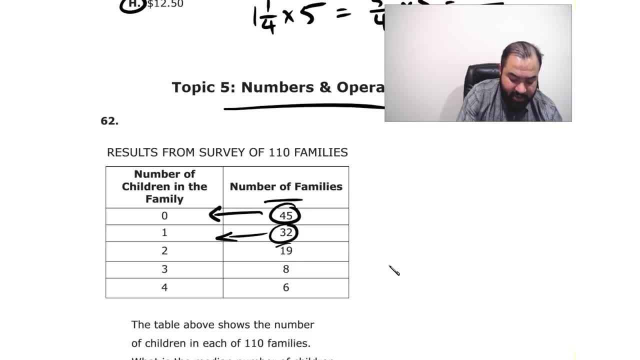 zero children. thirty-two has one child, nineteen have like two children each. so that's the table he's talking about. Oh, sorry, Now what is the question asking? they said, okay, find the median of one hundred and ten. 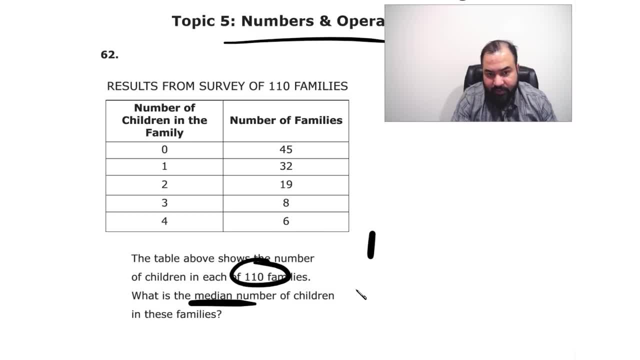 families. Well, one hundred and ten families. the median means you have to put them in order. so one hundred and ten families. so you divide one hundred and ten by two, so middle would be like the fifty-fifth one, that's the middle of it. 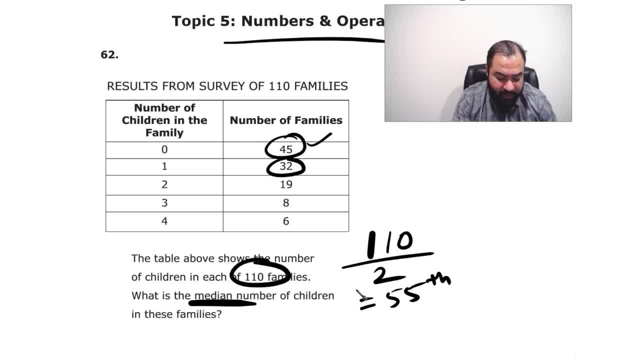 So forty-five plus thirty-two is the first. forty-five will be zeroes, right? So it's not going to fall in the median, And when the another thirty-two comes, they'll add up. They'll add up to like seventy-seven, so the fifty-five falls in somewhere here. so 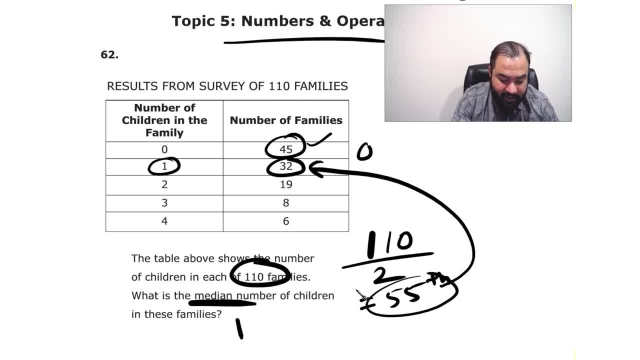 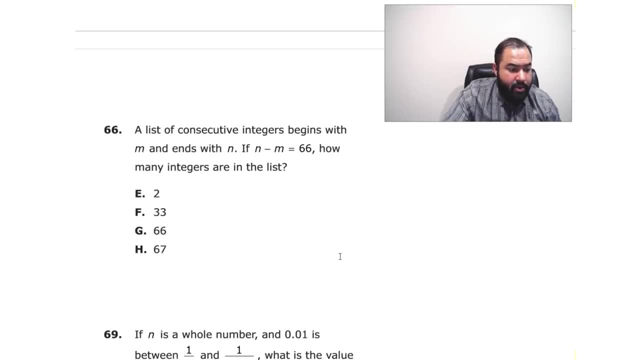 the median has to be one, okay, because if you list it like forty-five zeroes and then thirty-two ones, and then nineteen twos, and then you will see that the fifty-fifth one is falling in one. so one is the median. 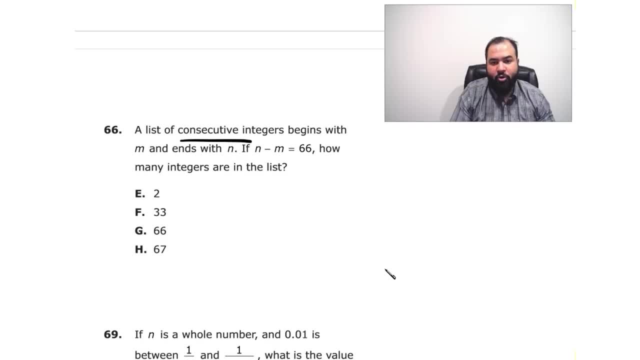 Number sixty-six. it says a list of consecutive consecutive means in order like you know, one, two, three, four, five, six, like that, Like you know, two, three, four, or like seven, eight, nine, these are consecutive. 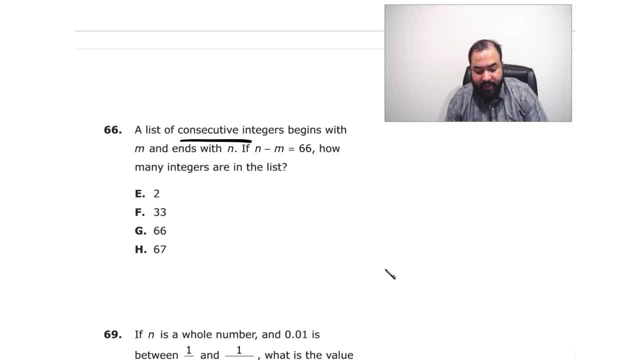 Now it says a list of consecutive integers. begin with m. it's beginning with m and then it's ending with n. So how many integers are there if n minus m is sixty-six? I forgot about this- n minus n? m- for like a moment. 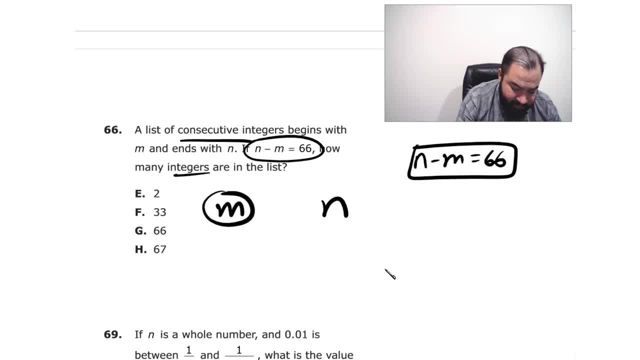 So it says: this is what. it starts with m, this is the beginning, and ending with n. So how many integers are there? So let's think about it. let's say, if I ask from five to eight how many integers are? 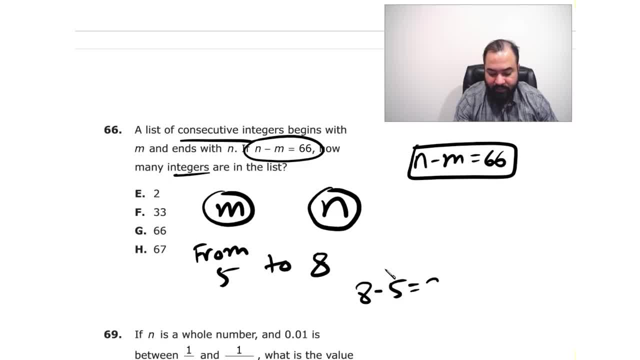 there You can be like: okay, just eight minus five, three. but that's not true. If you list it five to eight- five, six, seven, eight- there are actually four integers. So after subtracting you have to add one with it to find how many integers are there. 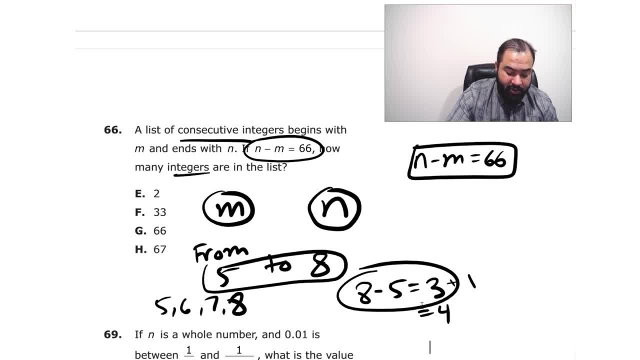 Okay, That's the rules. So let me explain the rule again. So if you want to find how many integers are there, you subtract, you do the last one minus the first one and then plus a one. That's how you find how many integers are there. 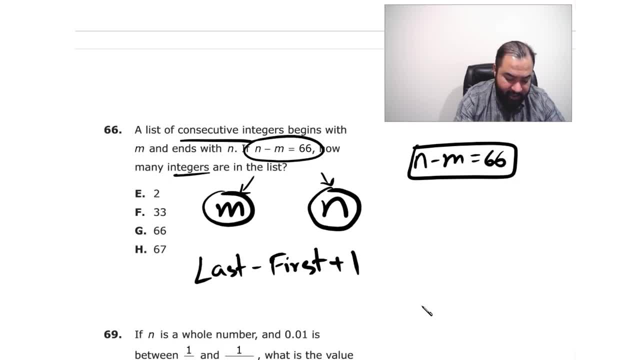 So now look at it Here. my last one is n, so minus m. so you have to do n minus m and then plus one. And the good news is I already told you what it is. I already told you what n minus m is, that's 66, just do plus one with it: 67, that's it. 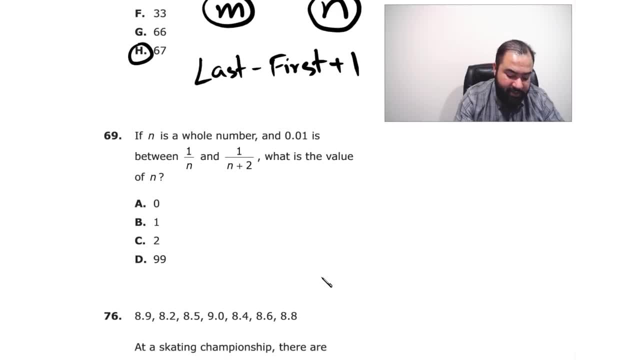 Question 69,. it says if n is a whole number. whole number means all. remember zero is a whole number. zero one, two, three, all positive numbers. don't be shocked, knowing zero is a whole number. So if n is a whole number and 0.01 is between one over n and one over n plus two, what is? 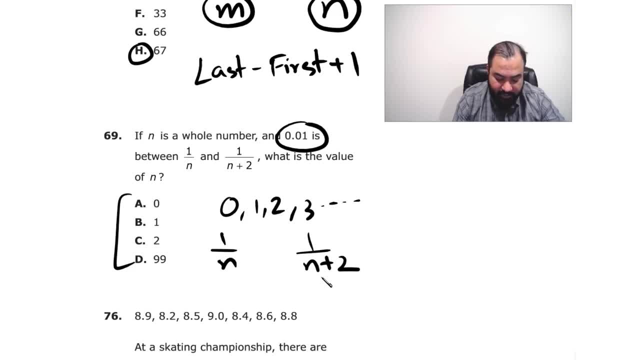 the value of n. So you can do trial and error, check out the each options. So first of all, zero is not going to work if n is zero, so one over zero. zero cannot be in the denominator, so it's not zero. 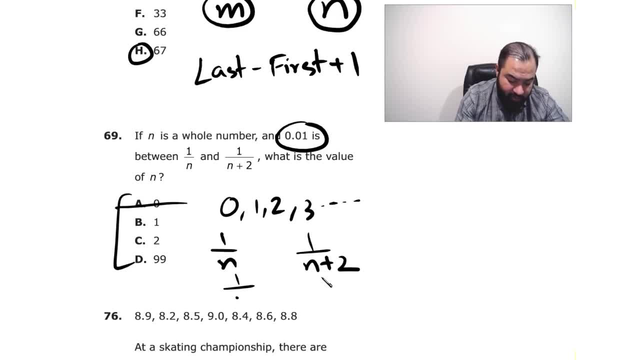 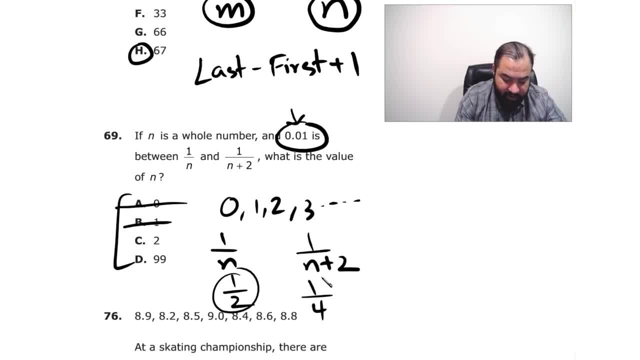 So it's going to be one over two. what do I get? So we'll get one over two and one over two, plus two, four, So that's between 0.5 and that's 0.25.. So this number is very small, it's 0.001, so it's not even there. so it's d. 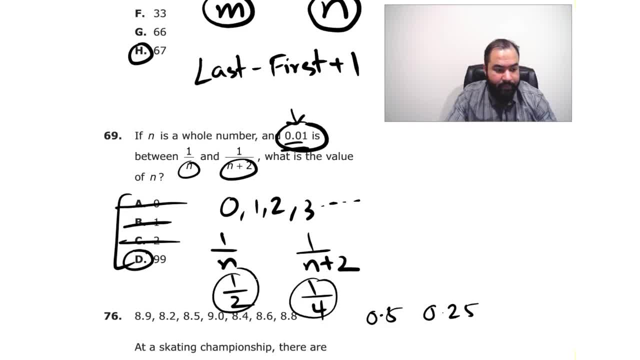 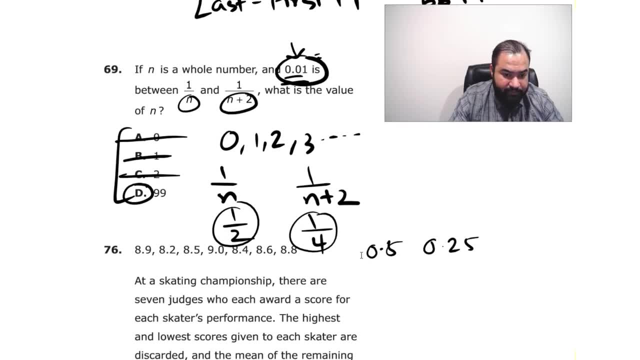 Also, it's common sense that the denominator has to be big for this number to be small, Because this number is what Like? another simpler way is what? 0.01 is one-third one over a hundred, right, So that's simple. closer to ninety-nine. 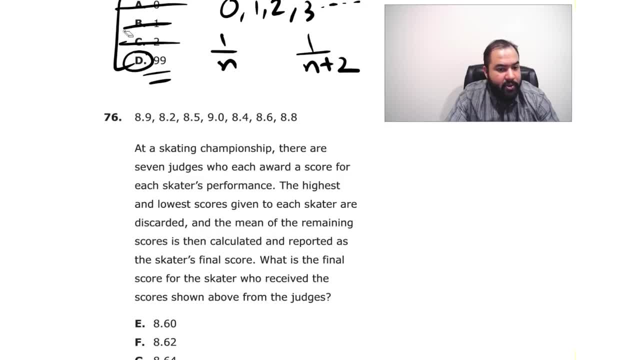 These are work problems, logic you're going to use. Alright, now here one more. It says they gave you a bunch of numbers and then it says at a skating championship, there are seven judges who each award a score for each skater's performance. 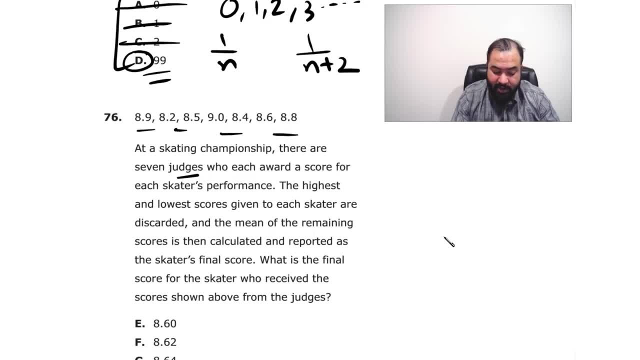 The highest and the lowest scores given to each skater are discarded. Discarded means you remove them. So what is the highest Like nine, remove it, And the lowest is eight point two. remove it, And after that the mean means you add them. divide by the numbers. 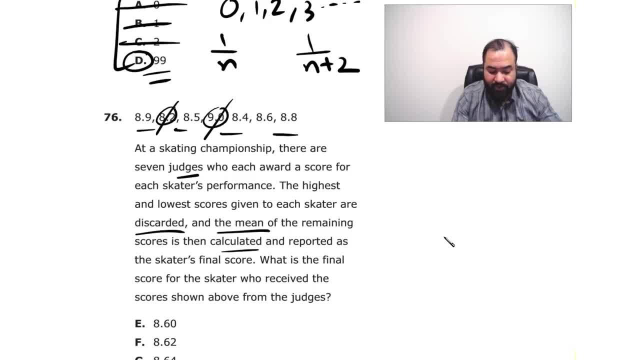 The mean of the remaining scores is calculated and reported to the skater's final score. So what is the final score? So we just have to find the mean of it. So you do eight point nine plus eight point five plus eight point four plus eight point six plus eight point eight. 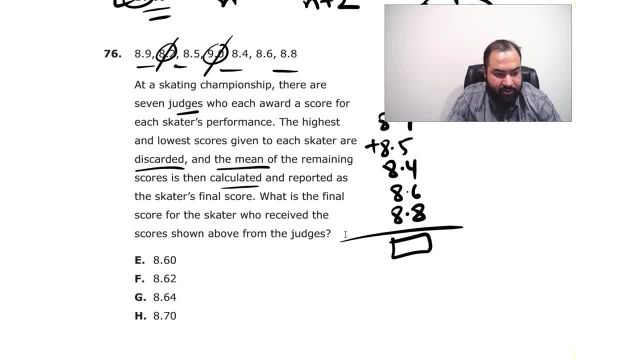 Whatever you get, you, divide by five and that should give you the answer. I'm not doing it now. it's going to take a long time. now You just do it. So let's do the next one. Let x be an odd number. 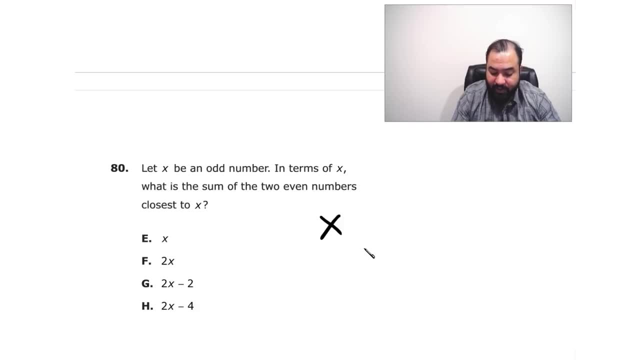 So let's say x is an odd number. So what is the sum of the two even numbers closest to it? Or pick a number. let's say five is an odd number. The next closest even is six and the one four. that's less than it. So this is a two. 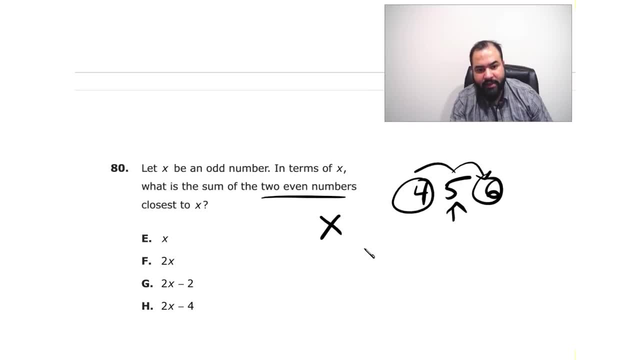 So with the odd number we have to plus one to get the next even And minus one to get the closest even. that's less than it. So x is odd. the next odd even will be x plus one And the even that was before it was x minus one. 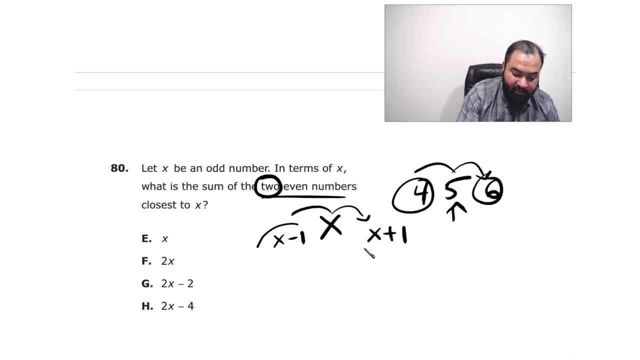 And they said: what is the sum of the two even numbers? So sum of just these two, this one, this one and this one. So if we just add, what do we get? So x minus one plus x plus one. So that's here negative one and positive one, just cancel out. 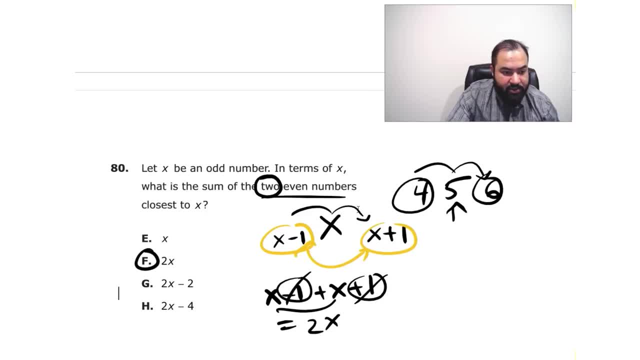 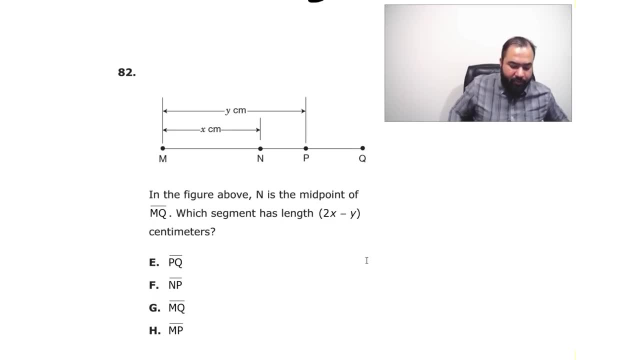 So that's here, negative one and positive one. just cancel out. It's just two x Simple questions, guys. There's another one. it says in the figure above n is the midpoint of m cube, So n is the middle point so of the whole thing. 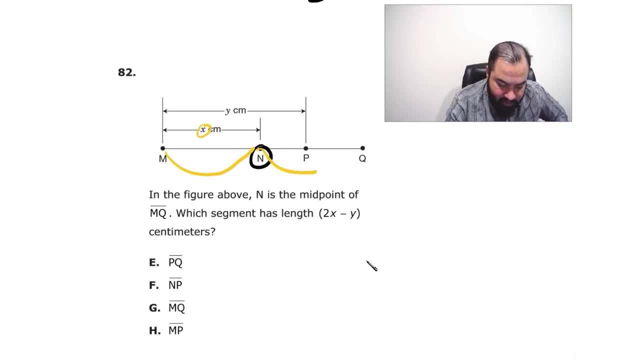 So from here to here is x, we can see. So here to here will be x also, because that's the middle point. So here to here is x also. So now they said which segment is two x minus y? Well, two x is the whole thing. we know. x and x is two x. 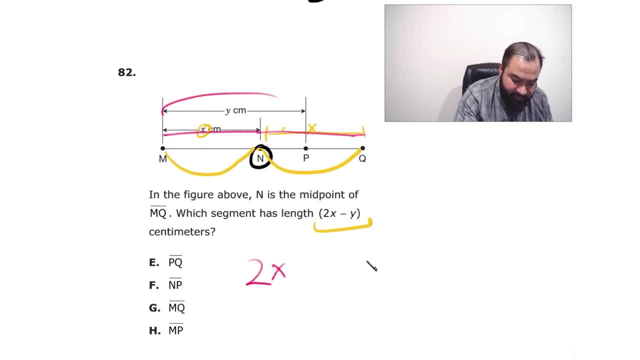 That's the whole thing From two x. if you subtract the y, two x is the whole thing. take out this part which is from here to here is y, So all that remains is p cube. You see that? Let me show you again. 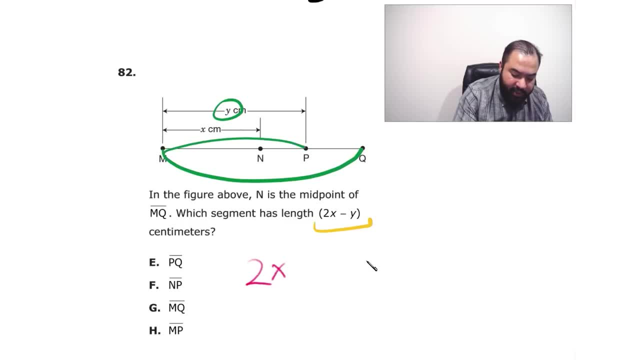 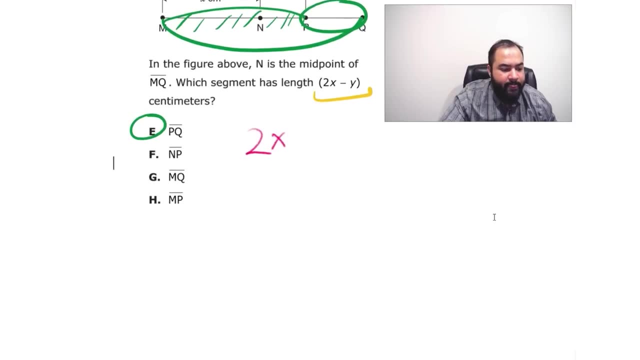 Two x is the whole thing and y is from here to here. So if you remove this part from two x, all what remains is p and y, PQ. That's why answer is PQ. This is just a simple absolute value question. So this: 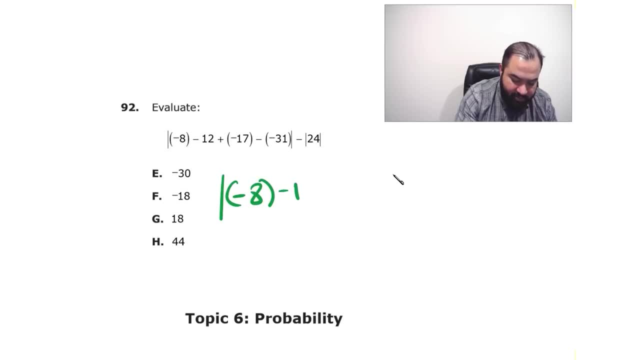 is negative 8 minus 12. Then this is a plus and a minus, so it becomes minus 17. Minus and a minus become plus 31. And minus 24. So negative 8,, negative 12 is negative 20.. 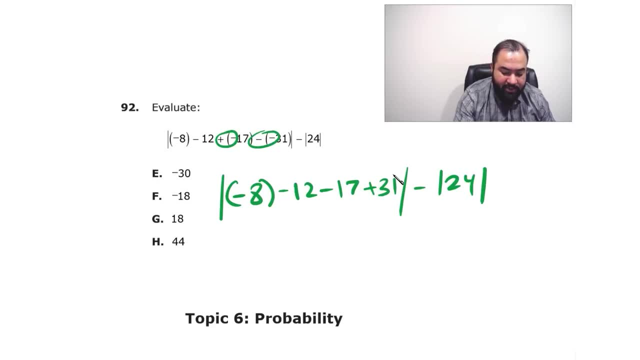 Negative 20, negative 17,. negative 37 plus 31 is negative 6 for the absolute value And there's a minus and another absolute value, 24.. Remember, this minus has nothing to do with the absolute values Because, remember, this is inside the absolute value, the negative. 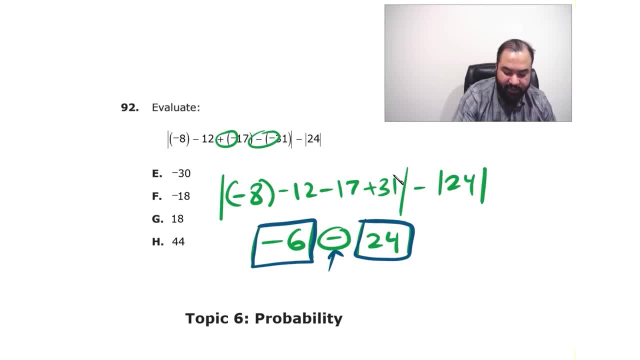 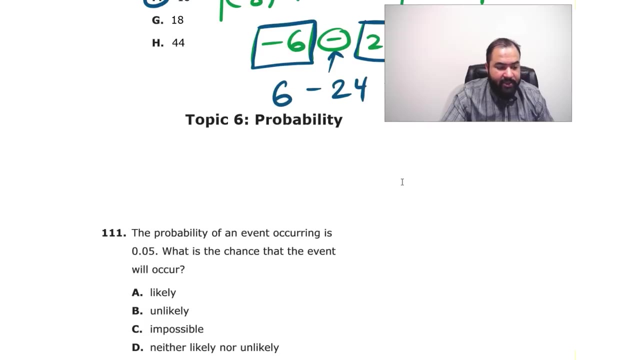 6 and 24, but not the minus. This minus is outside, So this negative 6 will become positive. 6 minus 24 is just positive 24.. And the absolute value makes it positive, So it's negative 18.. Well, the final topic is probability. This is very important. So, first of all, before 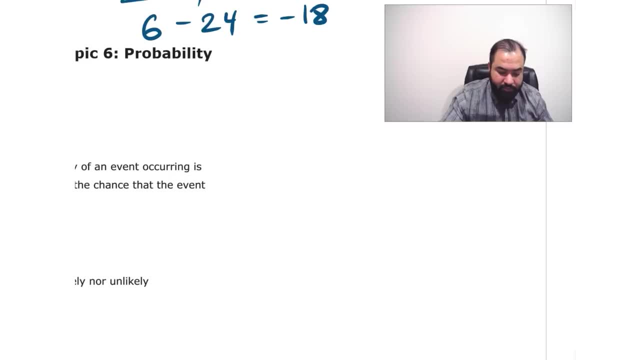 I go for probability. I'm going to give you some background knowledge. Three types of probability you've got to understand. The type 1 just says: let's say you have a box, There are 10 red marbles, 5 white marbles And simply they ask: what is the probability? 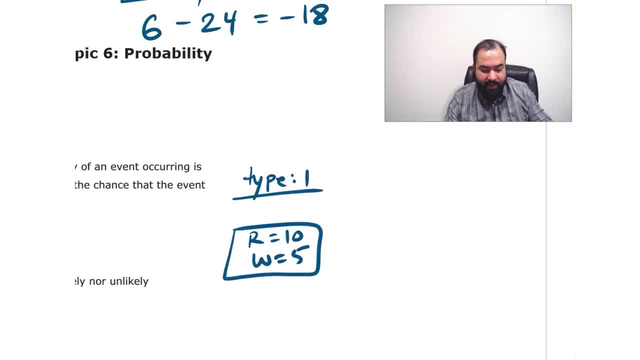 of picking a white. Let's say, if I were to put my hand inside the box And take out a marble, what is the probability that we get one white? How many white guys? One. But the probability means chances, like the chances, right, The probability of picking. 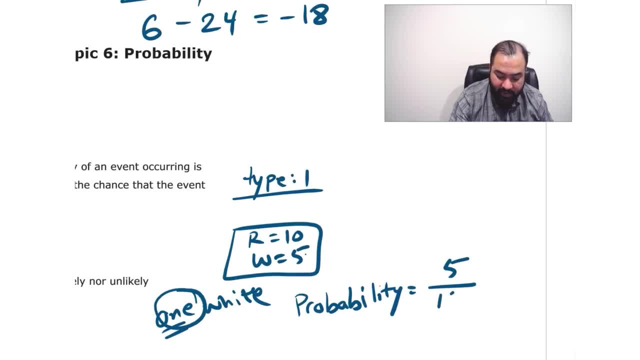 only one white. is what? 5 out of 15.. Because there are 5 white out of total 15, right, But remember, I just picked one white, not all 5.. Then why I put 5 over 15? Because the chances. 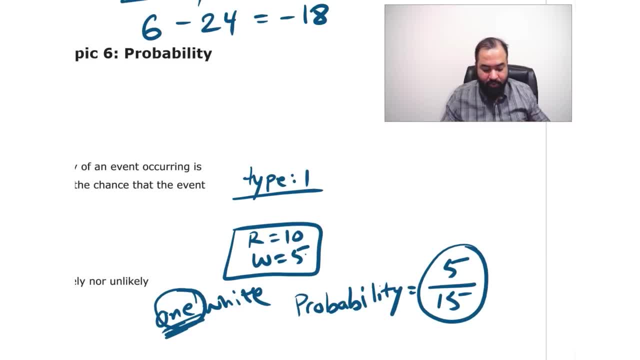 is 5 over 15.. So I only took out one. Probability is 5 out of 15, but I took out only one. Remember this, Excuse me. So that's the first type. So they will give you red and white And they're. 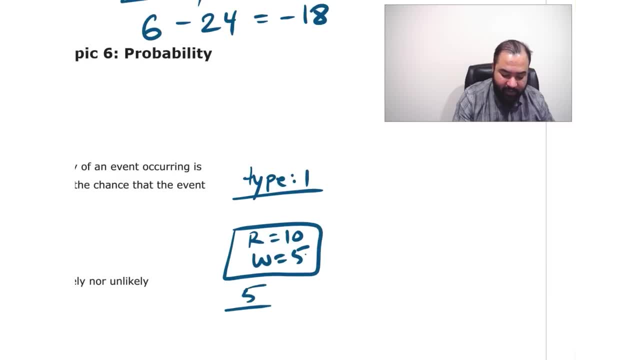 going to ask: OK, what is the probability of picking a white? So it's just 5 out of 15, probability of picking white. That's type 1.. Now type 2, they will give you. let's say, in a box there are total 20 marbles, 20.. 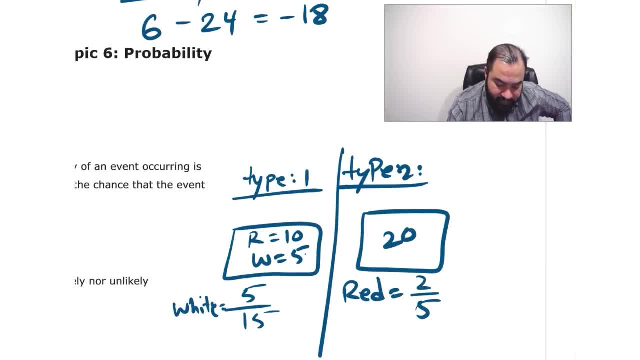 And they will say: red is 2 5ths, Red is what? 2 5ths? So how many red is there? So you just multiply this 2 5ths with the total 20 over 1. That gives you the answer. So remember. 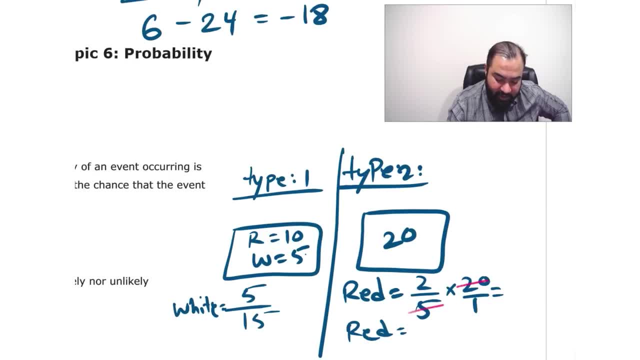 I showed you how to simplify. of course, Simplify 5 with 20,. right, Get a 1 and a 4.. Can I simplify 2 and 4? No, because they are both numerators. So we just multiply these two 4 times 2,. 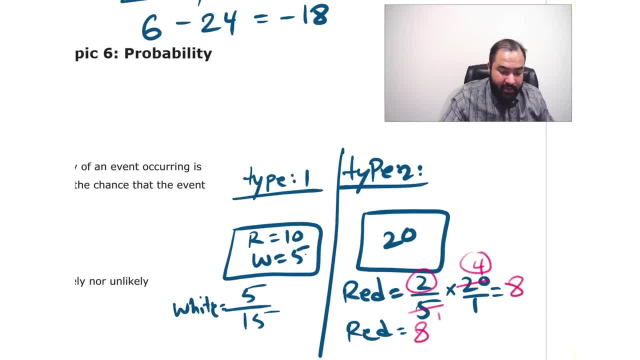 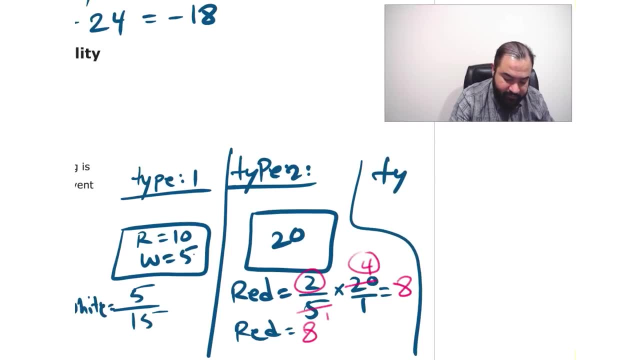 8. So total: 8 reds, 8 reds. So that's another, the second type. The third type, it's pretty simple as well. Type 3 is like 2 events, Like more than 2 events, right, 2 events, 2 events or more. Now you'll be. 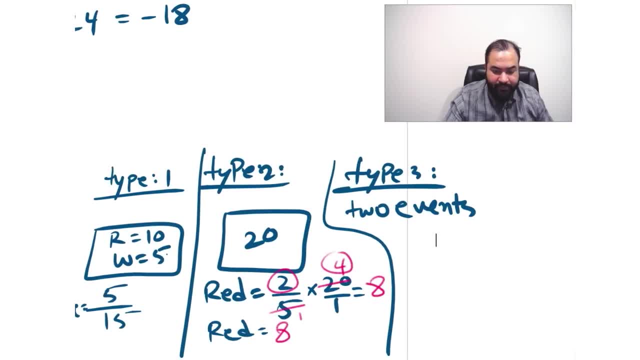 like: what do you mean by 2 events? Let me show you to play more briefly. So it says you have 3 red marbles. Let's make the box bigger, Let's see our big box. So 3 red marbles. 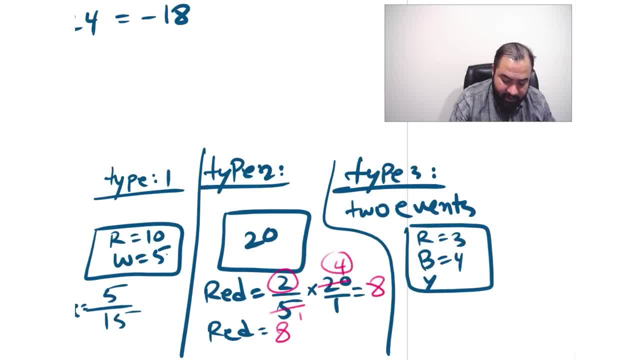 4 black marbles and let's say, 3 yellow, 5 yellow marbles. Now I say that if I were to pick 2 marbles, what is the probability that first I get a red and then I get a blue? 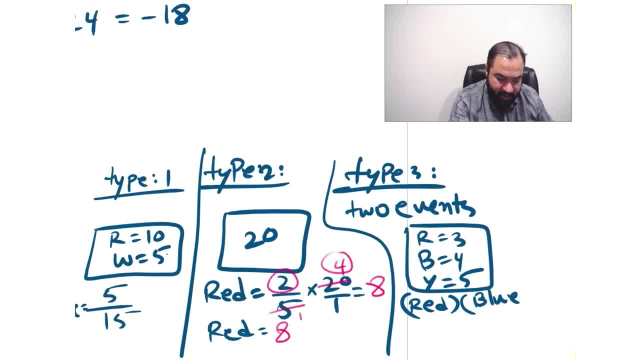 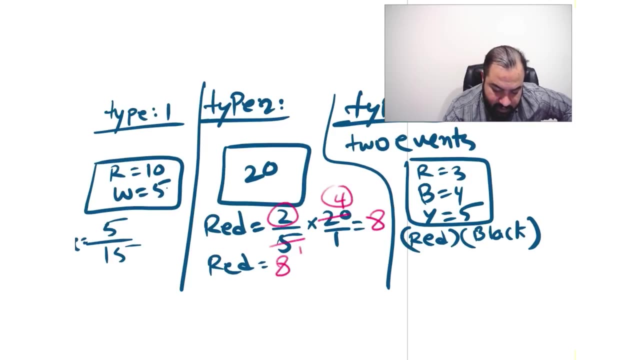 It was blue or black. Okay, Let's say that was black. Yeah, Okay. So 3 red marbles 2. right now, the probability of getting a red first is what three out of? if you add them all, that's a seven plus five twelve. there's the probability of getting red. so now there are two words. you. 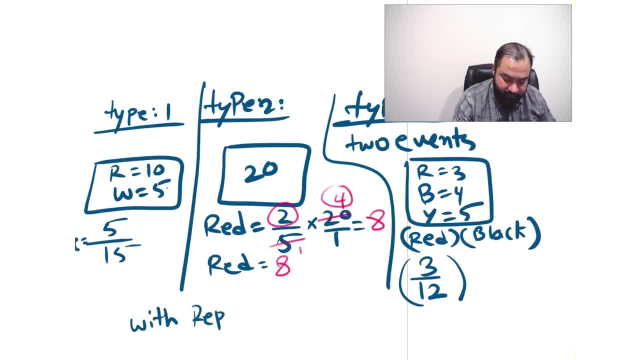 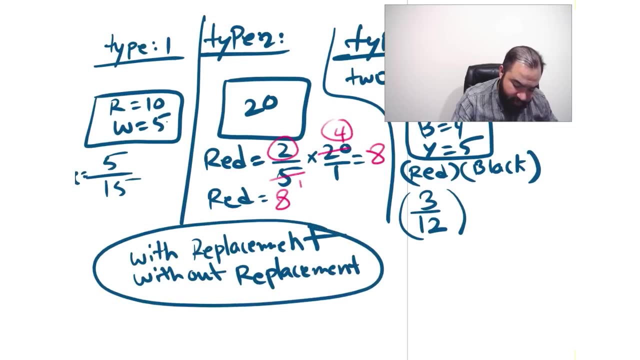 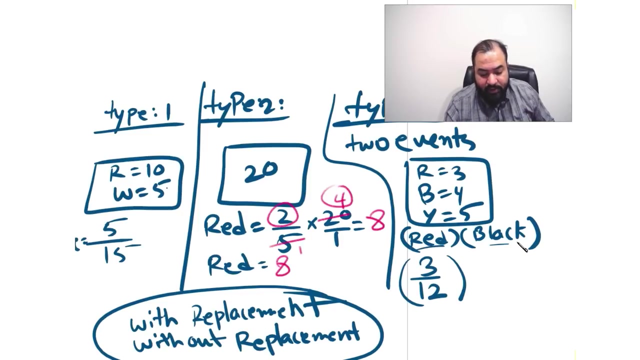 have to understand like with replacement or without replacement. so now the case is like: okay, you took out two marbles like red and black. you want the probability, so when you took out the red first, do you place it back again or you just threw it out. so let's. 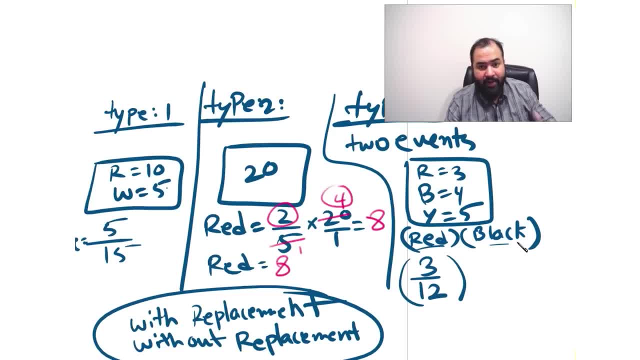 say. I ask a question like: okay, what is the probability of picking a red and black when you pick the red, you didn't replace it back, so without replacement, so you took out a red, only one red you took out, but the probability was three out of twelve, so now you have one. 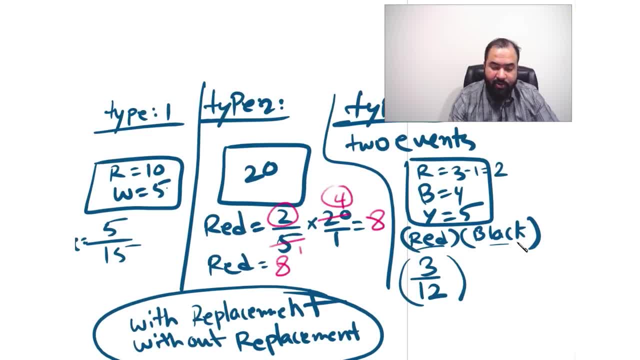 less red. so now you have only two red. now probability of picking a black now is four black out of total is 11. you see the total became one less because you took out a red already. so now you have one less total. now you just multiply them. so if you multiply them you get three times. 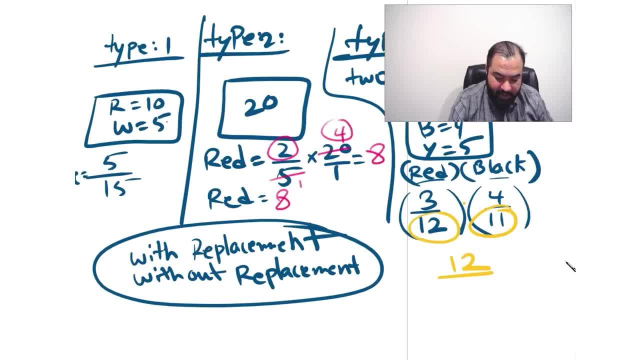 412 and 12 times 11. it could do simplifying. when you multiply, you know simplifying will make it easier. right, because we have four with 12, we get a three, one. right, we can simplify these three with that three numerator denominator, so it's just one over eleven, you get it two events, so we're. 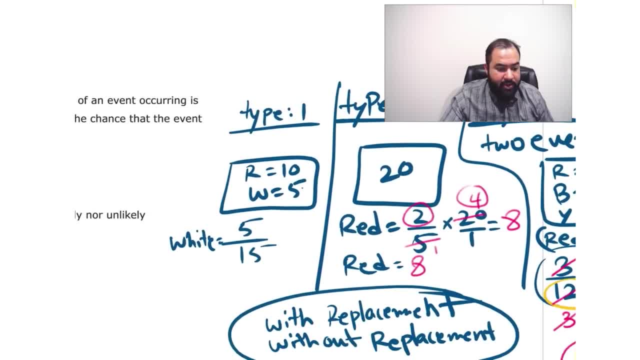 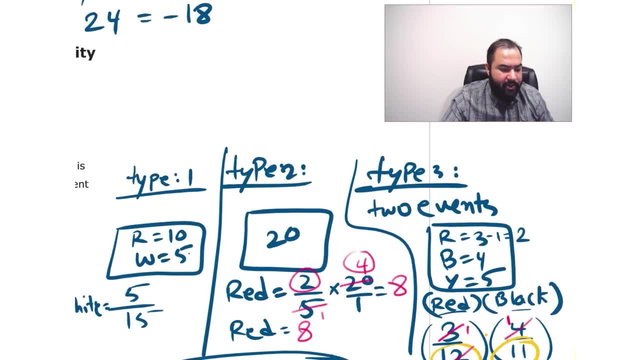 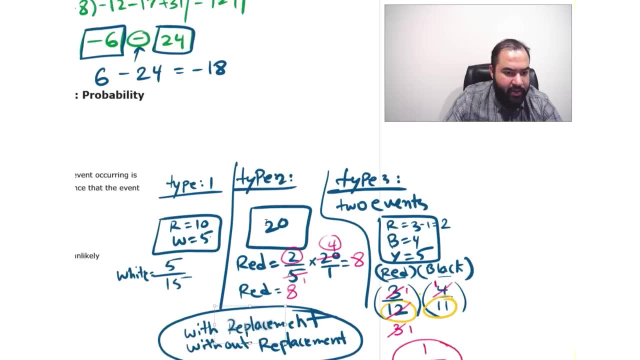 going to practice some questions so you'll understand the three types, all right. so let's take a look at the types again. type one is just simple: picking probability, right. all right, let's practice them, we'll get better. let's make it simple, easy, all right. these are 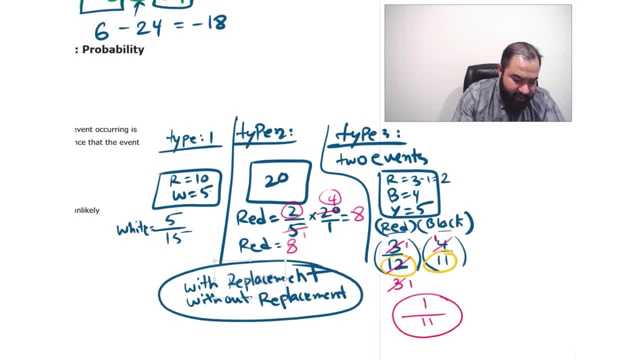 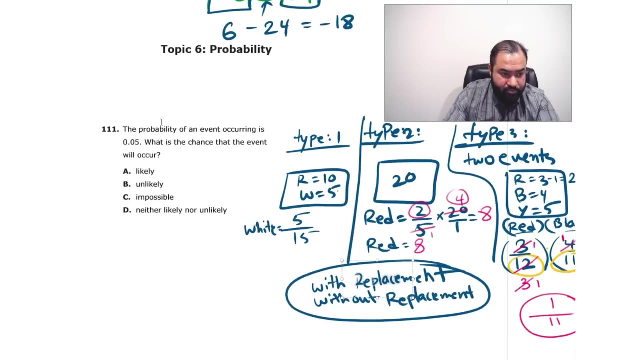 the three types. so type one: simply finding probability. that probably probably understood. type two is just: you know the fraction, you multiply to see how many red. type three is just the two events and what is the probability of picking red and black and they just multiply. we're going to practice them more, like this question. let's say here: first the type three. 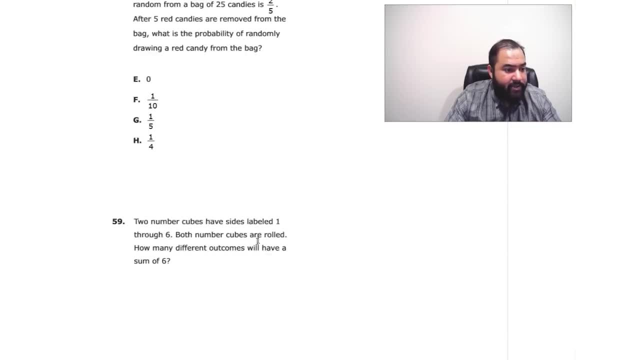 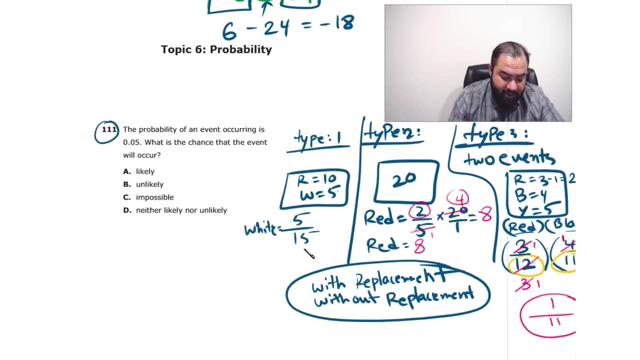 ones. let's say we're going to do that first. okay, let's go in order. so let's do 111. the probability of an event occurring is 0.05. what is the chances that the event will occur? 0.05 is like 5%, which. 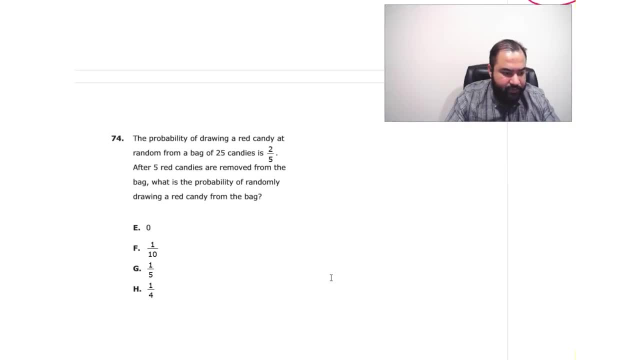 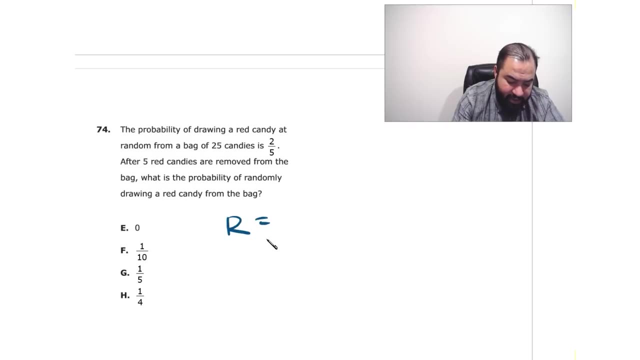 is very unlikely, very small, not impossible. unlikely. then the second: here it says that the probability of drawing a red candy and a random bag is 25, or bag of 25, sorry. so the probability of there is a bag, so the probability of drawing a red candy at random from a bag of 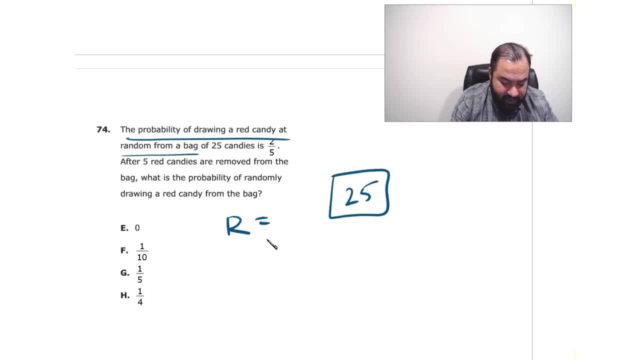 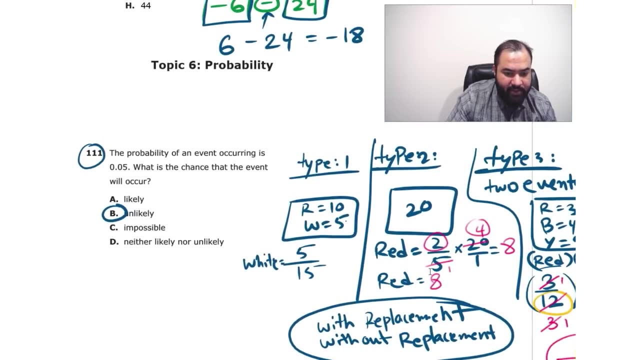 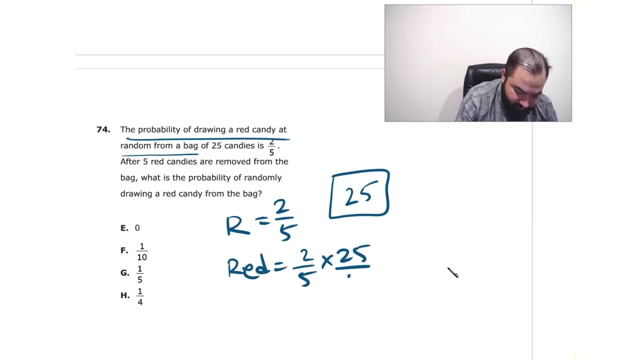 25 candies. so we have a bag with 25 candies. probability of drawing red is 2, 5th. remember the type two I showed here. so you just multiply the fraction with the number to how many, so how many red we have guys. 2, 5, 2, 5 times it by 25, remember? can we simplify the? 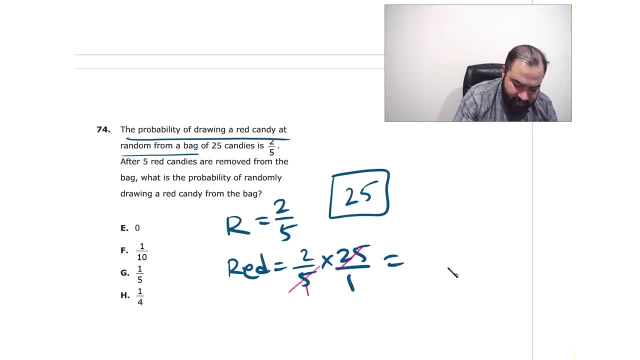 5 to 25, see simplification helps. so 1 and 5, so 2 times 5 is just worth 10. so we have 10 red. now, after 5, red candies are removed. okay, so remove 5 red. so I have only 5 red. remember when you. 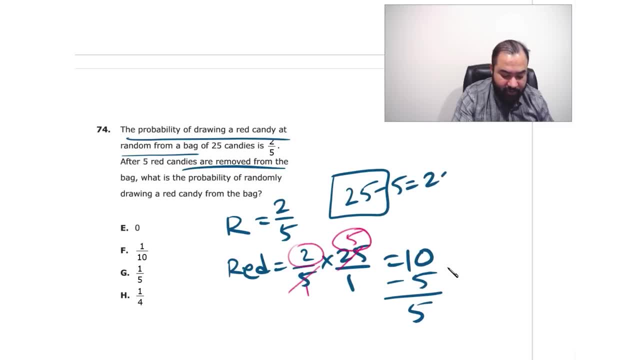 remove 5 red, the total is not 25 anymore. the total is now 20 because you remove the 5 red. so now what is the probability of drawing a red candy? so now I have 5 red, but total is 20, so it's 5 out of 20. I can simplify it by 5. we get 1 over 4 says 2 number. 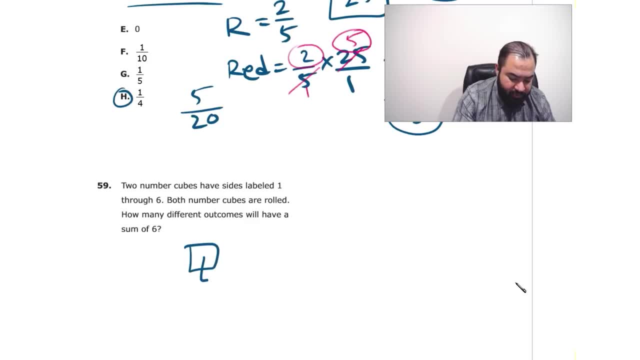 of cubes have sided labeled 1, so 2 cubes, right. they are each labeled with 1 through 6, like you know, like a die. now, both numbered cubes have sided labeled 1, so 2 cubes, right, they are each labeled with 1 through 6, like you know, like a die. now, both numbered. 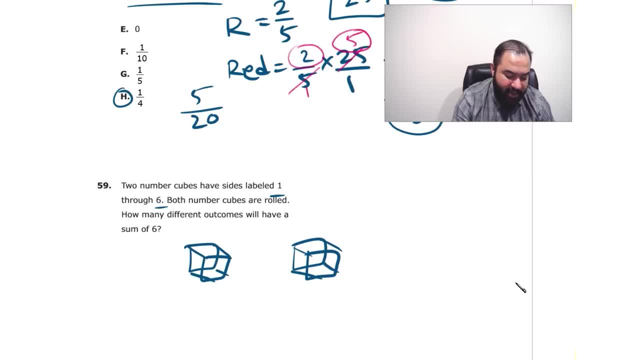 cubes are rolled, how many different outcomes will have a sum? 6. so you want to have an outcome six. in this kind of outcome situation, you can just list them. maybe from the first key we can get a one plus 5. the sum will be 6. that's one way, right, well, you could get like it. 2, and therefore still. 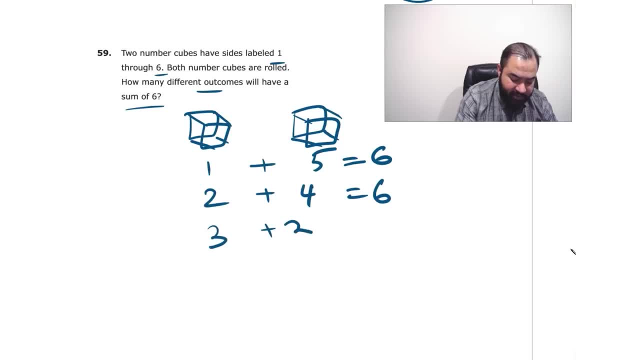 that's a 6. you could get 3 under 3, the 6 to get 4 first and then 2, that's a 6.. If you get 5 first and then 1,, that's also 6.. So that's it. These are the. 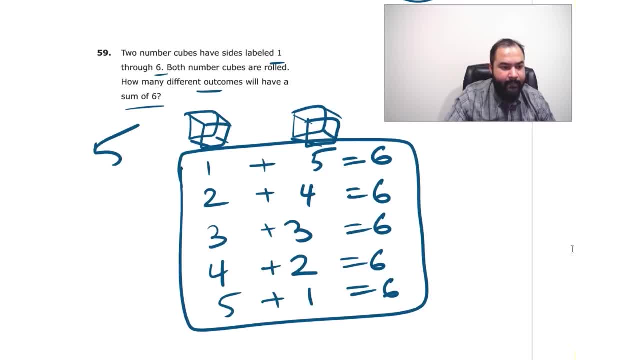 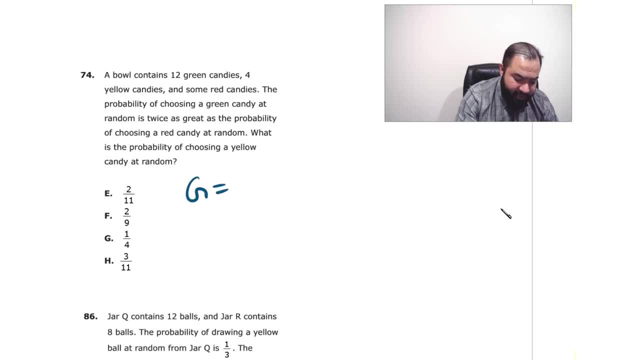 five different ways you can get it. So the answer is 5.. Now here it says, a bowl of candies. a bowl contains 12 green candies, 4 yellow and some red, but we don't know how many. Now the probability. 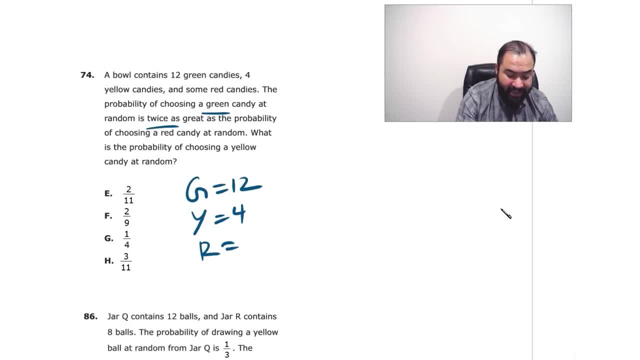 of choosing a green candy at random is twice the probability of choosing a red. So the probability of choosing green is 2 times the red. Well, green is 12,, so red is what 6, because 6 times 2 is. 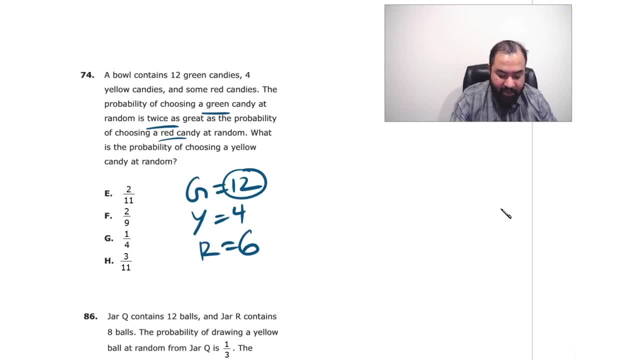 12. Green is 2 times greater than red, so red must have been 6.. Now what is the probability of choosing a yellow? So yellow is 4, so it's 4 out of what? Total, which is 12 plus 4, is 16. 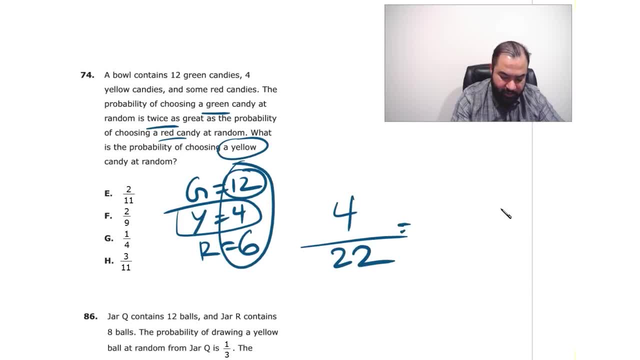 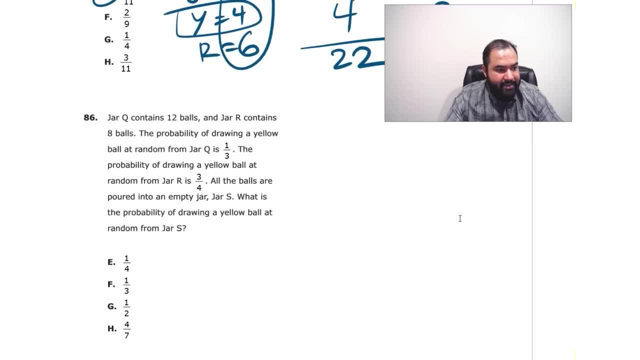 plus 6, 22.. You can simplify by 2, we get a 2 out of 11, so that's 2, 11.. All right now 86. here it says jar Q. so there's a ball. Q has 12 ball in it, total 12,. 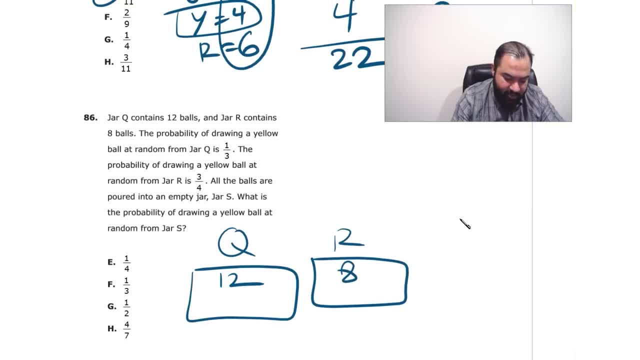 and jar R contains 8 ball, The probability of drawing a yellow ball at random from jar Q is one-third, So yellow is one-third, Remember. so one-third times 12, so that's 12 over 3,, that's 4, right? So I have 4 yellow. 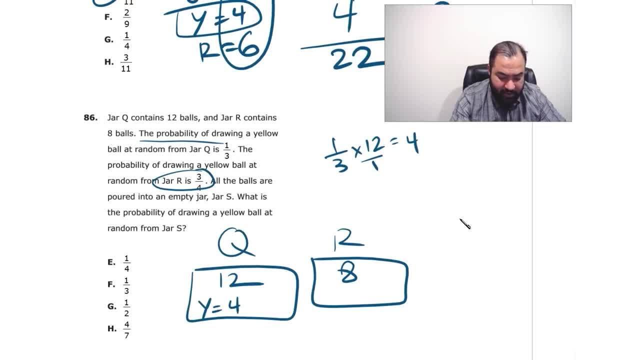 So the probability of drawing a yellow at jar R is 3-4.. So R has 8, so 3-4 times 8 over 1, you know, that's 24 divided by 4 is 6, so yellow is 6 here. You guys getting it what? 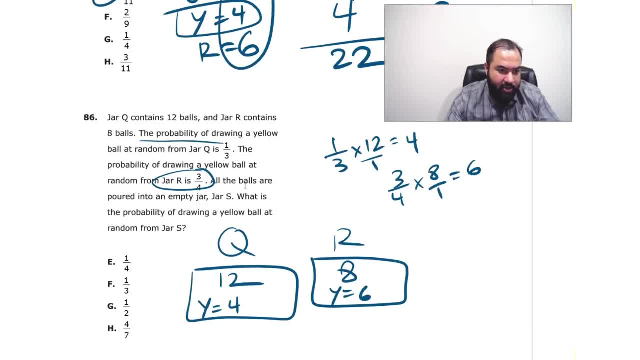 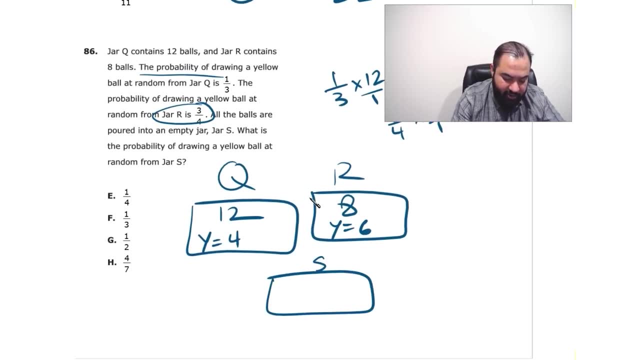 I did. I just multiplied the fraction with the number. that's it. Now all the balls are poured into an empty jar S. So now I got another jar S, we put all the ball there. so 12 and 8,, so total 20, and yellow is 4 plus 6, 10.. 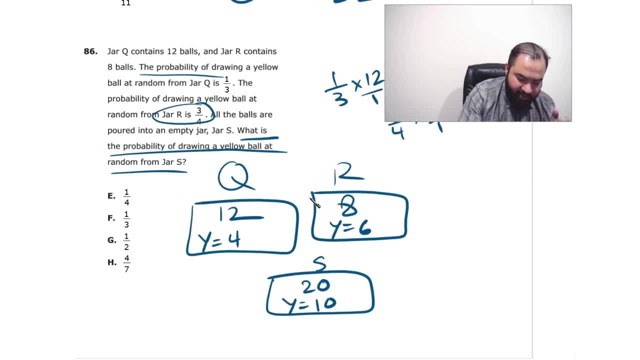 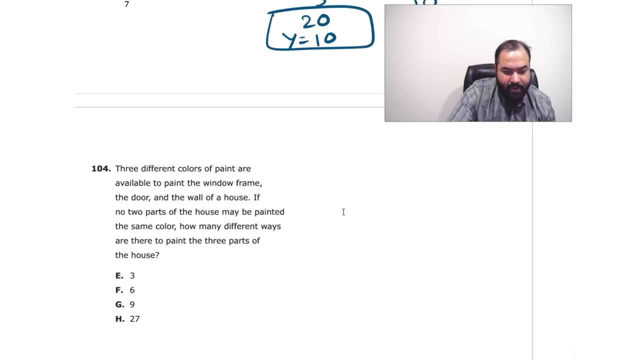 Now the question asking what is the probability of drawing yellow from the jar S? So it's 10 out of 20.. So that's one-half. It says three different colors of paint are available to paint the window frame, the door. 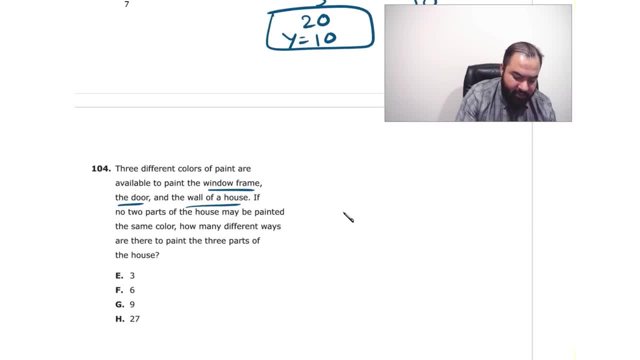 so we have a window frame, the door and the wall house. So you need window frame, door and the wall house. Two parts of the house may be painted the same color, So there are three different colors. So for window frame we have three options. right, You can pick anything out of the three. 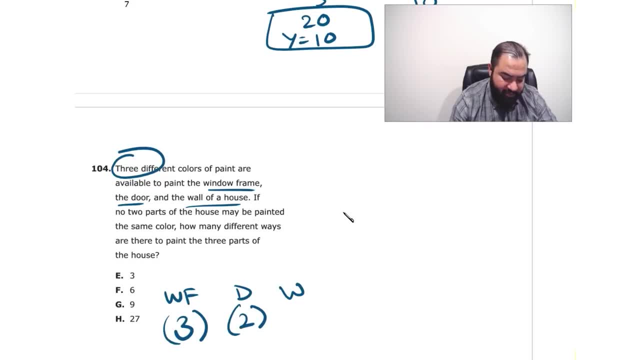 colors For the door. you have one less option. Remember: whatever paint you used for the window frame, you cannot use it for the door And for the wall. you have only one option, because whatever you used for window, frame and door, you cannot use it. 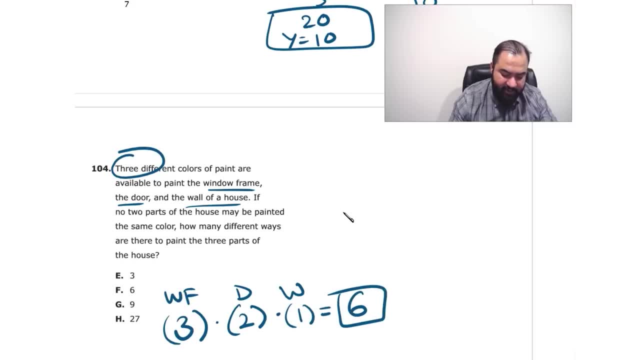 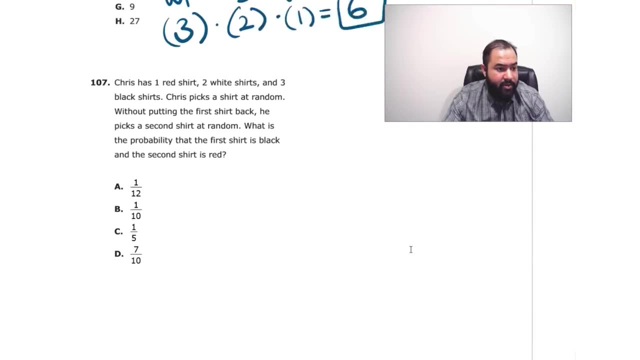 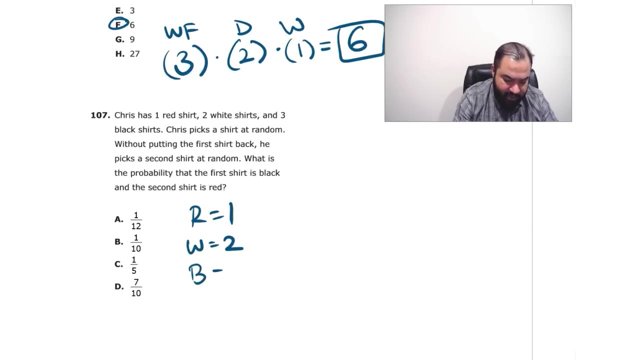 So you just multiply the options And then you get six. That's it. Clear 107 says: Chris has one red shirt, red shirt one, white two and black three. Now the Chris picks a shirt at random without putting the first shirt back. Remember the. 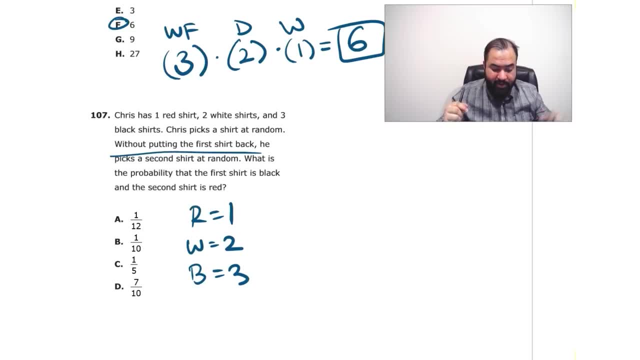 without replacement is. he picked a shirt at random and he didn't put it back, So in second he picked another shirt, right? What is the problem? The problem is probably that the first shirt he picked was black and then the second shirt. 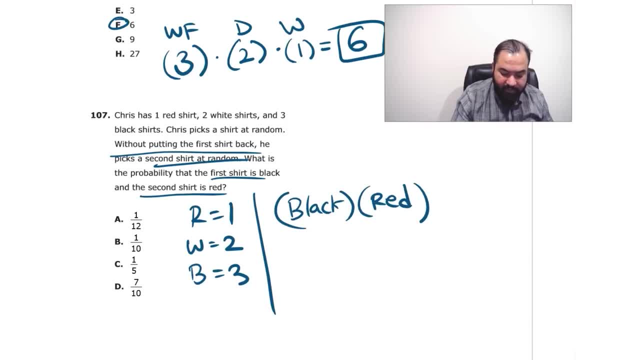 he picked was red. So the probability of him picking black shirt first is just simply three out of the total, which is three plus two five plus one six. But the probability of picking the red is red is one out of five, because one less. 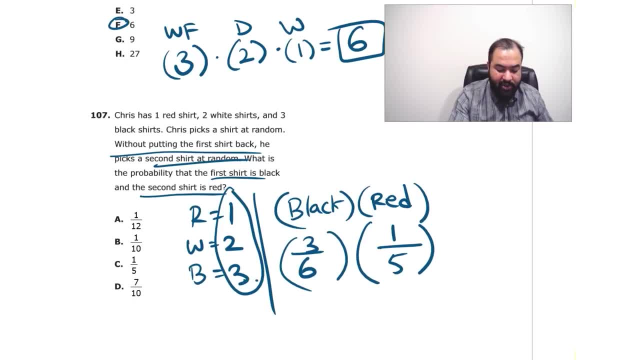 Because you already picked a black and you didn't put it back. So now you have total one less. So six over three means just one half times it by one fifth, So that's one tenth. That's it. That's the third type. 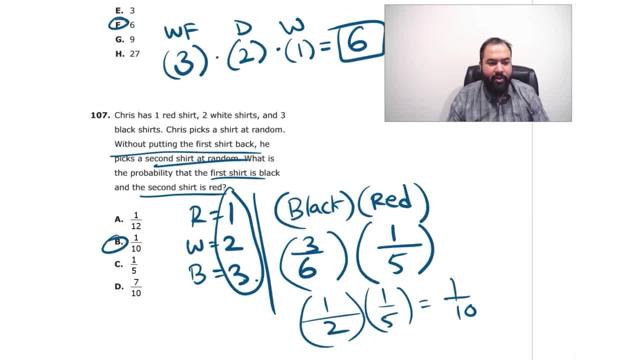 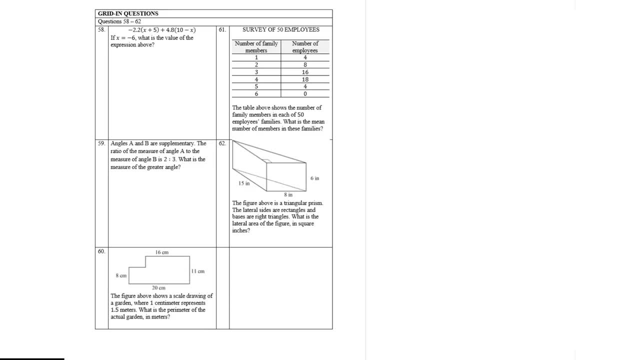 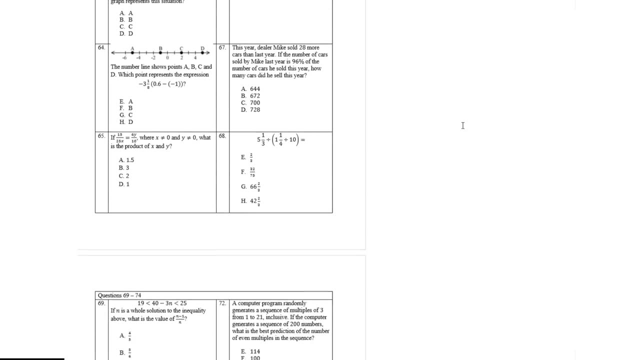 So I gave you guys the brief explanation. So if it were to be too fast, it's because I'm assuming that you guys know some basics. Okay, so these are some practice questions for you, So you can pause and practice them. This is page two.